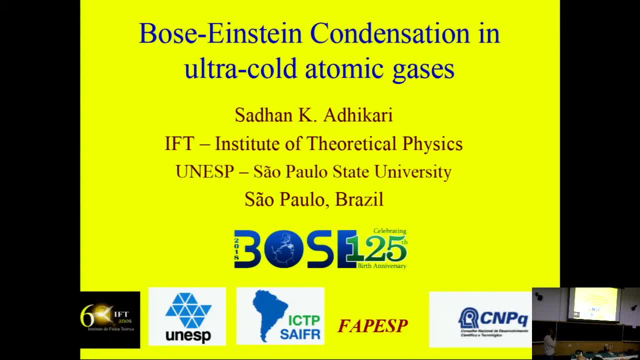 So today, Adhikari is going to tell us about Bose-Einstein condensation in ultra-cold atomic acids. So thank you very much for the introduction And thanks for the invitation to talk about Bose-Einstein condensation, And this year is the 125th anniversary. 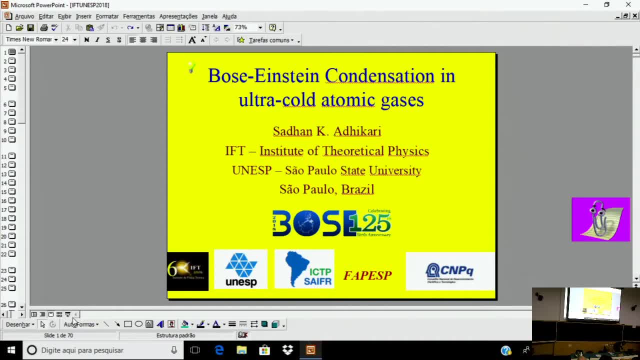 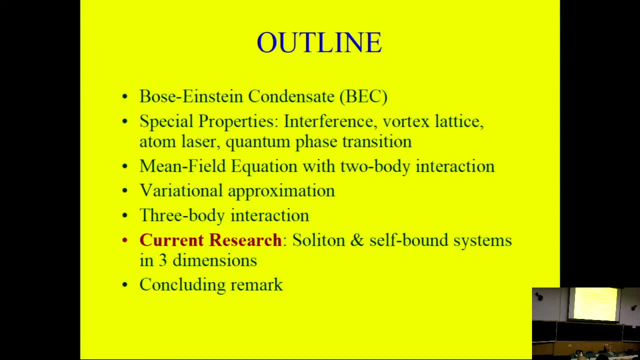 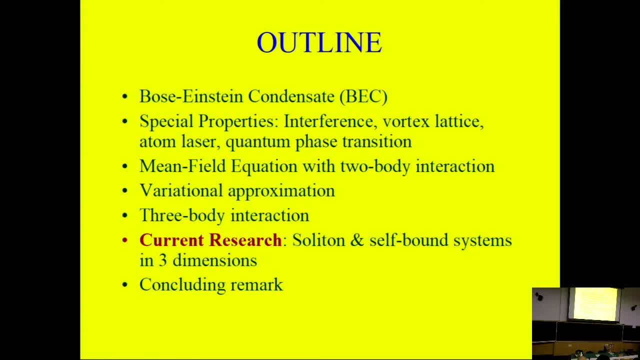 special properties of Bose-Einstein condensation. I will be talking about interference, vortex, lattice formation, atom, laser, quantum phase transition, and these are only few, because this is a quantum system. We have studied quantum mechanics in textbooks, which mostly talks about electrons, and this is quantum mechanics in a different type of matter. so 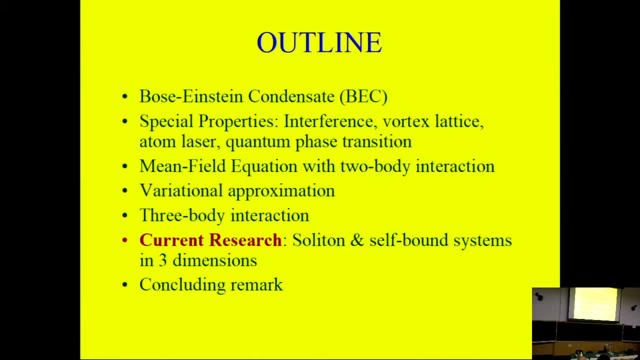 we will slowly introduce everything, and there are some theoretical treatments using various ways: Mean field equation, variation approximation, three body interaction and in the end, I will talk little bit about our current research on soliton and cell bound systems in three dimensions and then concluding 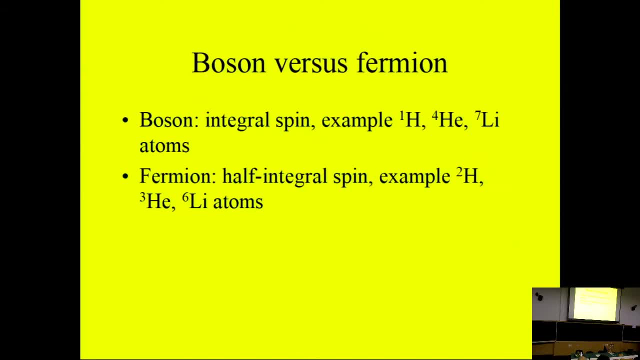 remarks. and boson versus fermions. So we will be talking about atomic gases. So you have fermions and bosons. Bosons have integral spin and examples are one: hydrogen helium 4, lithium 7. and fermions have half integral spins and the examples are two: hydrogen three. 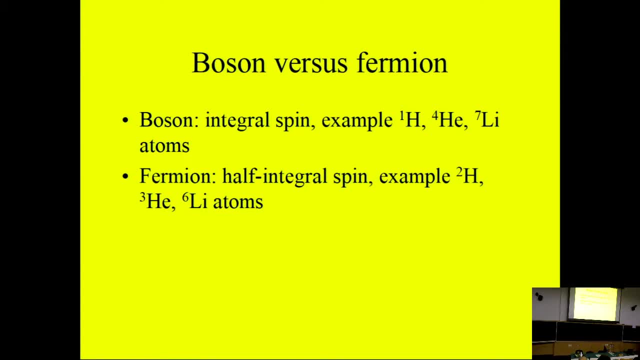 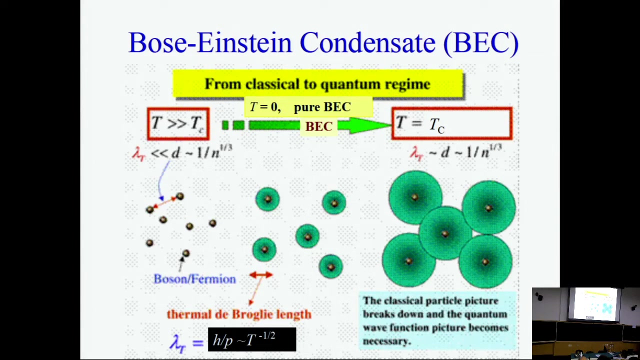 helium and six lithium atoms. So the integral spins have an even number of half integral particles, spin particles like electron, proton and neutron and here, and even integral and integral. Okay, and half integral spins, And what is Bose-Einstein condensation? So this is, you have the atomic 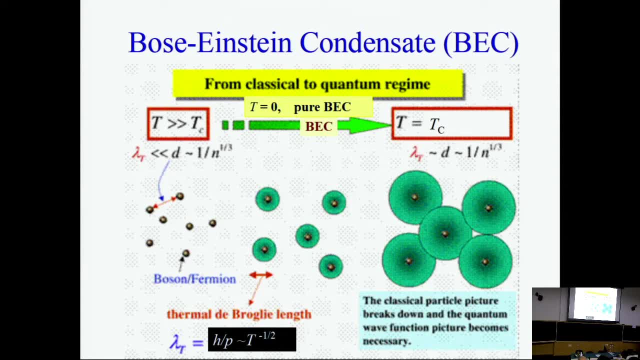 particles. We are talking about atomic gas. So you have the particles here at high temperature, large temperature, room temperature. As the temperature is reduced, size of the particles increase. So it really increases. This is the de Broglie wavelength that becomes the 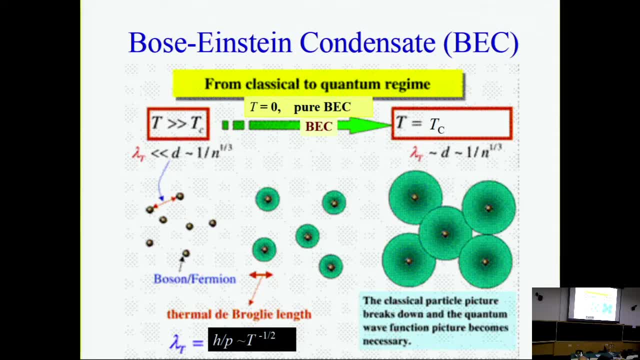 size of the particles. So if you have a hole of small size, at high temperature the atoms can pass through it. At low temperature it cannot pass through it, And at very low temperature this becomes even larger and there is big overlap between the atoms And this size is. 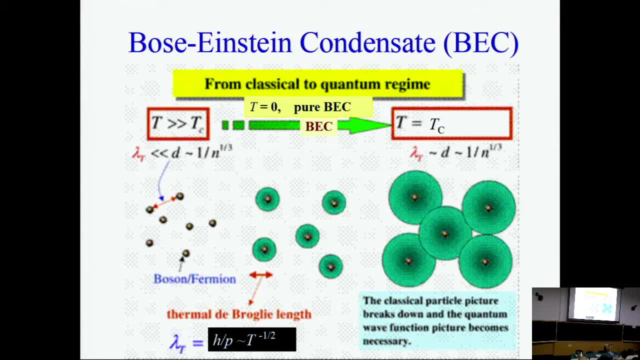 roughly given by the thermal de Broglie. wavelength h by p is t to the power, half t is the temperature And this was predicted. when there is overlap, there is a critical temperature when this overlap happens and you have the Bose-Einstein. 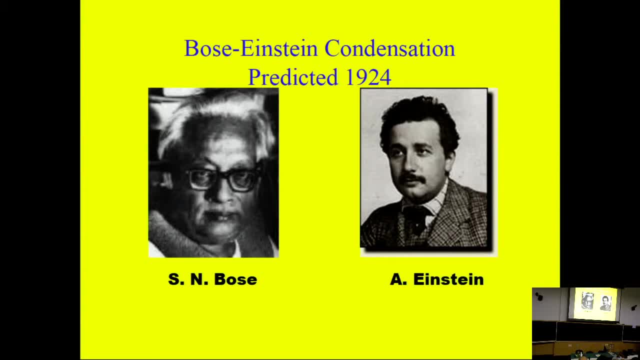 condensation, And this was predicted in 1924.. It has some history. Bose was trying to explain the distribution of photons in a black body, in black body radiation, with respect to energy. He tried to find the quantitative formula of this distribution of photons And he was. 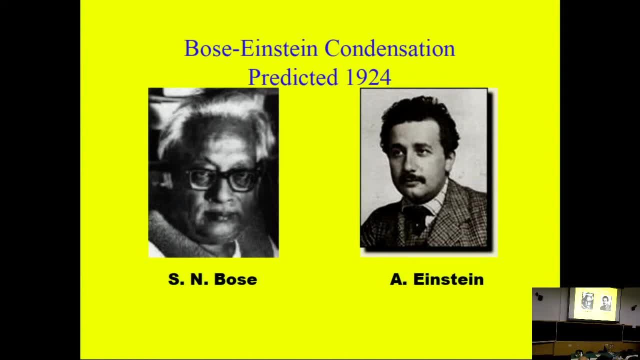 trying to fit so that it gives the Planck's radiation formula And since he had, he put some parameters- I will show the distribution function later- And that fitted the distribution and gave the Planck radiation formula And he tried to publish it And he was unable And 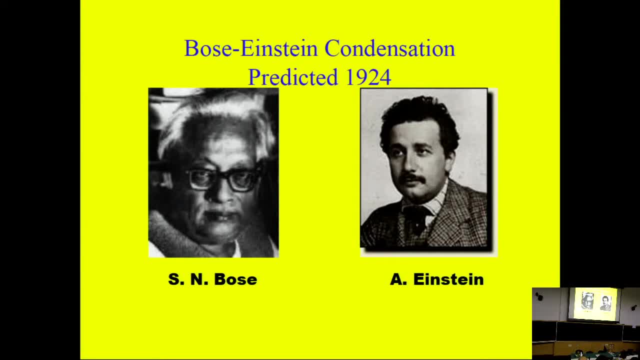 he asked help from Einstein. And Einstein understood the work and he published it in Zeitgeist Physics. And he went a little farther. He thought that if the atoms obey these statistics, or particles in place of photons obey these statistics, what happens? And he realized: 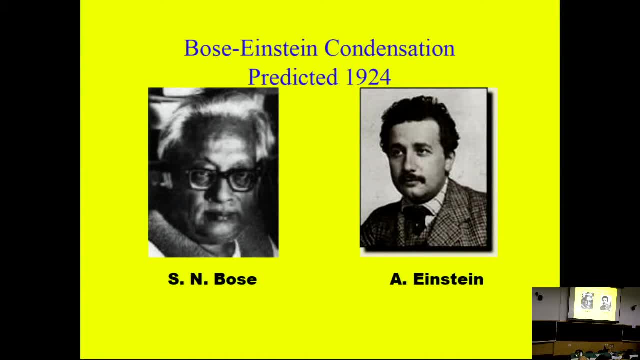 that something interesting happens because at a high temperature most of the particles can come to the ground straight with this distribution. But he didn't Einstein, I think at that time he did not have much idea about bosons and fermions And these statistics. 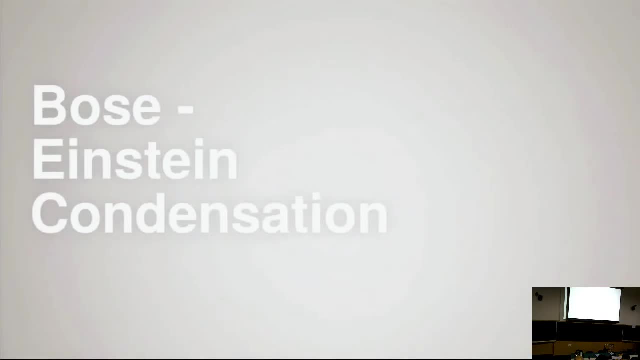 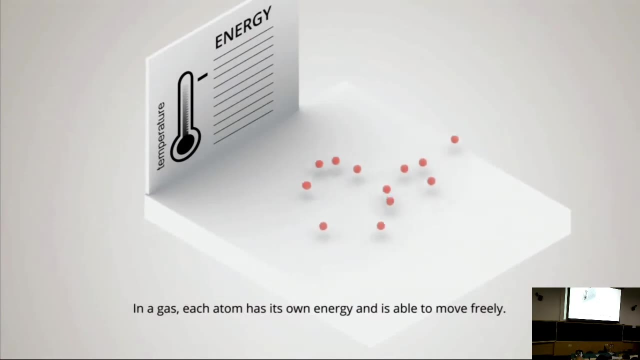 here what happened, Okay, So here this is a small view of what is happening. So they have. you have the atoms which are moving freely there And the temperature is decreasing And the atoms become larger and larger and move slower and slower. Eventually all the atoms come to the ground. state Drive: 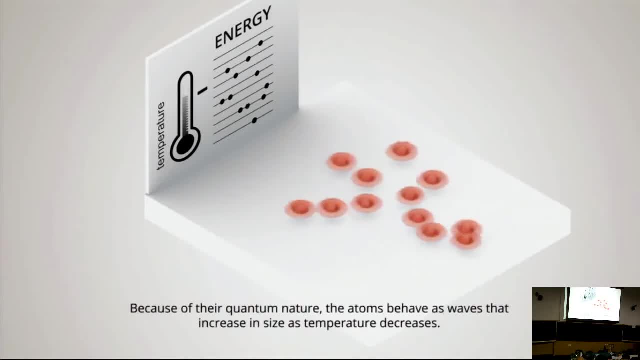 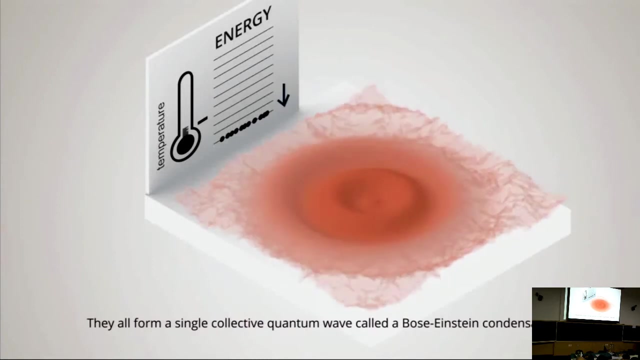 f on the disk for few second And there is a overlap And zero state in the point And this became a constant curvature and the giant molecule is formed. This is the Bose-Einstein condensate. The atoms lose their identity and we have this condensate. 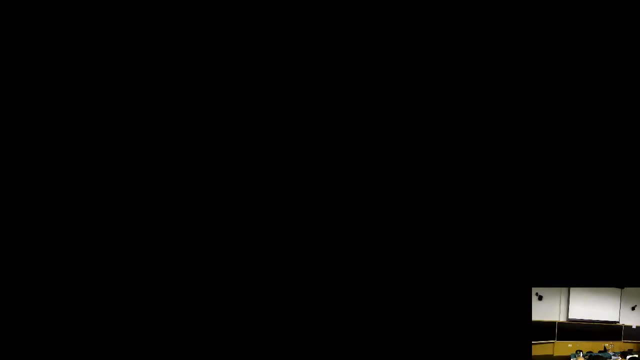 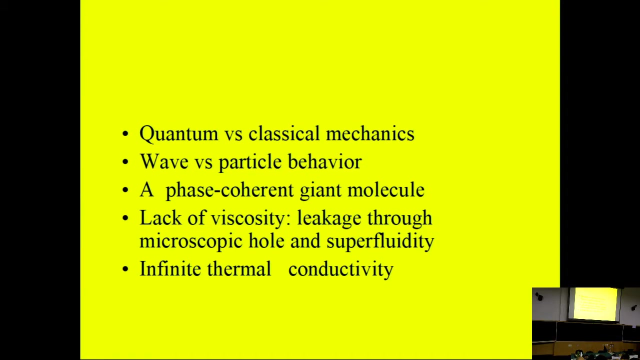 So there were two papers, one by Bose and one by Einstein. Yes, yes, But then Einstein didn't talk about condensation. Einstein talked about condensation and Bose talked about the distribution. So we have the quantum versus classical mechanics- Bose did not talk about condensation- and wave and 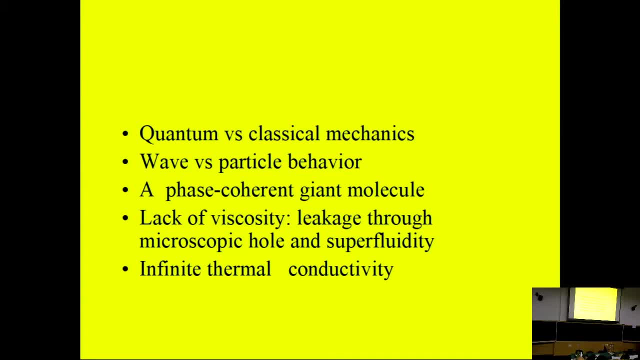 particle behavior and we have a phase, coherent giant molecule and there is lack of viscosity and leakage through microscopic hole and super fluidity. These are the special properties. and another thing is infinite thermal conductivity. If this has charge, it will be super conductor, as it does. did not have charge, It becomes. 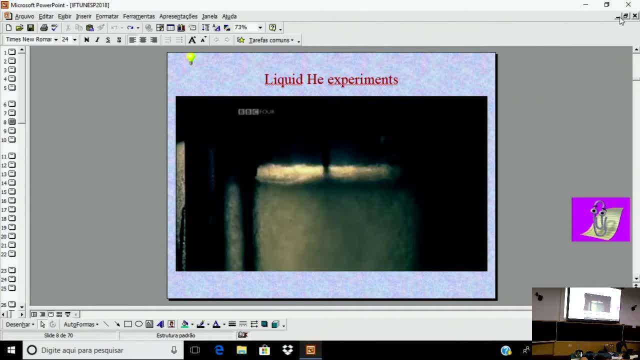 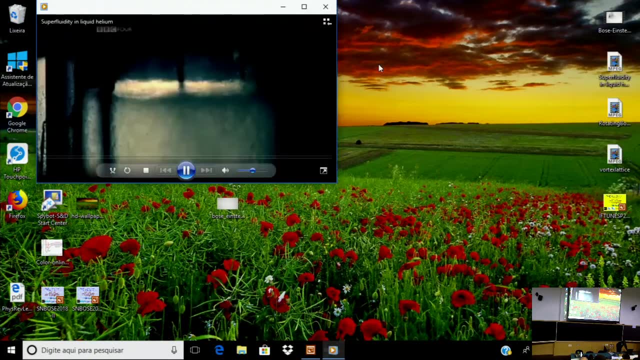 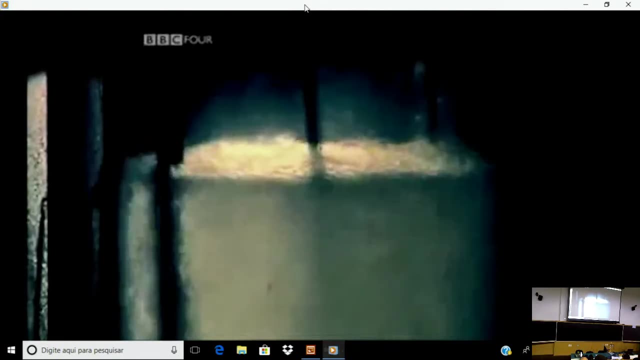 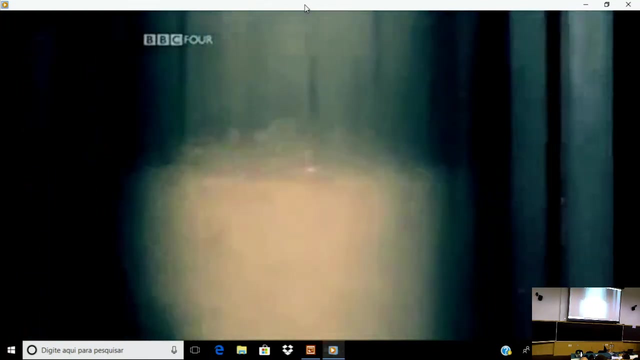 a thermal conductor, So we show another video. This is this video. You will see it's liquid helium 4 which is boiling at 4 degree Kelvin, and when it's boiling it takes latent heat and it tries to become cooler and cooler, and when it reaches 2 degree, 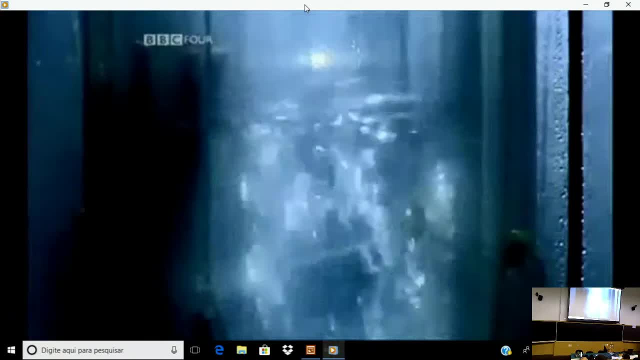 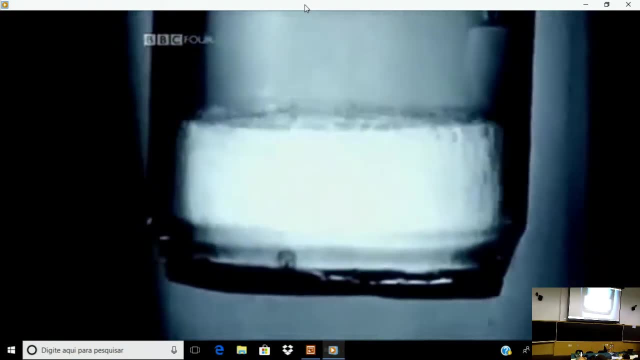 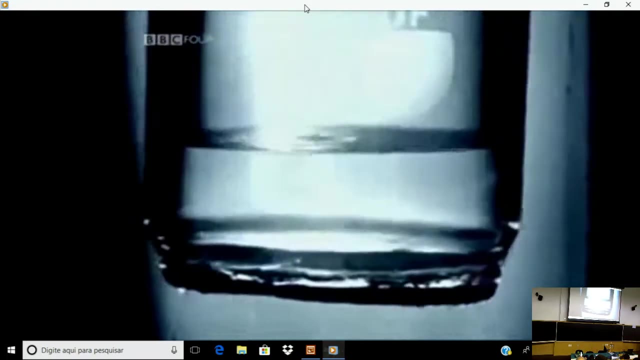 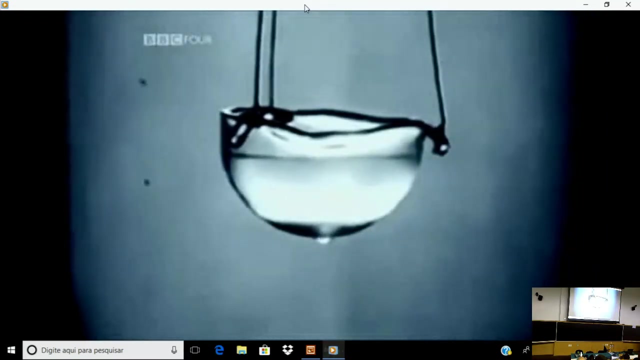 Kelvin, and that is the Bose-Einstein condensation temperature. at this, in this case, boiling stops because the thermal conductivity is infinite, So there is no need for convection to reach an equilibrium temperature. and then you have leakage through this thing, the microscopic holes, and you can go super flow. that means it can go over also like this: the super fluidity. 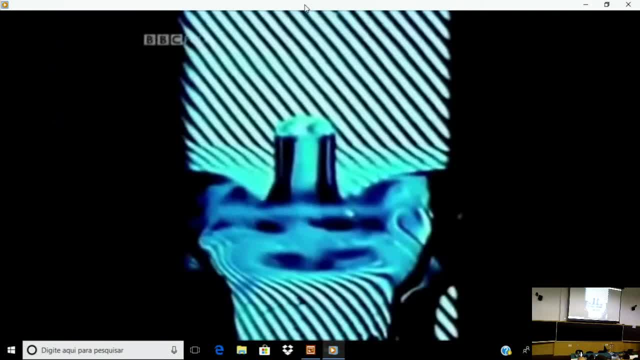 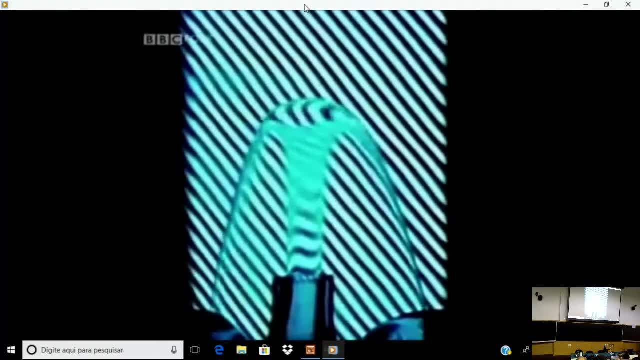 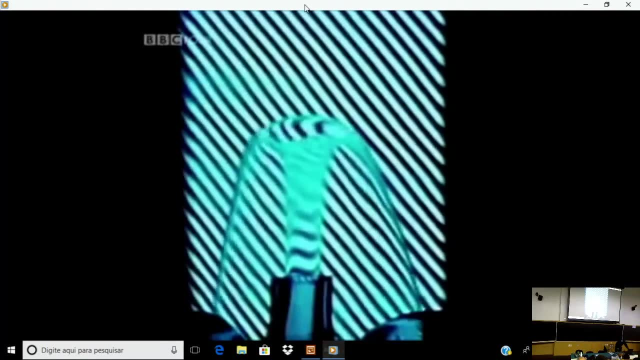 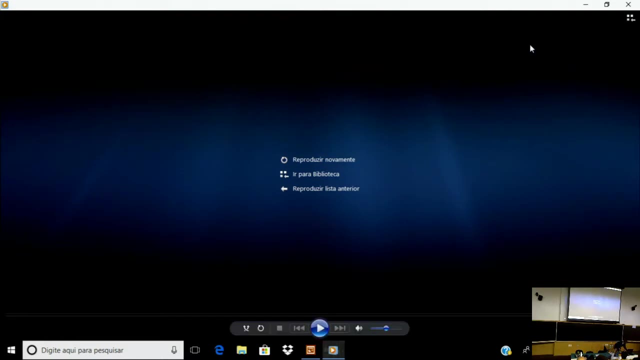 and then if you have a fountain, if you make a fountain, this fountain will never stop. without any pump, like in superconductor, The current goes, It goes round and round and never stops. for years There is no friction. Sorry the fact that there is no friction, I mean they still feel the force of gravity. 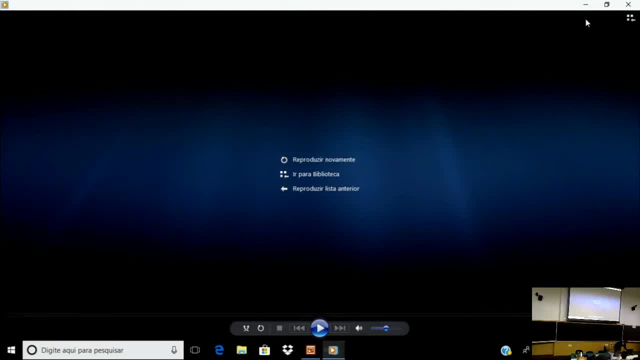 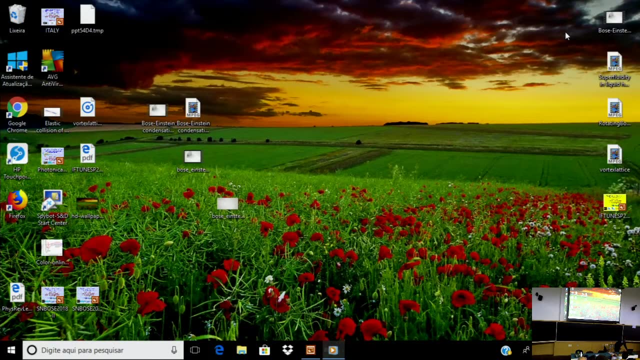 It still feels the force of gravity. Yes, so once it is there, the pump was there. like the current also goes around. but if you have a big force downward then it may not work. But once the force was given then it will work. The force was given once to make the 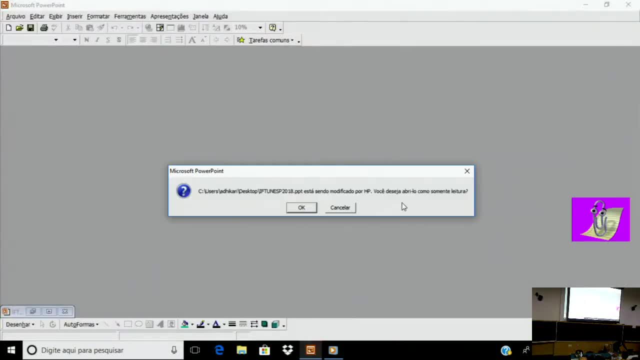 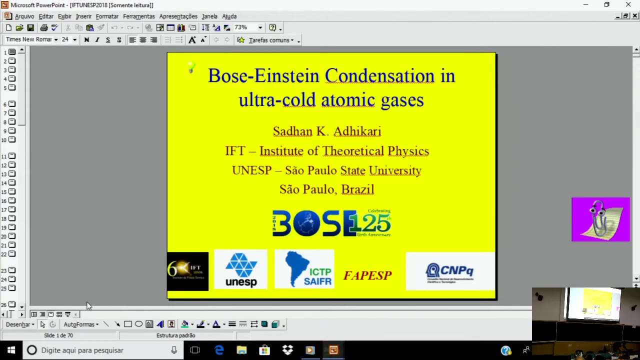 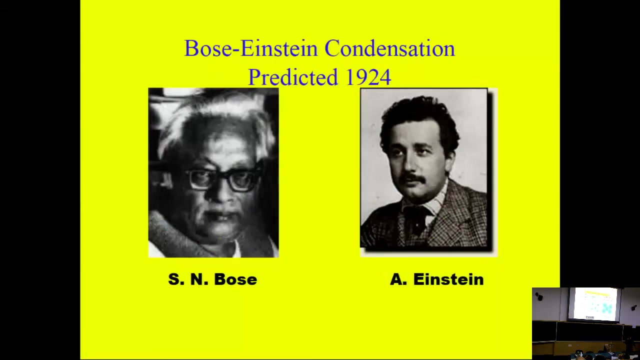 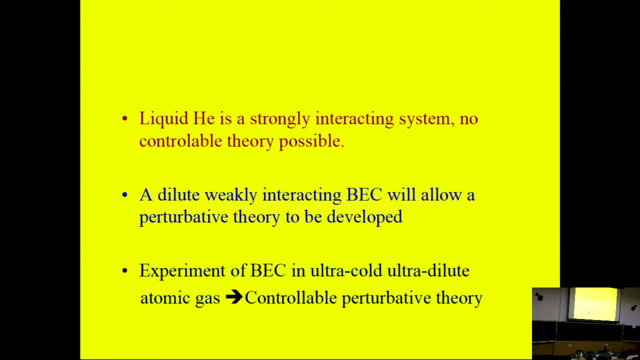 fountain. Something is wrong. This is okay, Okay, Okay, Okay. Actually, this video refused to play inside the. so liquid helium is strongly interacting system, So you cannot make a controllable theory. A dilute, weakly interacting base will allow a perturbative theory to be developed and we can study it in a different way. 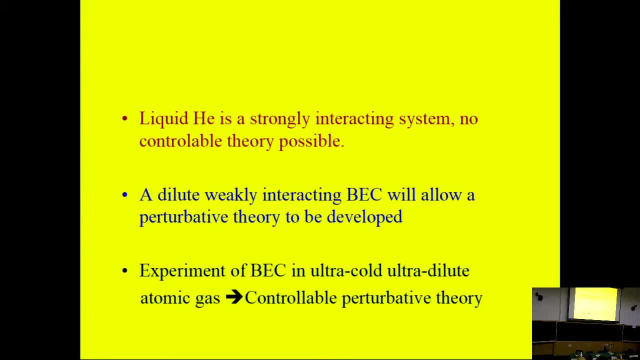 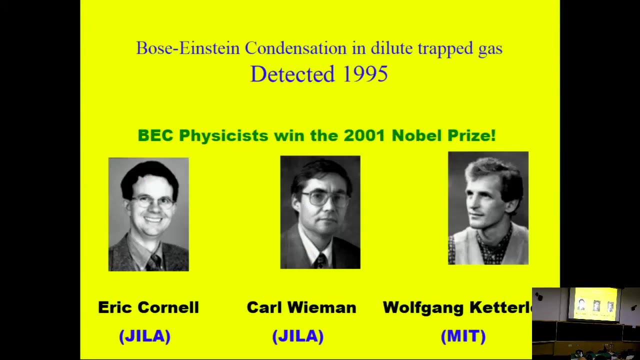 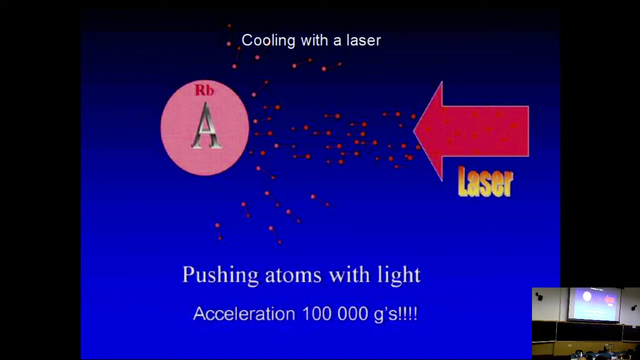 decent way. So experiment of BEC in ultra-cold, ultra-dilute atomic gas will give that controllable perturbative theory this weak coupling theory. So this was done by these people in 1995, and they got Nobel Prize for this in 2001.. So you cool these atoms using a laser. This 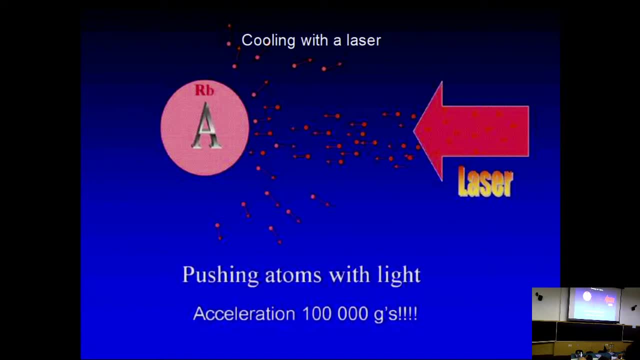 technique was known before. So you have the rubidium atoms, which has magnetic moment. All these atoms have magnetic moment. So rubidium atom has one unit of magnetic moment. Laser falls on that which has energy equal to the most probable excitation energy of. 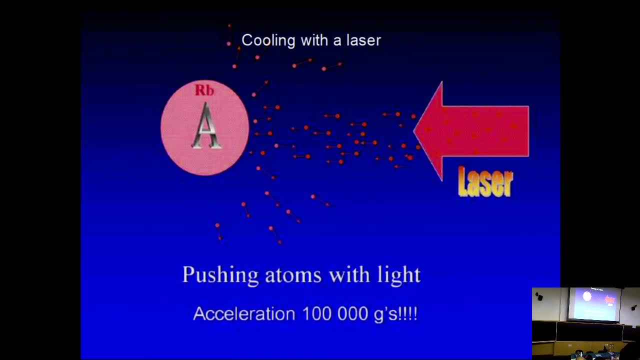 the rubidium atom, Like in hydrogen atom. it is the. it is the 1s to 2p excitation. That is the most probable excitation, And here is some ns, always ns n plus 1p. That is the most probable excitation energy this laser has. So it excites the. 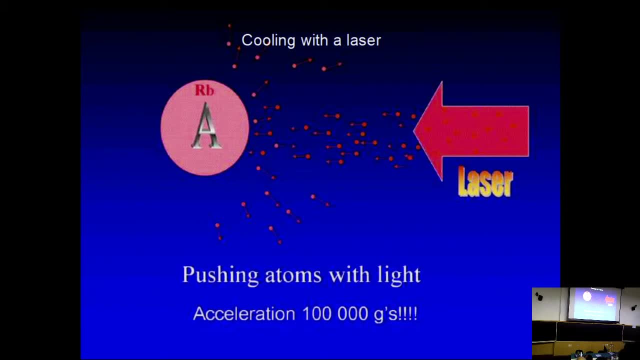 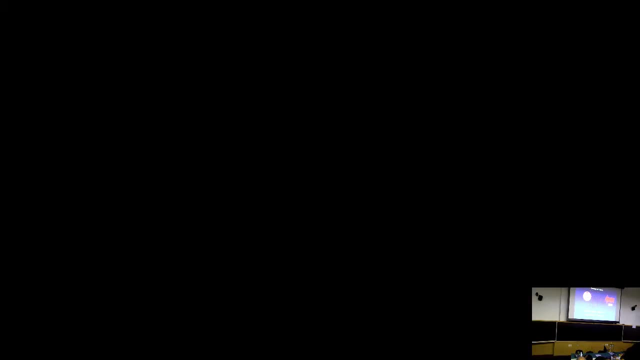 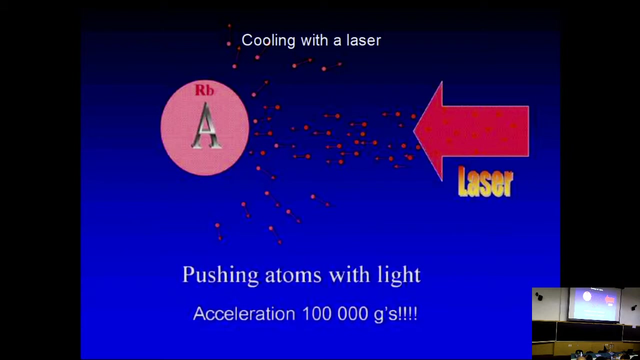 atom. Once it excites the atom it goes to the excited state but it gets the kick from the photon So it momentum is reduced, It moves slowly but goes forward. Then it emits the electron photon back and electron comes to the ground state And one once that happens. 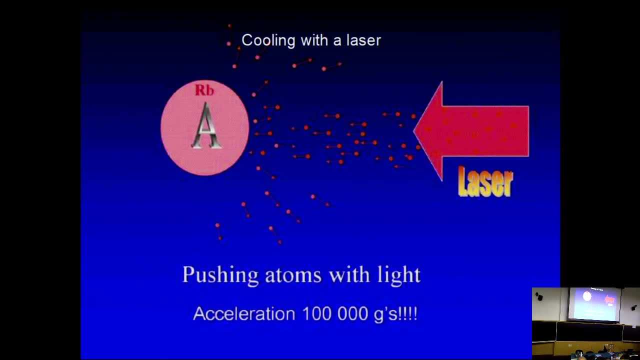 it has less energy and it is prepared to accept another photon, so that it is again excited and comes back to the ground state. And each time it gets a photon from the laser it it slows down And in a, in a matter of one meter it can cool down and then it will. 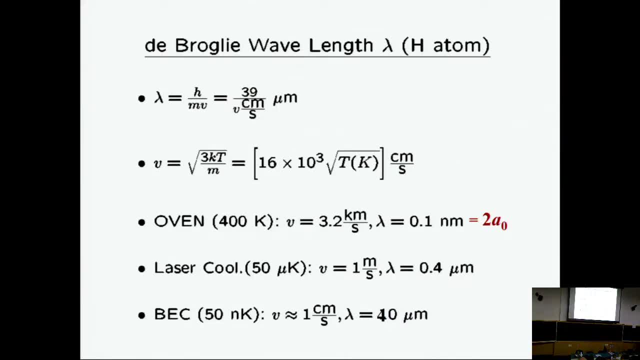 phase back again And it it will phase back once again. That is called the quantmale velocity. here It is like getting to the explosion from from a large velocity of something like- see here- kilometers per second to micrometer per second. So this is a de Broglie wavelength. 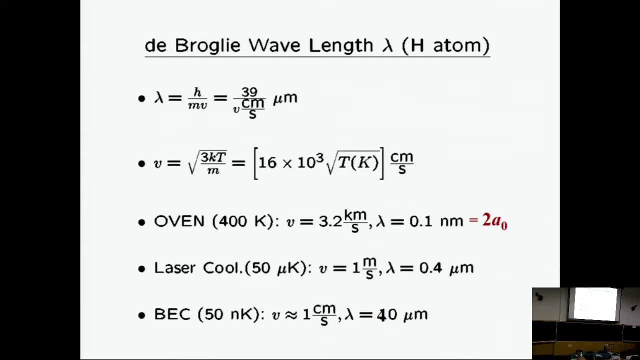 lambda temperature is 400 degree Kelvin, So velocity is 3 kilometers per second and the size is 2 times A naught of the hydrogen atom. 2 times A naught A naught is the Bohr radius. This is roughly twice the size of the hydrogen atom. And then it cools down. It can cool. 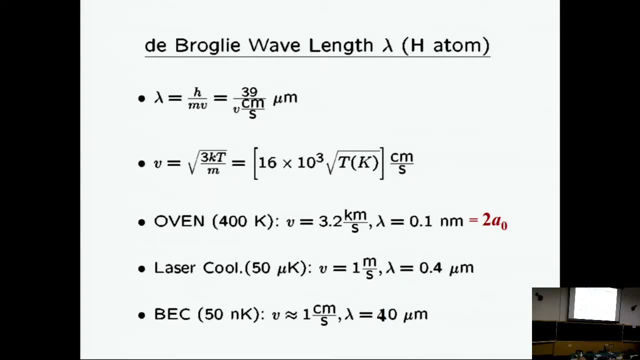 down to 0.4 micrometer at 50 micro Kelvin. This is the capacity of the laser. It can cool down to that. And then for BEC we need something more. The velocity has to be of the order of 1 centimeter per second and wavelength of 40 micrometers. 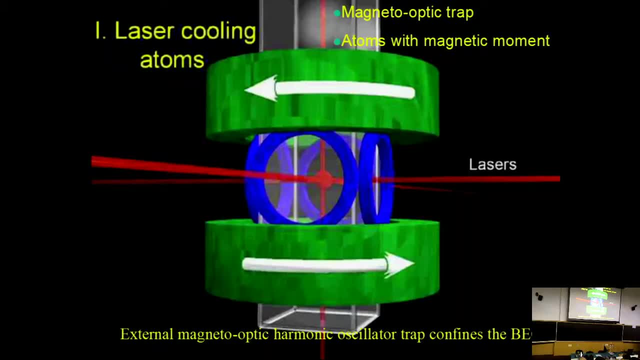 So then, this is some setup, how it is trapped. It has 3 electromagnets- This blue one and the green one- And the atoms come from the top and stays at the middle, And if it tries to come out, then you have these lasers, which pushes it back with appropriate energy And atoms have. 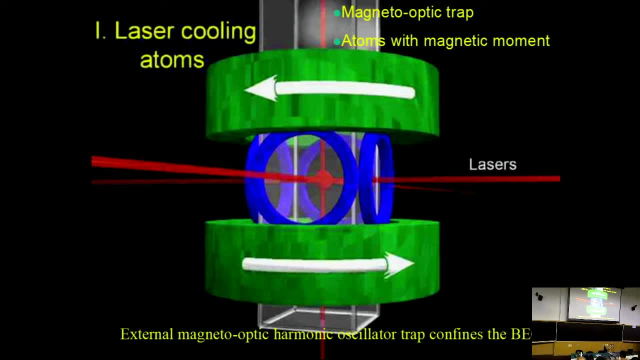 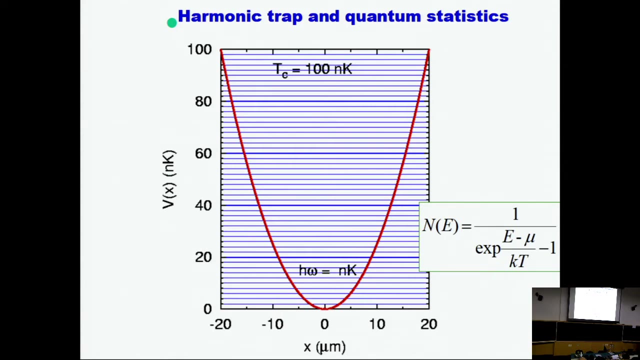 magnetic movement. So this trap is roughly harmonic oscillator type trap. And you have this external magneto-optic harmonic oscillator trap which confines the BEC, And this is a distribution. This distribution function was first found empirically and then it is interpreted correctly. 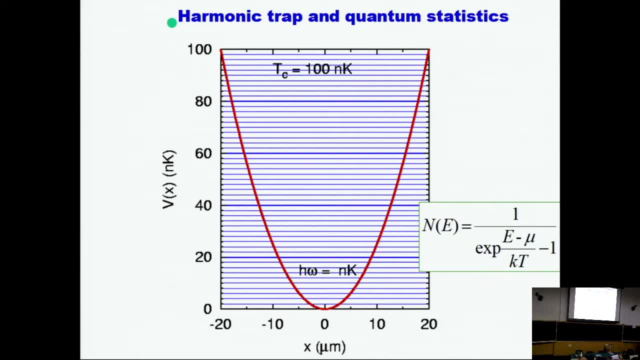 This is the function. The interesting feature of this function is that when the energy is roughly 100 nano Kelvin, this is the trap energy of the order of nano Kelvin. Most of the atoms classically should be here, But in BEC it comes down here at that temperature. 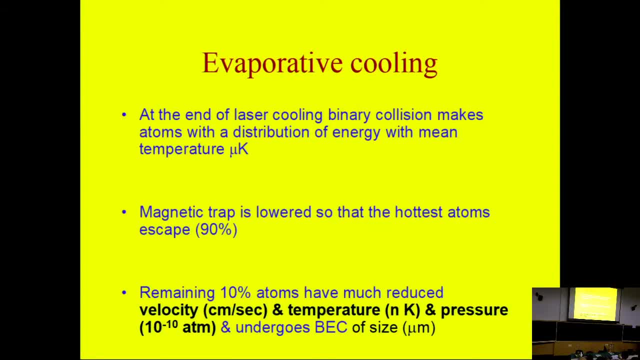 So then you have condensation, So then it is not enough, So you have to cool further To have BEC, because the velocity has to be 1 centimeter per second for it to condense and the size has to be at least 40. 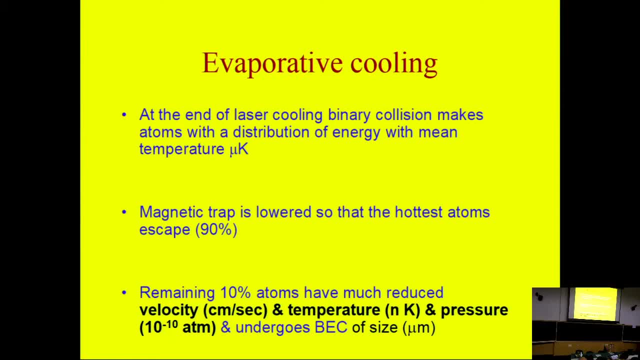 50 micrometer to have a big overlap. So then you have this distribution of energy At the end of the laser we have there in the trap. It is a distribution of energy because of collision and then you reduce the magnetic trap that the hottest atom escapes. So magnetic trap is reduced. 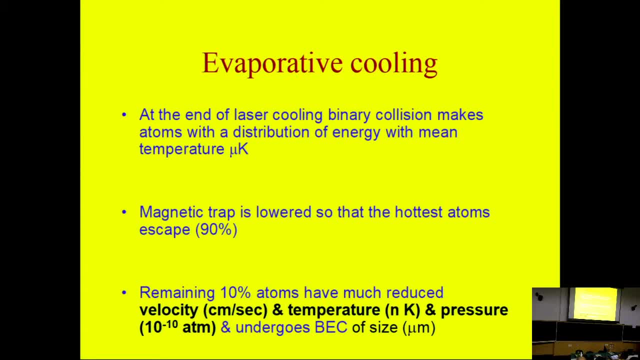 in size so the hottest atoms escape, and so you have 90% of the atoms which escape and you have only 10% which cools down and forms the BEC. So remaining 10% atoms have much reduced velocity of the error of centimeters per second and temperature of 10 nano Kelvin and pressure of 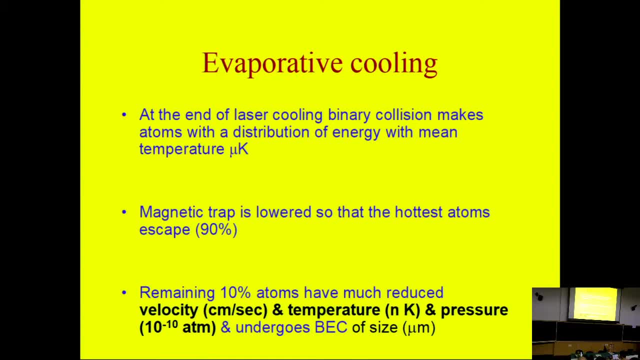 10 to the power minus 10 atmosphere, and that was BEC of size micrometer. This pressure could be larger but the we made this pressure so low so you can have a perturbative theory, weak interaction. So the atoms are very far away, See normal case. the atoms are about angstrom away few. 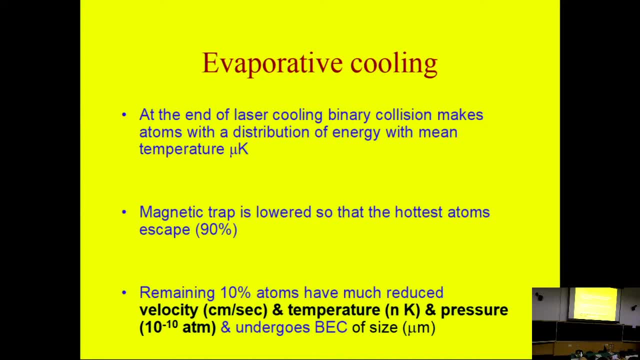 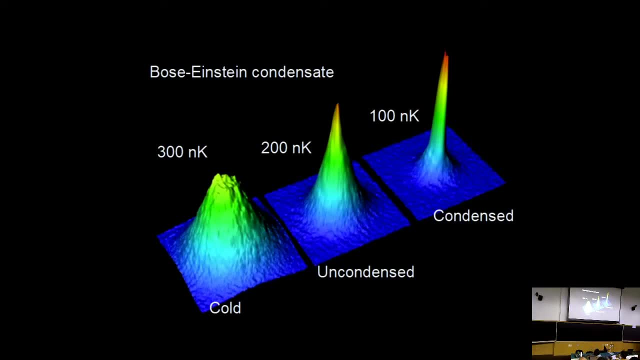 angstroms, And here it will be thousands of angstroms away. This is the artist picture of the Bose-Einstein condensation. As temperature is down, the higher peak means that you have most of the atoms at 0 velocity and distribution of velocity. 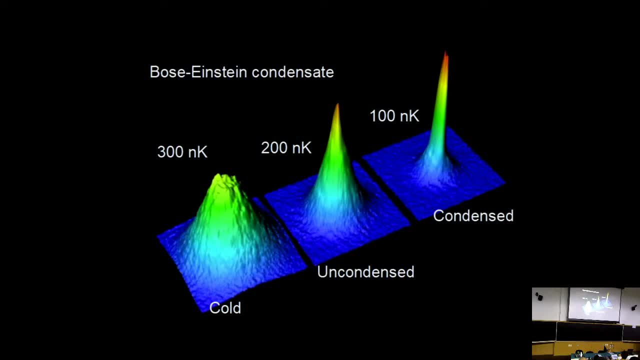 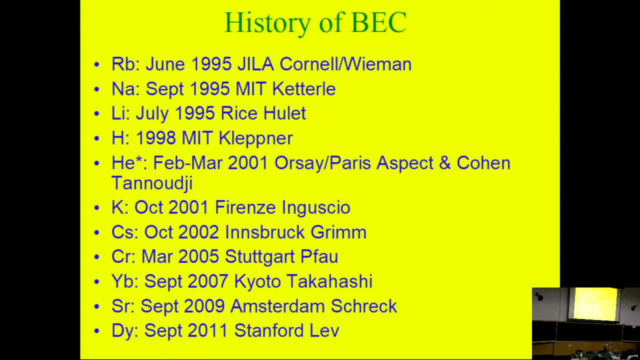 is very small And here you have lot of atoms with higher velocity. in this case it means By now there are many atoms which has been condensed: Rubirium, sodium, lithium, hydrogen, helium, potassium, cesium. the big list I stopped at 19- 2011. that could be more atoms. 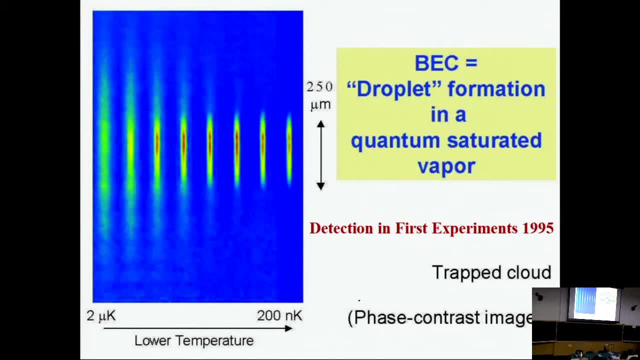 Then how to detect that you have formed. it has formed a condensate. The detection is interesting. This is a squash shaped trap. It's hard to detect in this case. So you see the big list. I stopped at 19, 2011. that could be more atoms. Then how to detect that you had formed. it has formed a condensate. The detection is interesting. This is a c? gerset trap. It's a hard time to do. In fact, we do have the C-Gercept trap. It's a hard time to do And you'll notice. this is exactly what we call for. 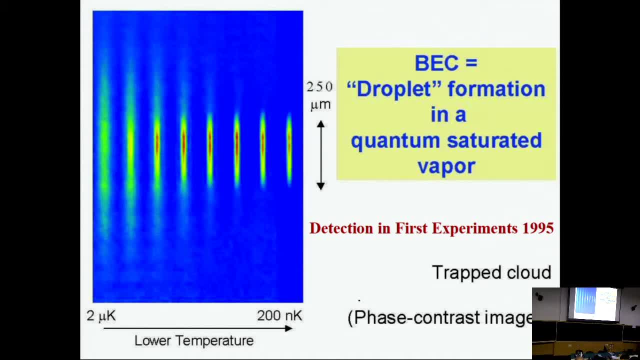 This is a called the SIGAR and this is a much easier And you will notice that there's many things trap. It is a harmonic oscillator trap which is stronger in one direction compared to others, so that the condensate has form of a pencil or cigar. 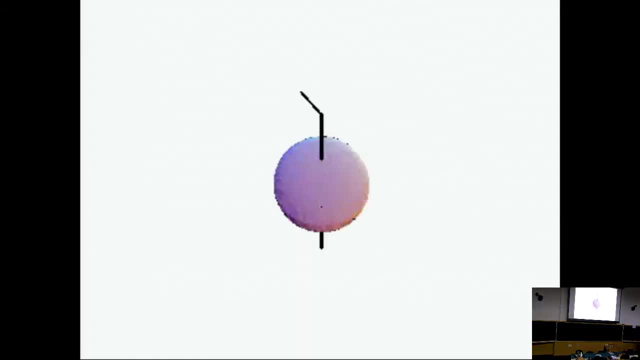 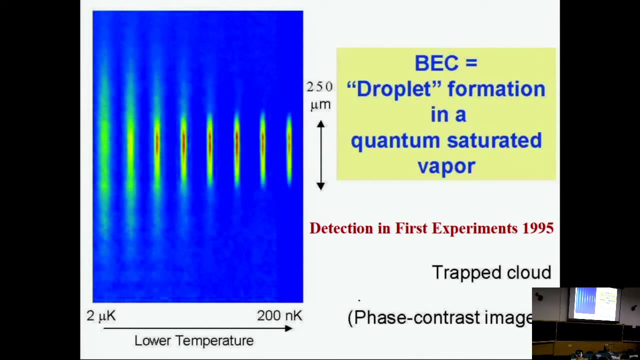 So when the temperature's higher- micro-Kelvin- you see there's a cloud, gaseous cloud, and you cannot control it very easily. but now it is condensed, temperature is lower. and when it is condensed it takes the shape of the vessel, it takes the shape of the 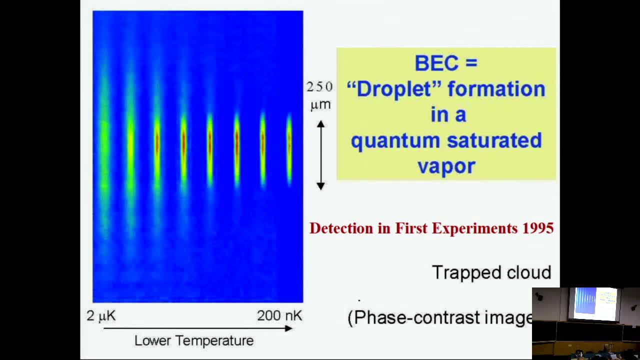 trap. You can turn the trap a little bit. The shape will be immediately changed, which will not be case when it is not condensed Like liquid takes the shape of the vessel. The vessel is round, liquid is round, So this is how it was detected in the beginning, But now there are many other. 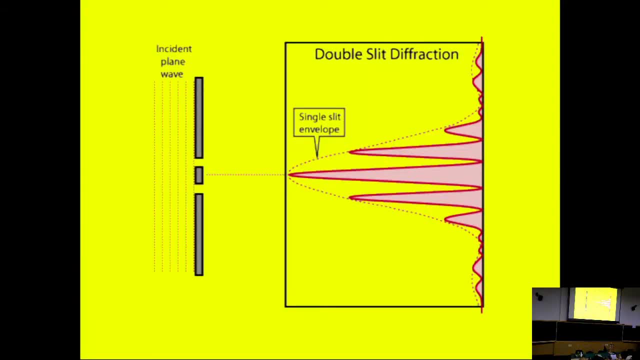 ways to detect it. I'll talk about another way to detect. So this is a interference interference, double slit, interference in optics. So light enters coherent light enters through the two slits. It forms an interference pattern: Bright, dark, bright, dark. So but 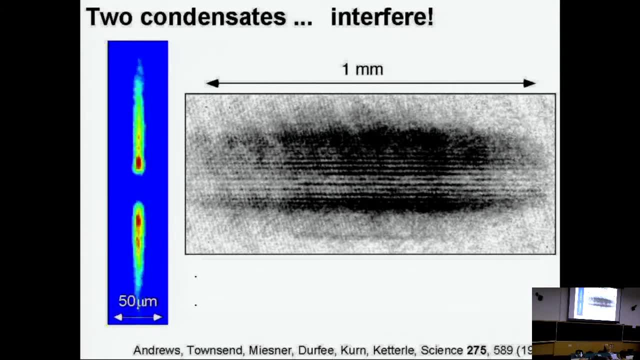 the total energy of light is conserved. So same thing happens here. This is a coherent straight. In the other light experiment you need a coherent light beam, Here you need a coherent matter wave. So once it is formed in a trap and cools down, comes to the ground state, it's a coherent. 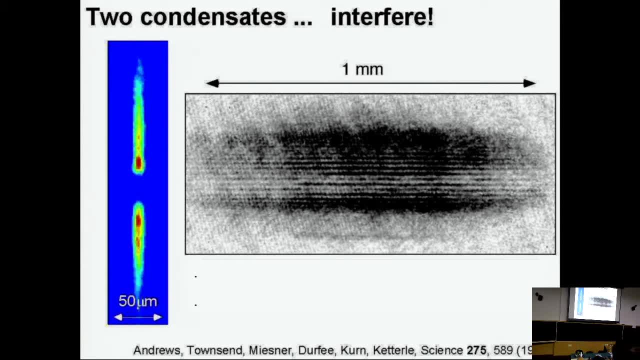 state. Now, this is the. this is in the form of a pencil. You burn the middle by a laser, destroy the middle. The two parts still remain coherent. Now we allow them to expand, Much, much expand for many seconds. So you see, the size is here 50 micrometer and here it's 1. 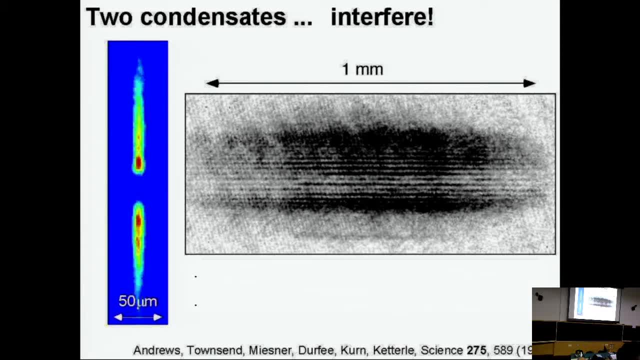 millimeter, So it is. So it is in the shape of pencil, but because of internal force it changes shape and becomes the. takes the shape of this disk, Spheroid, And you see that the interference fringes. you can see the interference pattern here, Interference pattern here, black and white. 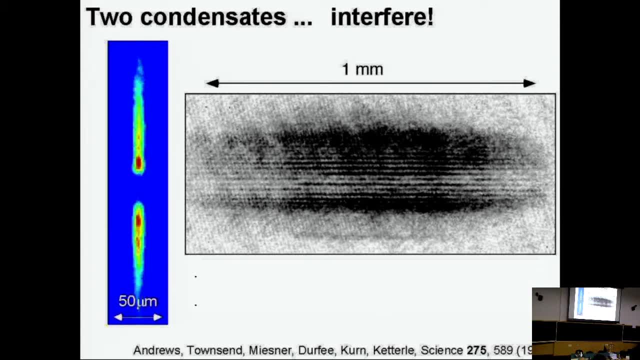 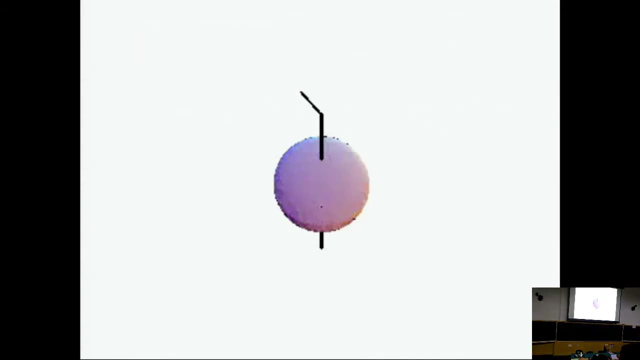 black and white, But the total number of atoms is conserved. So in one place you have double the number of atoms, In other place you have vacuum. So this interference of matter when it expands. Now there's another way. So if you rotate it, the interesting thing happens there in. 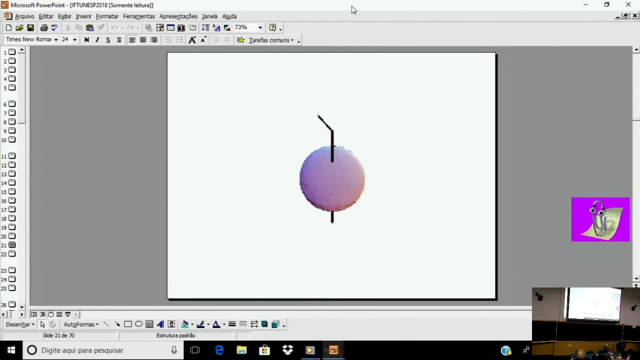 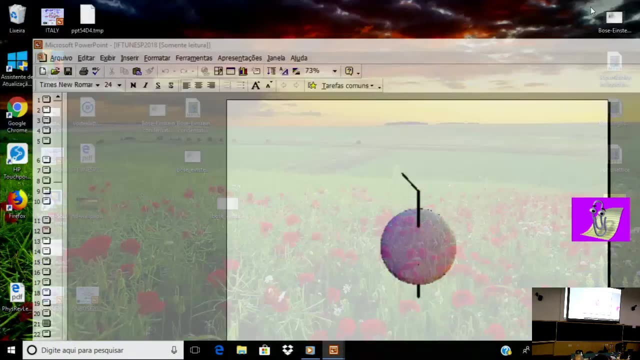 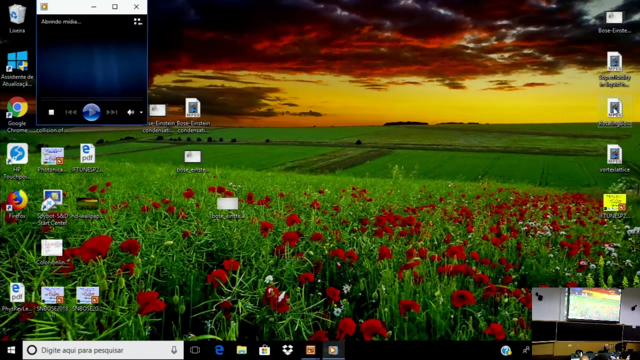 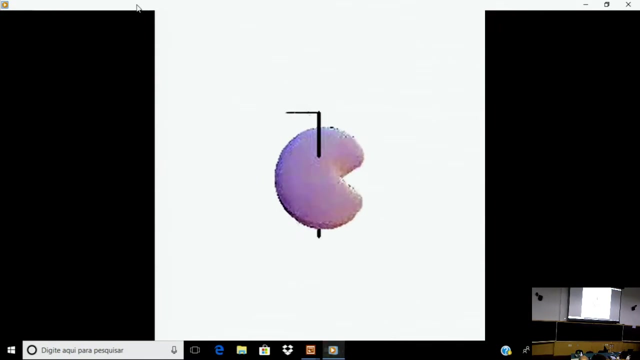 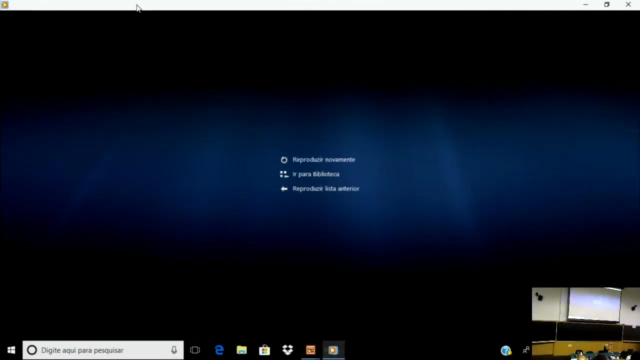 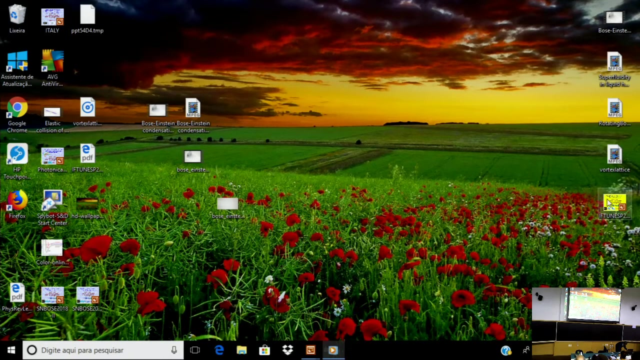 the following: that it generates a small, many small. it's not moving. This, you see in one of our. So the thing is that if you have 5 square, it's greater than 5 times 1 square. 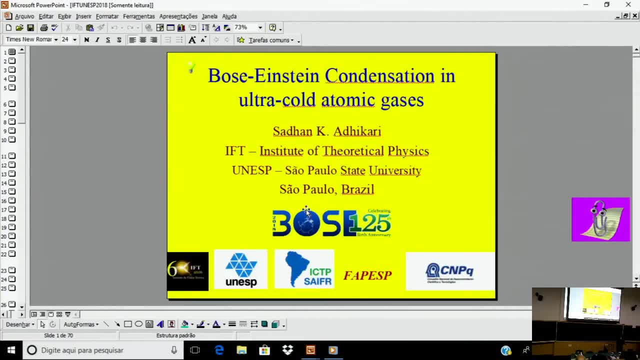 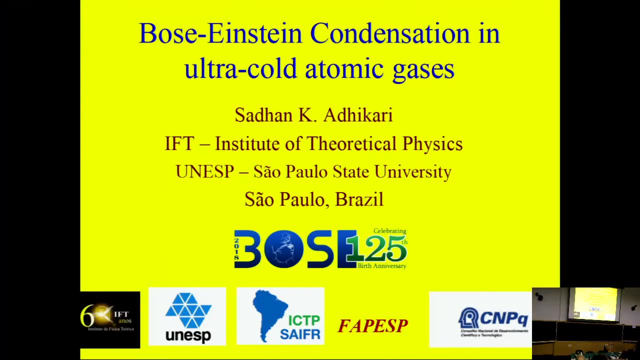 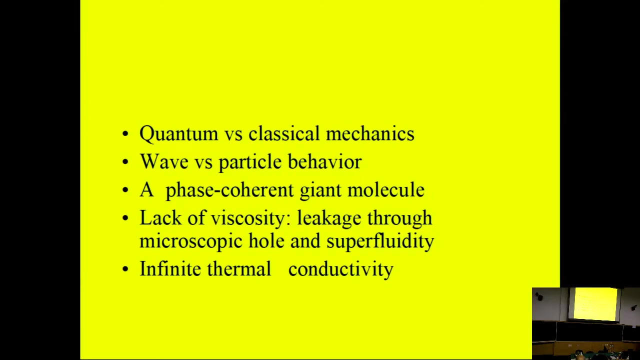 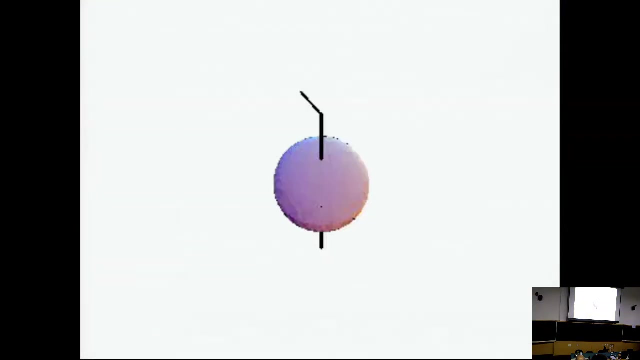 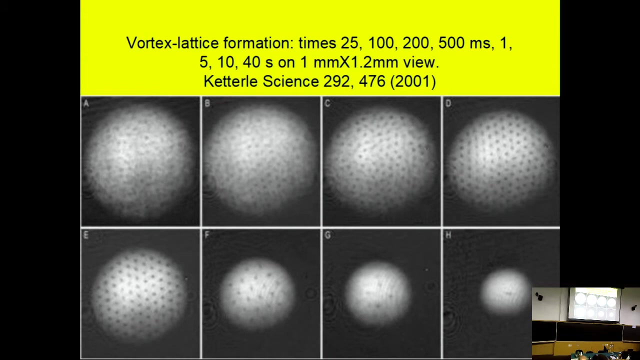 So in case of having 5 units of angular momentum, it's easier to have, energetically convenient to have 5, 1 unit of angular momentum. So this, each hole corresponds to 1 unit of angular momentum per atom. So you have. this experiment was done in 19, 2001.. 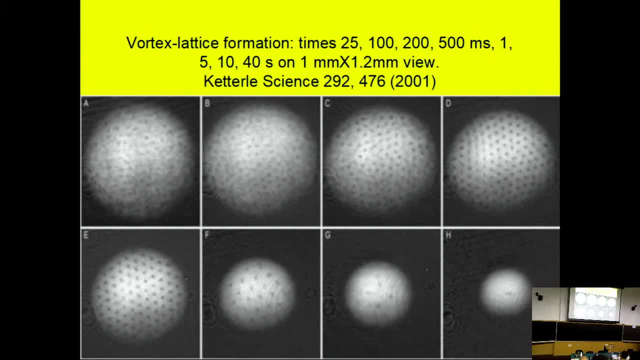 You rotate the Bose-Einstein condensate. So this is the time: 2500, 200, 500 milliseconds, then 1 second. You see here very beautiful lattice is formed. So each hole has 1 unit of angular momentum per atom when it is rotating. 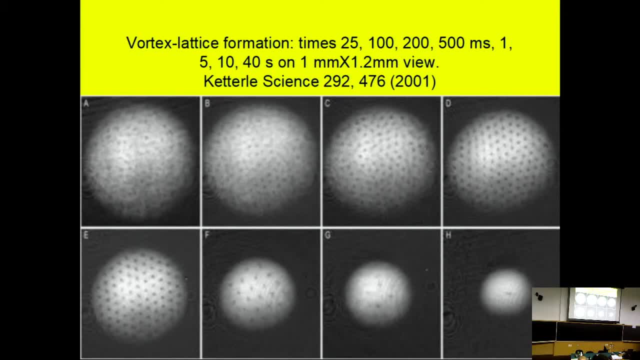 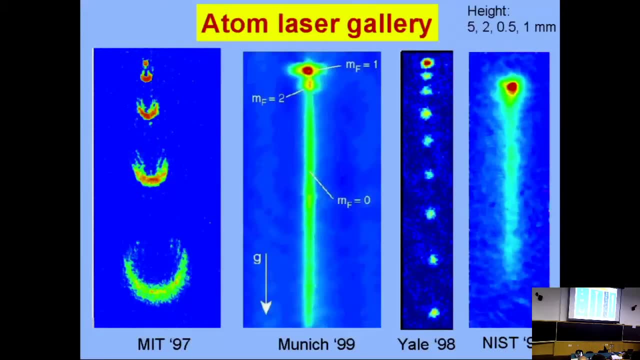 So it has so many units of angular momentum per atom, But it disintegrates in this way, Isn't it? This is an experimental thing, And then, with time, it's destroyed. This is the correct order. So you can make an atom laser, coherent atom laser, like optics laser, the coherent light. 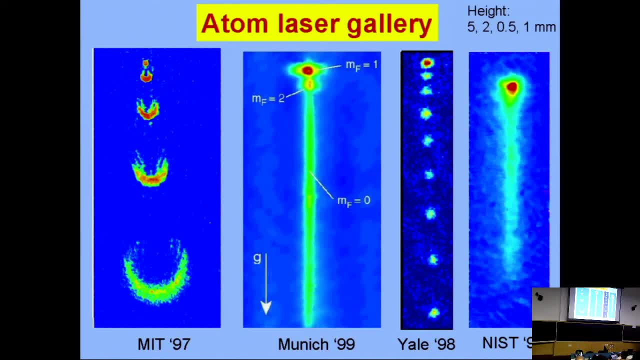 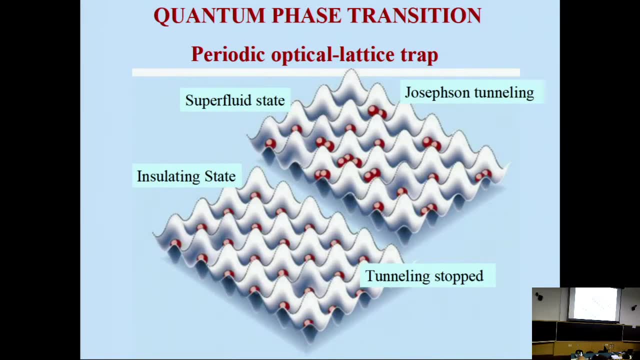 So you can do many experiments. So laser was made, but no, so far no experiment was done with it. Now we'll talk about quantum phase transition. What is quantum phase transition? For that, an ingenious experiment was done By periodic optical lattice trap. 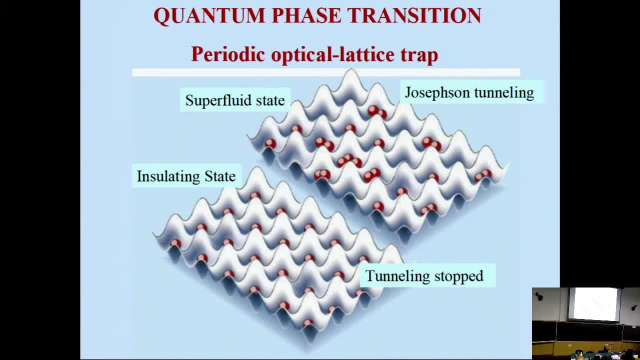 The periodic optical lattice trap was also an interesting idea. You have two laser beams, polarized laser beams, That means electric field pointing in one fixed direction between two mirrors. So laser comes this way and this reflects that way. So it's, this technique was known. 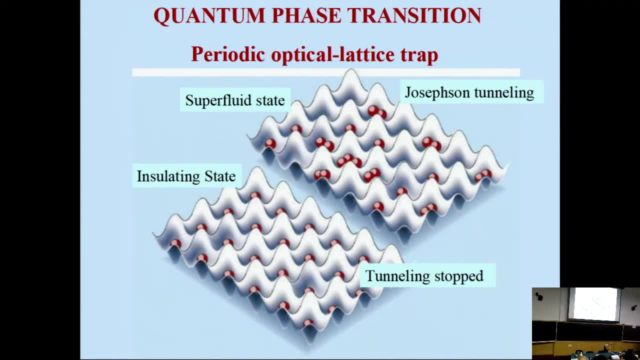 To keep a laser between two mirrors. So what happens? The laser carries a magnetic field perpendicular to it, propagating magnetic field. The other one will have a propagating magnetic field in the opposite direction. So superposition will make a stationary magnetic field. 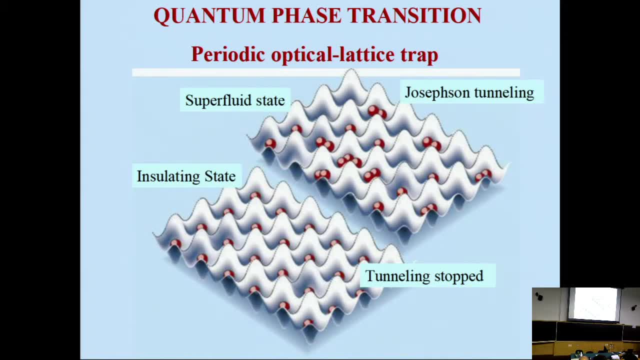 Stationary magnetic field because these atoms have magnetic moment. it gives a trap, So this will make a in two directions. if you have two lasers, This will make a trap like this. So it's a potential well, where you can put the atoms. 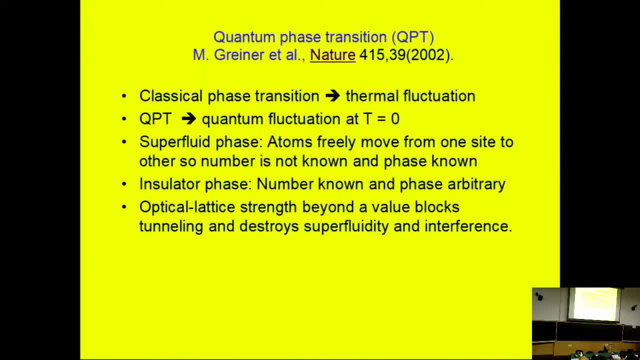 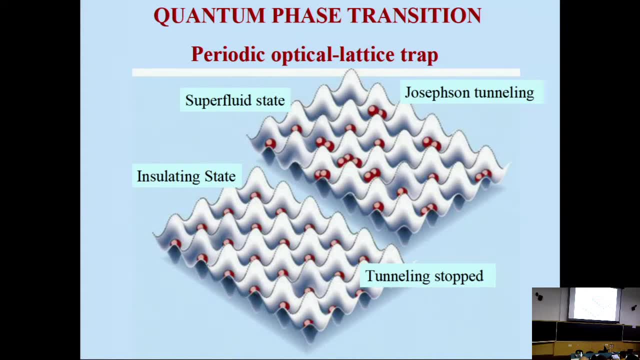 You put the atoms. So atoms can be in a superfluid state or in an insulating state. So if the atoms are there on top, the atoms are moving apart. It can move from one tray to another, one hole to another hole. 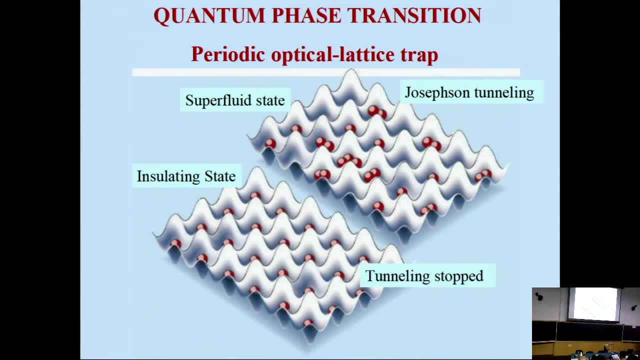 So this is a superfluid state. It can freely move. This is some kind of quantum tunneling, superfluid tunneling, which is different from tunneling in quantum mechanics. Tunneling in quantum mechanics takes time, like alpha decay. It takes months and years. 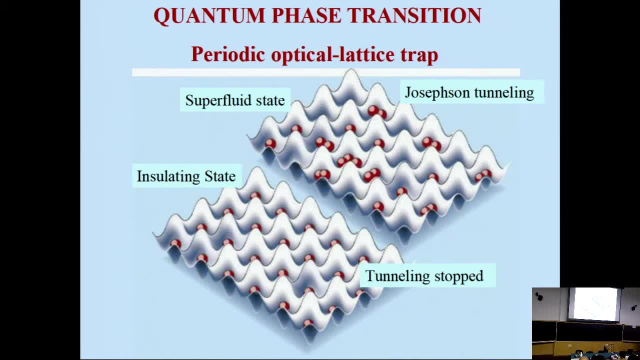 But this is instantaneous And this was predicted by Joseph Schoen by studying Schrodinger equation in his PhD thesis- A very interesting work. And if tunneling is stopped, then you have a situation like this. This is an insulated state and the superfluid state. 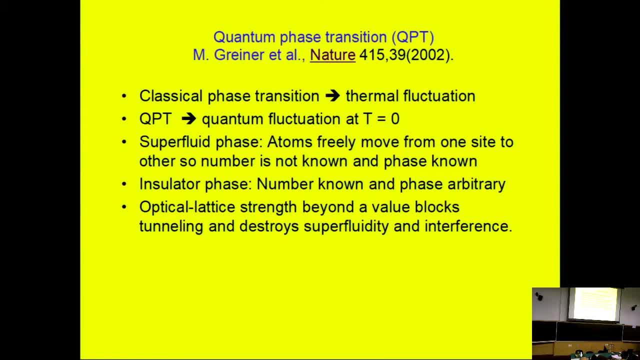 Now, the experiment was done in 2002.. So you have classical phase transition which goes by thermal fluctuation. You have to have variation of temperature. But quantum phase transition, it takes place because of quantum fluctuation At same temperature, 0 degrees Kelvin, you can have quantum phase transition. 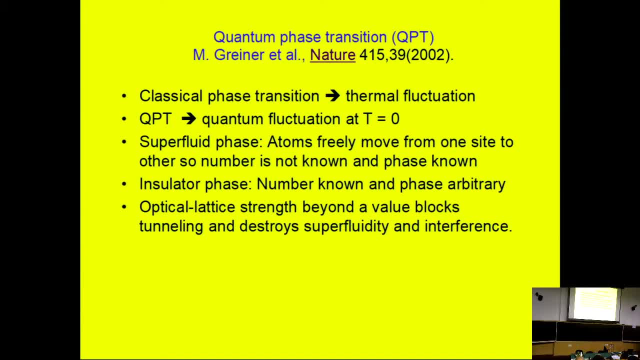 So superfluid phase is. atoms move from one place to another slowly, So the number is not known, but the phase is known. Each atom knows the phase of the other. It's a phase coherent state, An insulated state. the number is known. 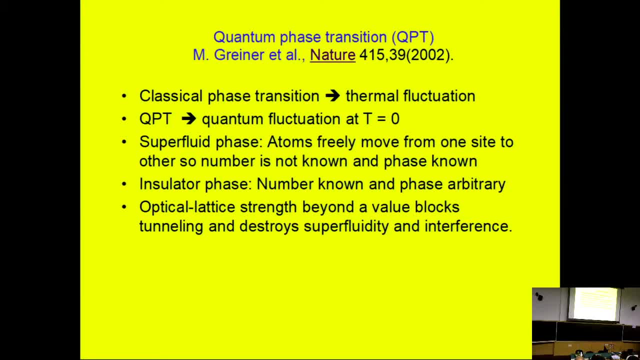 Each hole you know the number, But each atom does not know the phase of the other hole. So number known in the phase, arbitrary. So optical lattice trap: if it is more increased, if the intensity of the laser beam is increased, the trap will be higher. 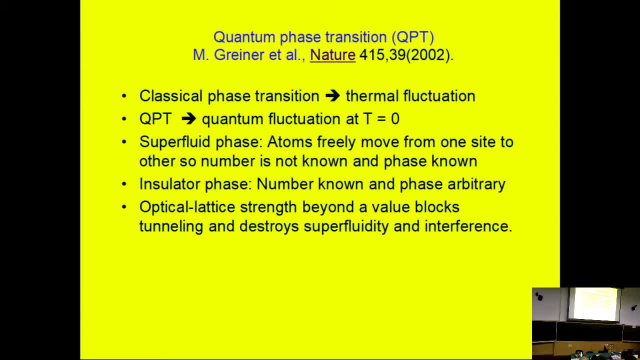 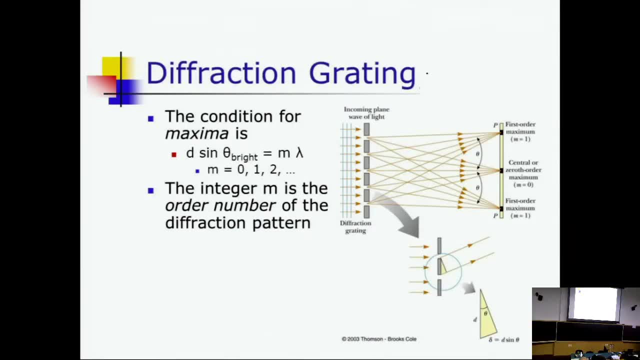 And this will make a superfluid state go into insulated state. So this is a quantum phase transition. This is like diffraction grating- How to detect it. So diffraction grating is that you have many holes through which a coherent light can pass. 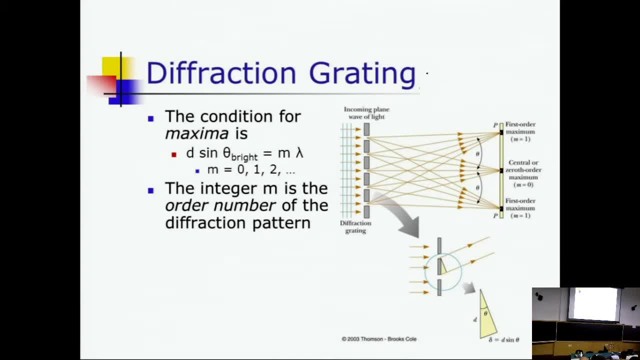 You saw that if there are two holes, you'll have multiple dark and bright places, But in this case all the other things are destroyed when the number of holes is very large. You have three spots. So what will happen if you translate it into Bose-Einstein condensation? 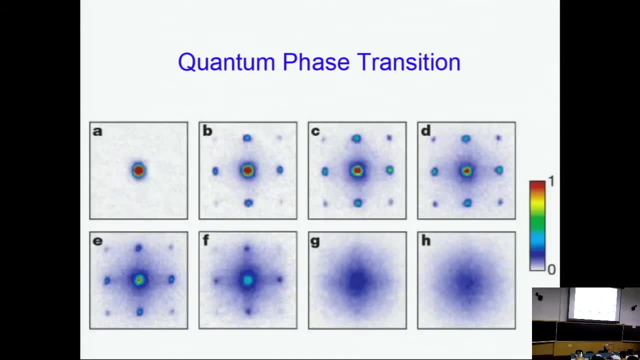 is two dimension. So you had that optical lattice trap And suppose that everything there is condensed here, size of the condensate here. Now you allow it to expand 100 times more. When you allow it to expand 100 times more. 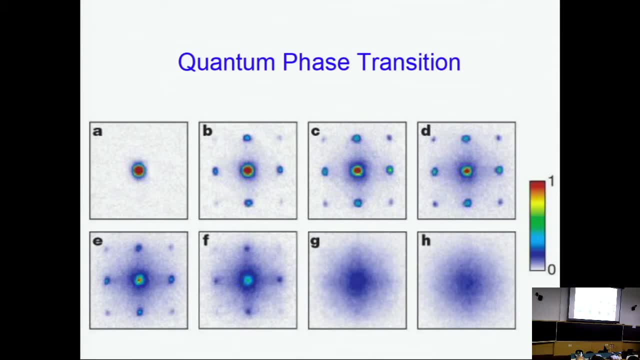 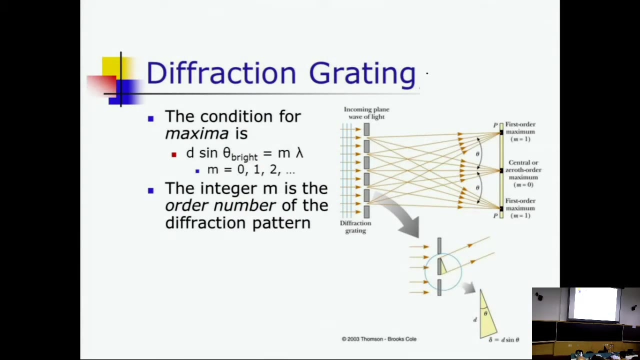 in two dimension, So everything happens in two dimension. So instead of this thing, when it expands, you will have these nine spots, Because one array makes three spots And a square box will make nine spots, So we have matter in nine places. 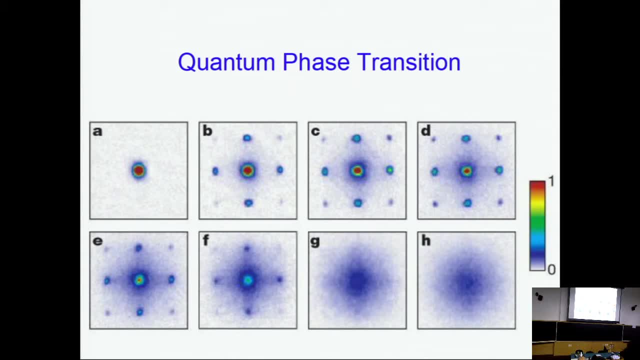 Here you are increasing the height of the optical lattice trap, So here the whole thing is coherent and superfluid. So we have these nine spots detected after removal of the traps And then making an observation after a long time when the whole thing has expanded. 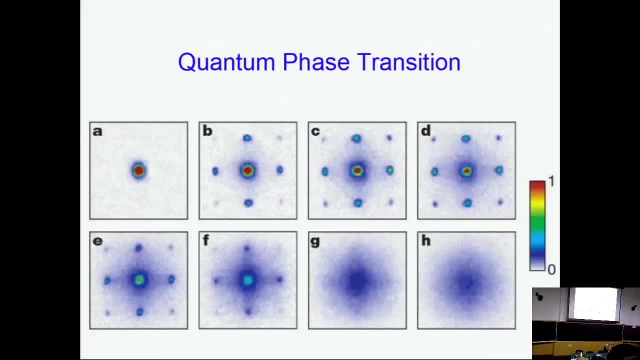 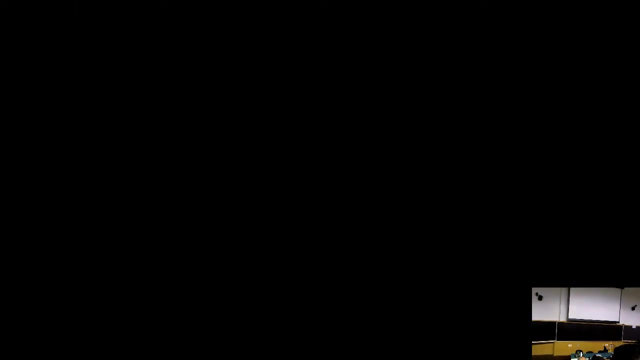 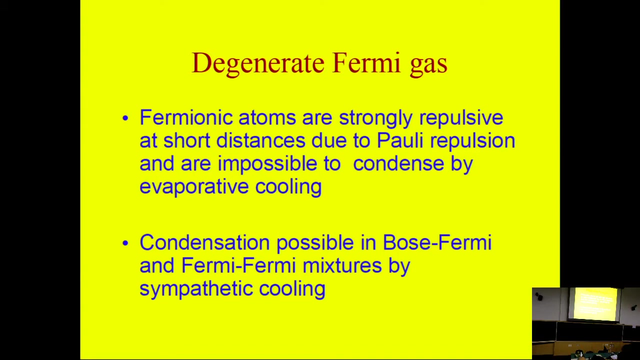 from a point size to a very big size, 100 times more size. But if the optical lattice trap is increased the interference pattern is lost. So you have a transition from superfluid state to insulator phase. So you can have whether Fermi gas can have similar things. 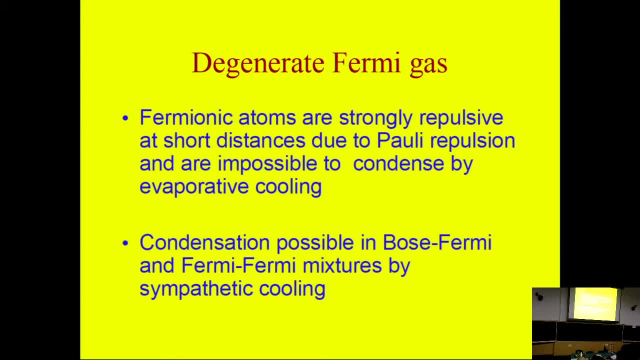 Fermi gas as such cannot have similar things. But if you can couple two Fermi atoms, spin up and spin down to make a boson, then you can have similar superfluid state And that is VCS condensation Bose-Einstein. 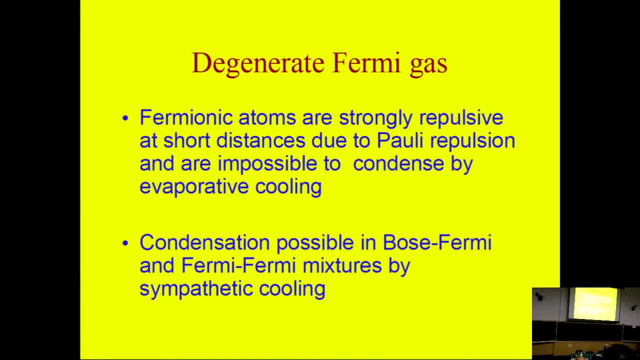 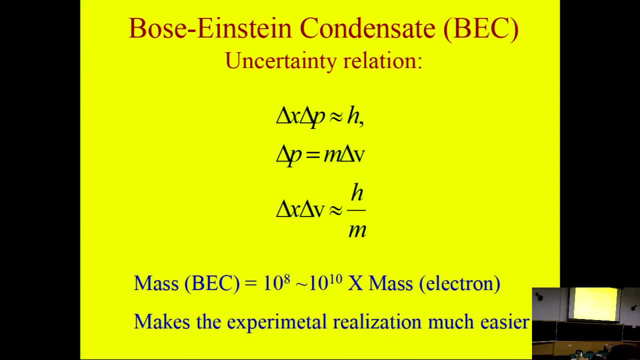 Baryon-Cooper-Schrieffer condensation, But I will not go into that. This has been also done experimentally. So what is the difference from textbook quantum mechanics? So you have the uncertainty relation: dx- dp equal to h, The dp. 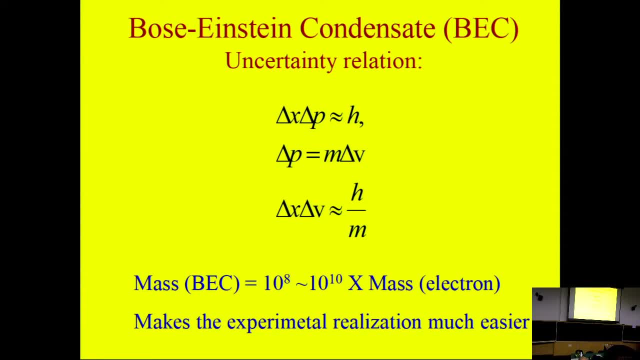 the uncertainty in momentum is mass times, uncertainty in velocity. So you have dx, dv, delta x, delta v is h by m. But mass of a BEC is roughly could be typically 10 to the power, 8, 10 to the power, 10 times mass of electron. 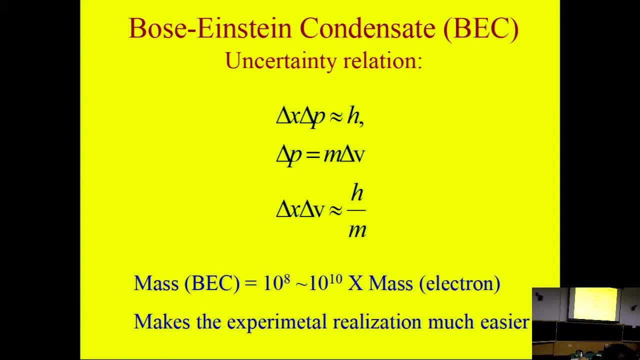 So this is practically zero. So this makes the experimental realization and study of BEC much easier, Because otherwise in textbook we learn that we cannot follow an electron, Because if we fix the velocity then you cannot have the position. The uncertainty in position will be infinite. 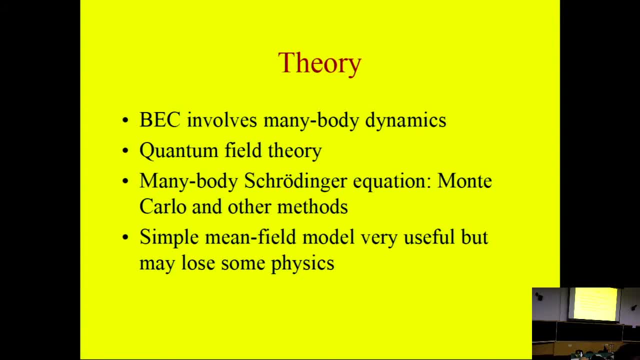 So you have to make a theory. BEC involves many body dynamics And you can do it by quantum field theory, Or you can do by many body Schrodinger equation and solve by Monte Carlo and other methods. So or you can make a simple mean field model. 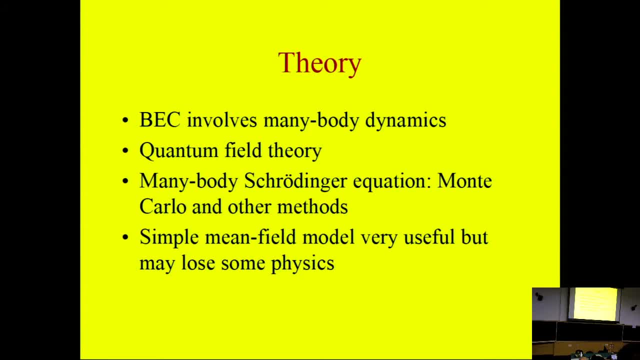 which is very useful, But may lose some physics. So if you are here at the level of Schrodinger equation, you already have lost some physics. because Schrodinger equation is a mean field equation, You have lost the photon degrees of freedom. 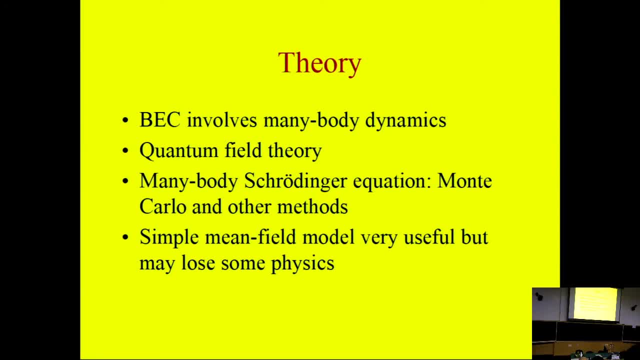 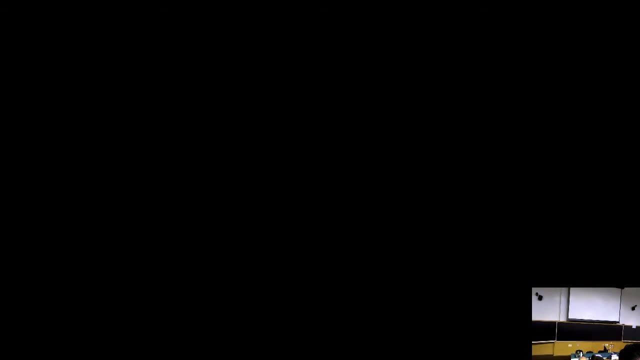 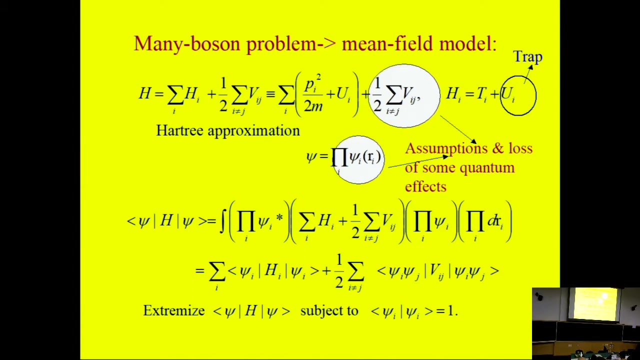 So you have lost lamb shift, which you have studied in undergraduate courses. So, assuming that that doesn't contribute anything to it, we'll make a simple mean field theory. So you can do it in different ways. I'll show only one way. 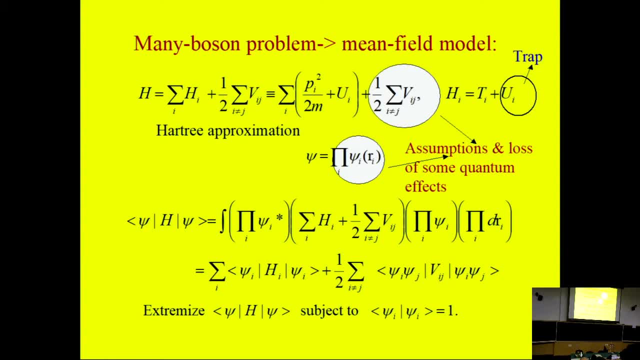 Starting from many body Schrodinger equation. So this is the Hamiltonian, This is the kinetic energy plus the trap, external trap, And this is the potential between different atoms. vij, They make an approximation which is called Hartree approximation. 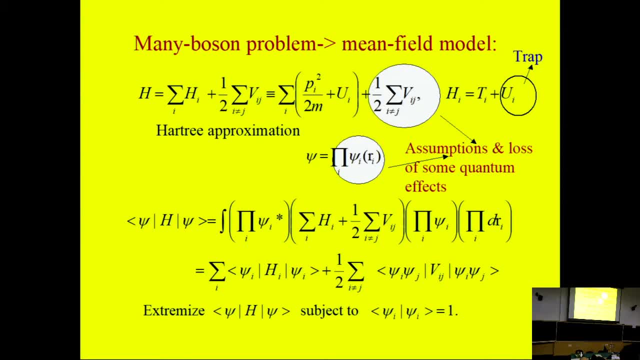 which, as the atoms are all in the same level, they occupy the same state And you can say that the whole wave function will be a product of wave functions, And there's not too much correlation. These are assumptions And some quantum effects will be lost. 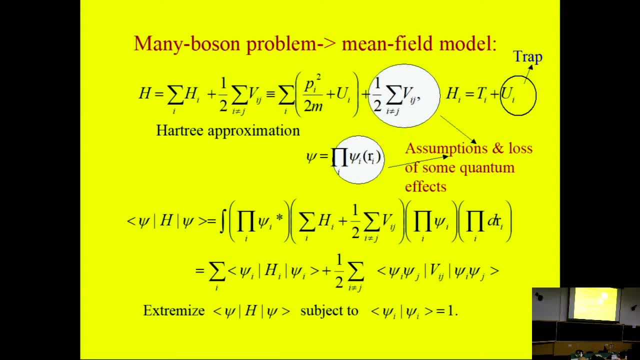 Because of these assumptions. Now we take the expectation value of the Hamiltonian. These are the two wave function on both sides And this is the integral over all atoms: i, number of atoms. This is the h, i, this part, And this is the potential. 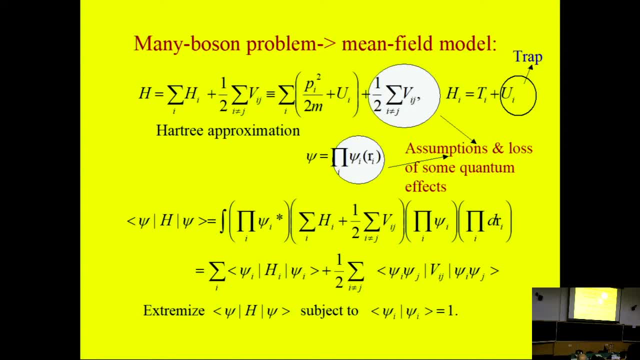 And easily you get this. This is one body term And these are two body terms Because they have two body potentials And you have two waves And you have two wave functions. So now we extremize this, Subject to the condition that this is one. 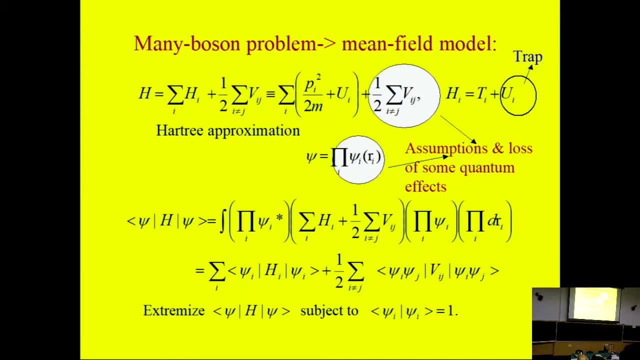 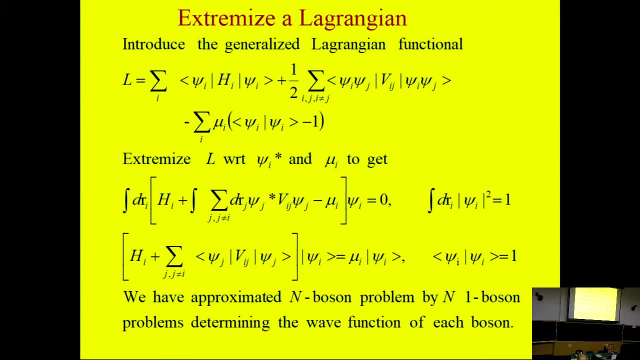 The easiest way is that why this Something is. So you used a generalized Lagrangian functional, which is that wave function, that that expectation value of Hamiltonian Plus this thing is the Lagrange multiplier. So you want to make this equal to one. 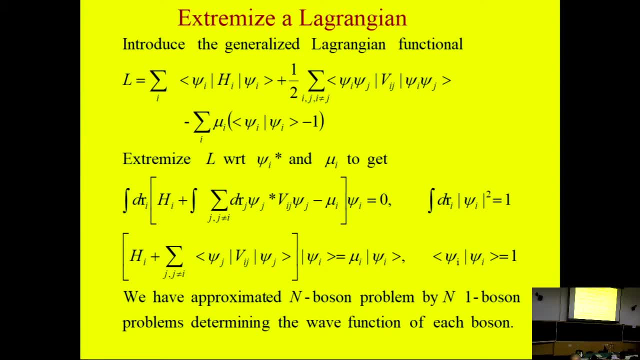 Extremize with respect to this, You get this equation and that equation, So this is a normalization equal to one. You derive. make derivative with respect to psi i, So you get this equation And factor of half is lost Because you have two terms. 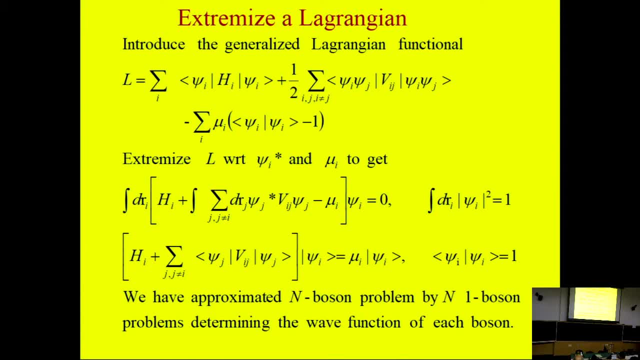 And this is the equation you will get, Because this is valid for all possible variations. So you take the integral out And this is the equation you will get. So you get many one body equations. Now this look like a Schrodinger equation. 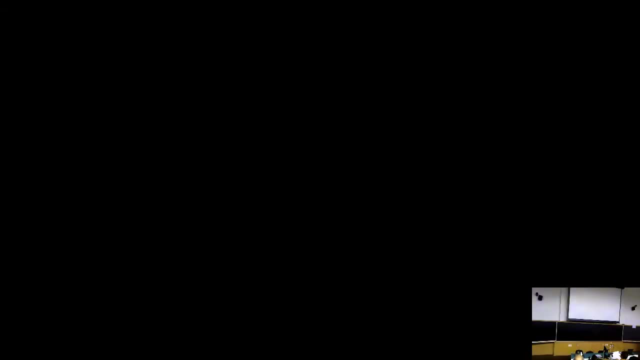 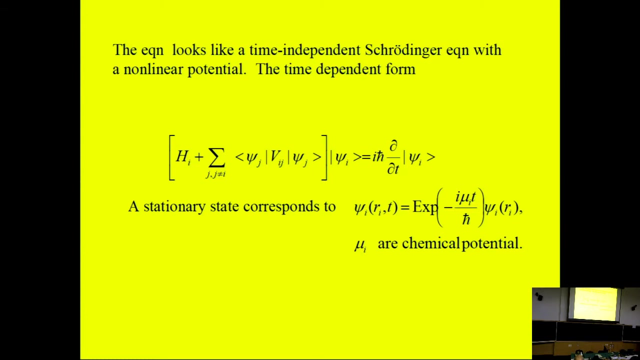 One body Schrodinger equation And you can have a time dependent form. You could have derived this time dependent form Starting from a more sophisticated Lagrangian, time dependent, Lagrangian functional, But we just introduce it here till it is possible. 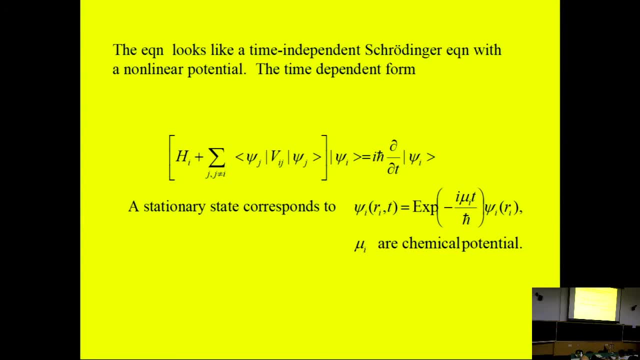 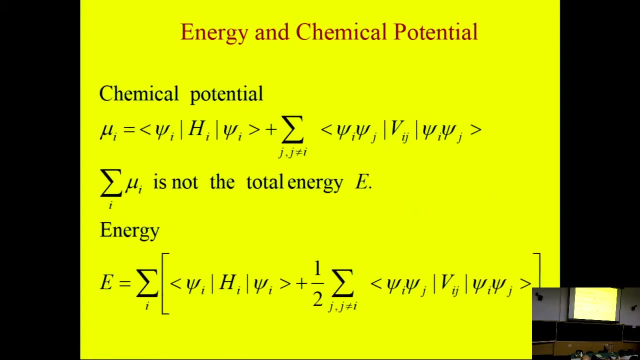 Now you do energy and chemical potential. This looks like a hydrogen atom Schrodinger equation, But this term is not the correct Hamiltonian Because when I derived we lost the factor of half. So this is chemical potential, the top thing. 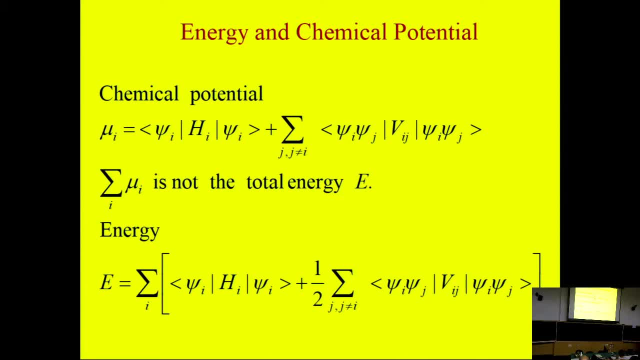 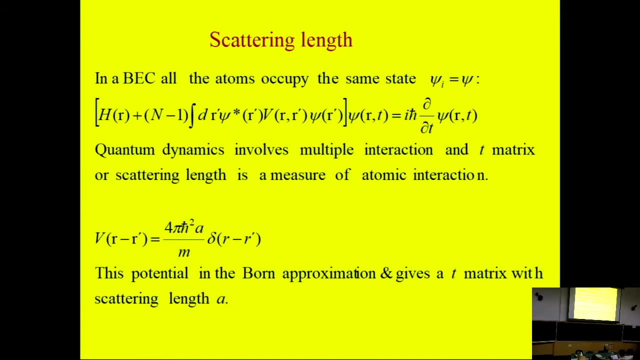 The factor of half is lost And the energy will be this, And that is the chemical potential of the non-linear equation. So in BEC all atoms occupy the same state, So psi, i should be psi And the I remove the i level from this equation. 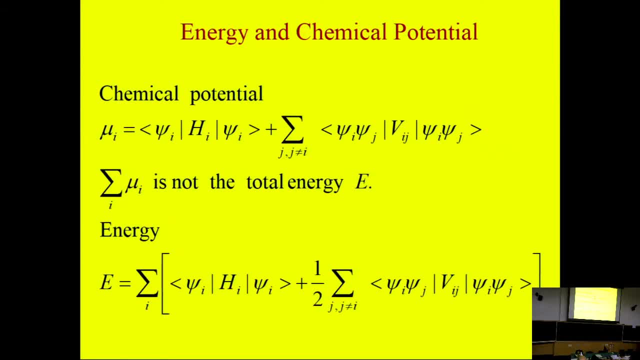 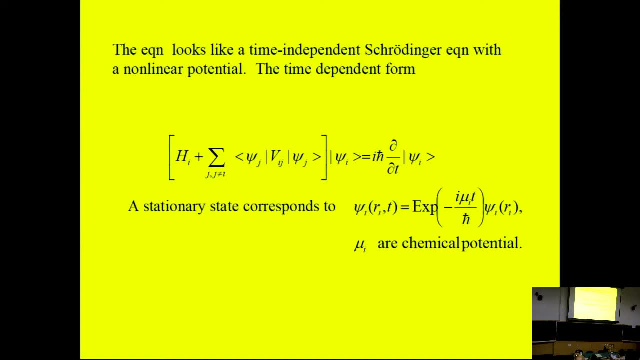 So this equation will become this. You see this term here. This can be immediately summed: V, 1, 2 and psi j is the same. It will get n terms And j naught equal to i, So it will be n minus 1.. 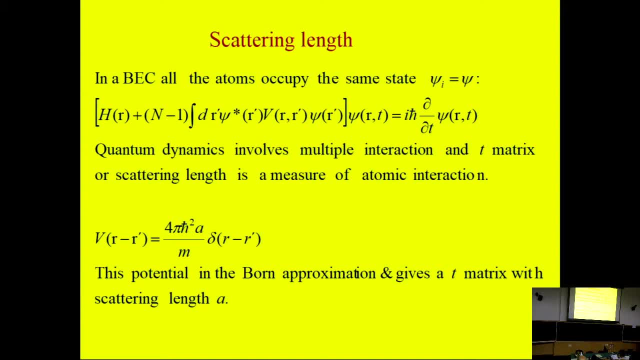 One term will be lost. But how do I use this equation? So quantum dynamics involves multiple interaction And the T matrix of scattering length is measure of atomic interaction. So we make this approximation a delta function approximation. For two reasons I take this: 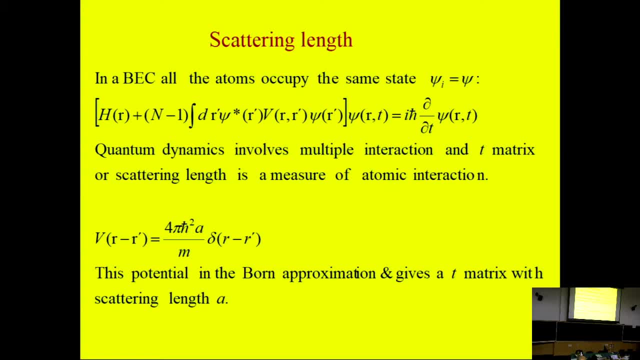 First, it is very dilute, So all details of the potential will be lost. So we have a delta function And in Born approximation this gives the T matrix. So you take the Born approximation and a is the scattering length. So you put this into BEC. 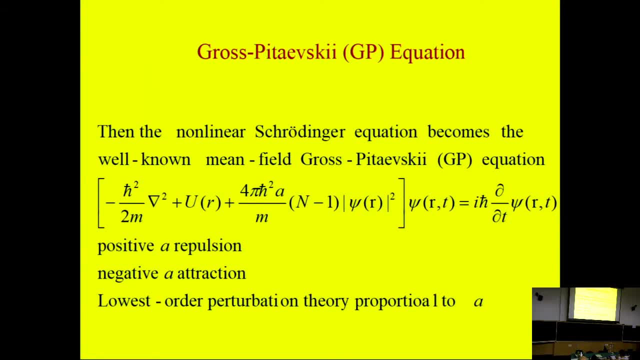 you can do the integration immediately And you get this equation. This is the mean field Grosbe-Typski equation which is used to study a condensate. The scattering length can be positive or negative, So if it is positive, the condensate is attractive. 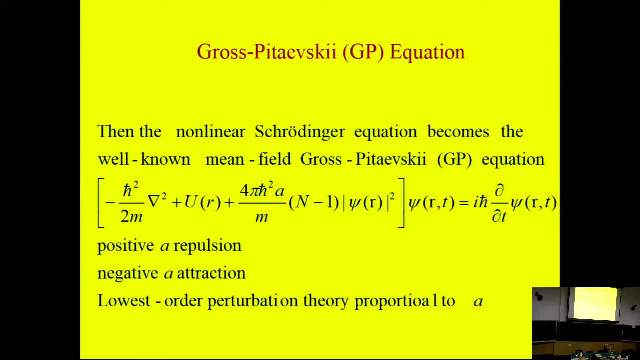 repulsive And if it is negative it is attractive. So we have this is the lowest order perturbative equation, proportional to A. like first order perturbation theory, You will have correction terms which will be higher order in psi square. This is a non-linear equation. 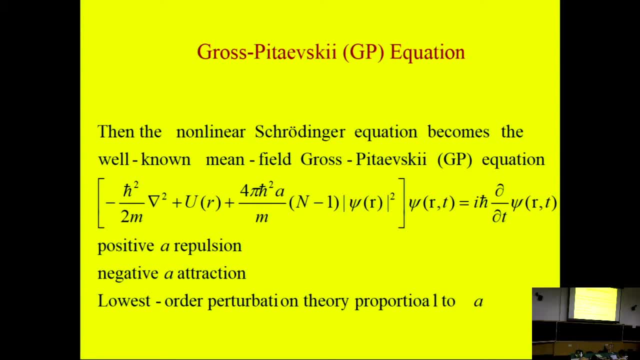 What is capital N? again, Capital N is the number of atoms, total number of atoms, And this could be, This could be 1 million. So this term is wrong. This term can be very large. This term can be very large. This term can be very large. 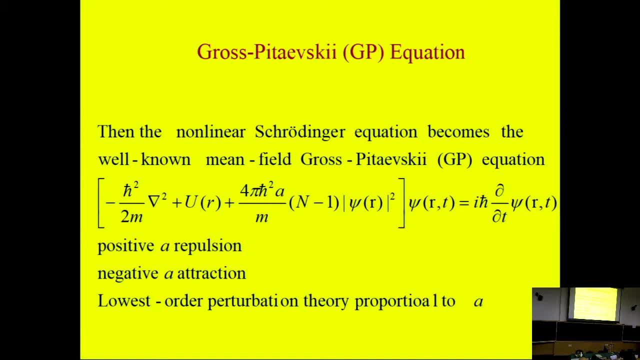 Especially when the number of atoms increases. Then you have an approximation. You can neglect this term because this is very slowly moving. So this term will be large. So you can solve this equation very immediately. The derivative is not there. You put a mu here. 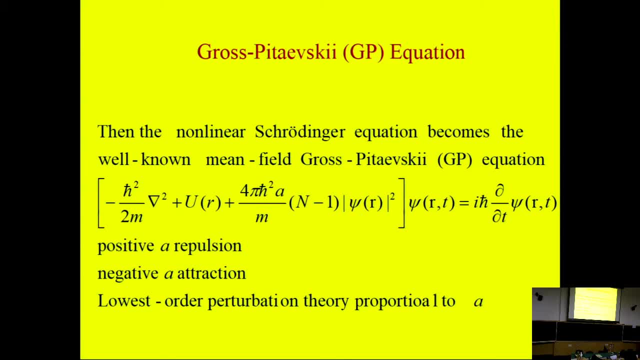 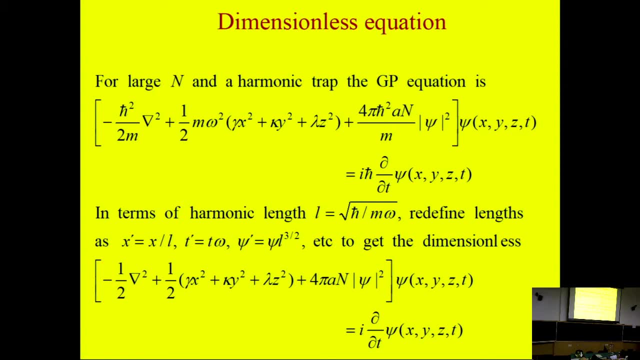 and this psi goes out. You can solve it immediately. You get the wave function. You can write a dimensionless equation, which is very common In physics. write this: This is the track, This is the equation, And you write this equation. 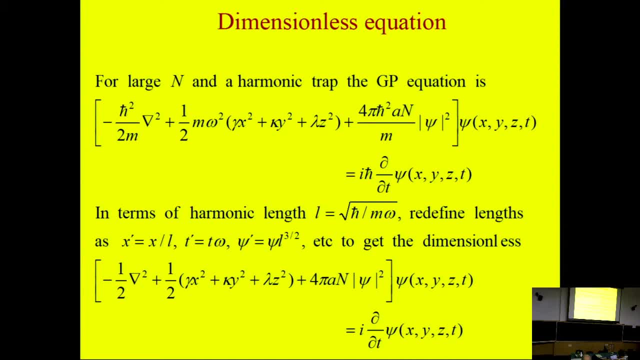 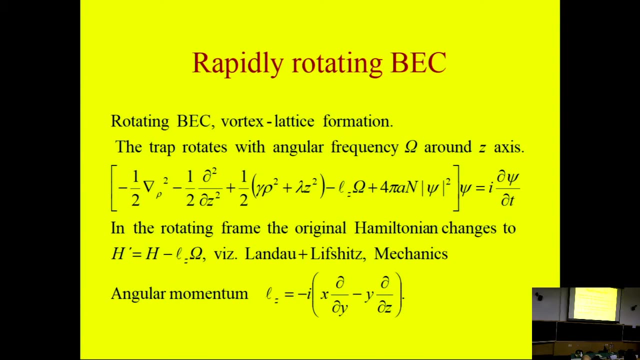 And you have a transformation which takes this to this. Usually you study this equation because you don't have h, bar, m, c, Everything is 1.. So if you have a rapidly rotating BEC, Let us see if this equation can explain. 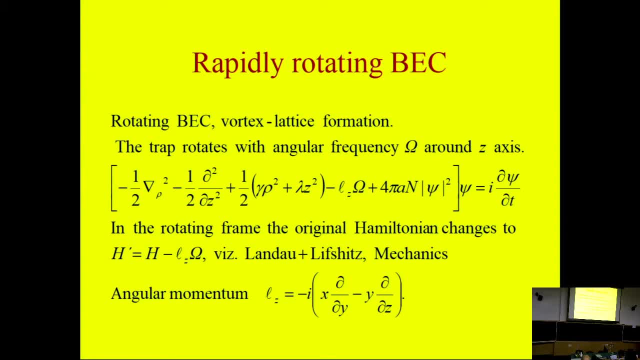 the properties of a rapidly rotating BEC. The trap rotates with angular frequency, omega, around z axis. This is the equation, This is the kinetic energy term, This is the trap And this term comes because of that. So how will you study a rotating BEC? 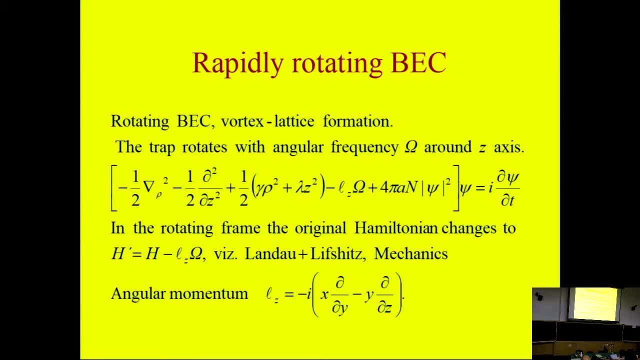 And we are observing from outside. So in the rotating frame the original Hamiltonian changes to that And if you can go to the rotating frame, it's a stationary problem. So this was given by Landau and Lipschitz And Landau used to study this. 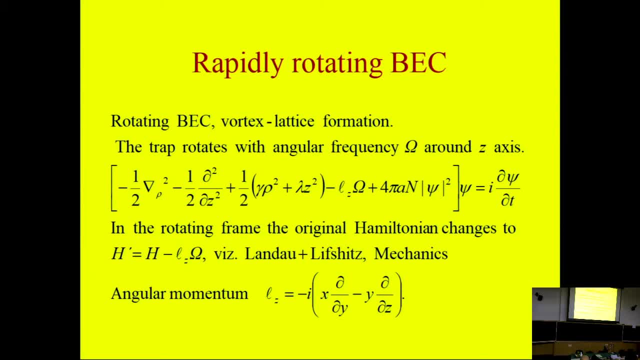 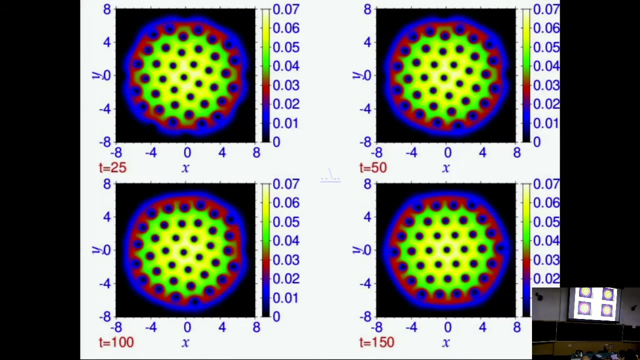 He studied this thing at that time, 1940s, So he knew this. So the system is rotating. You go to that frame And this equation will give the stationary And this is momentum. So if you solve this equation, you start with a Gaussian state. 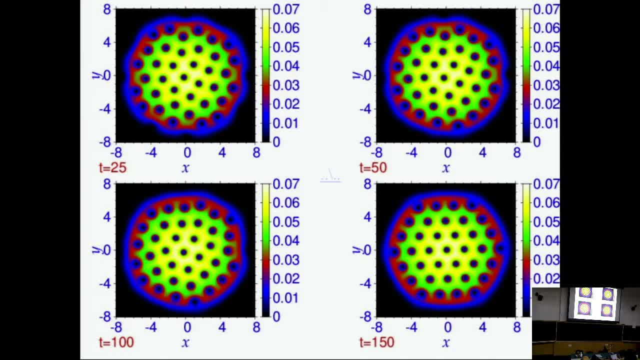 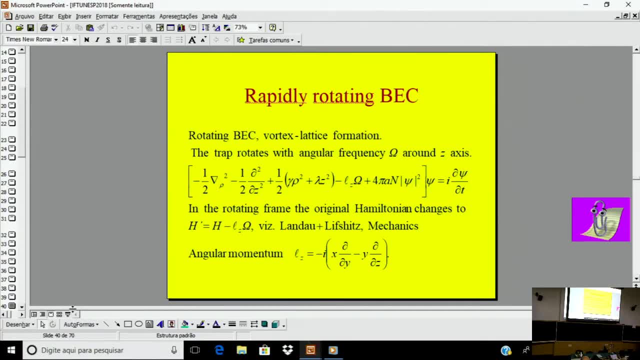 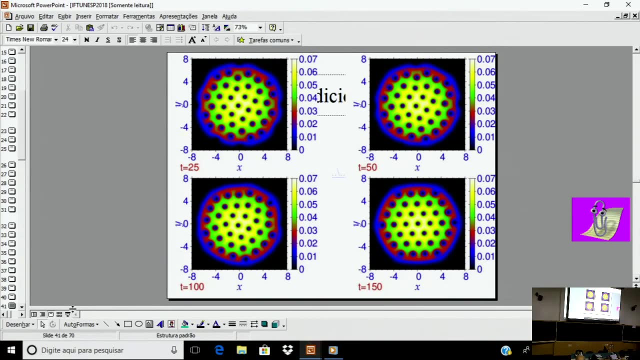 And then it starts generating vortices. So this is, after you iterate the equation for taking a Gaussian solution For psi And keep on iterating it, Calculate it next time, next time, next time. You see, after a unit of time, 25,. 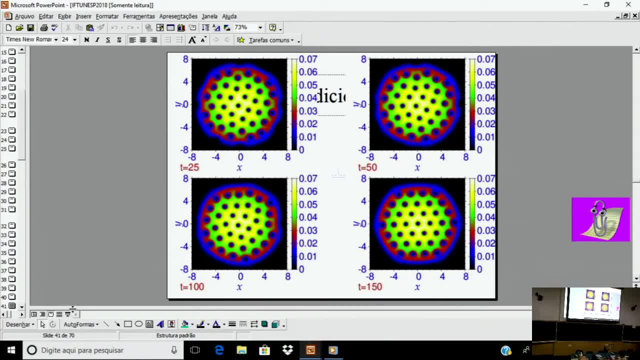 it has generated vortices After a unit of time, 50, it is more organized, It's 100. At time 150, you see, it is a perfect triangular lattice And that is the perfect condition to have the minimum of energy. 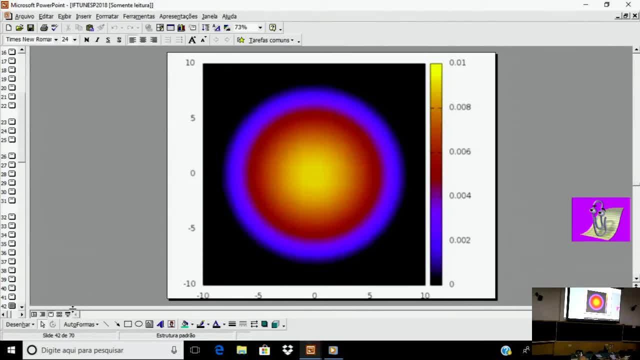 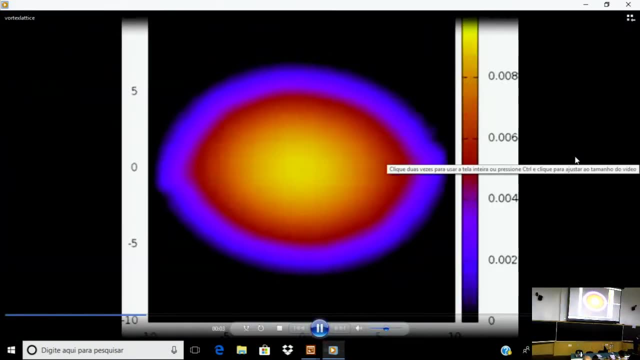 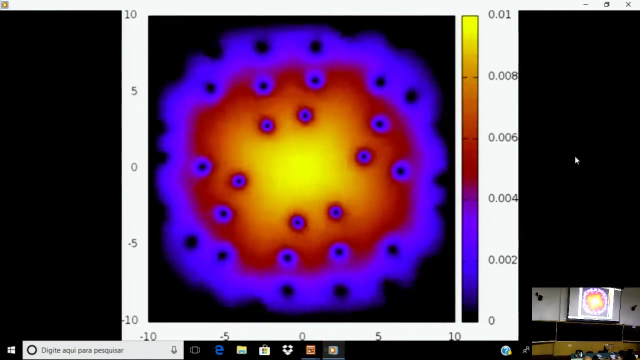 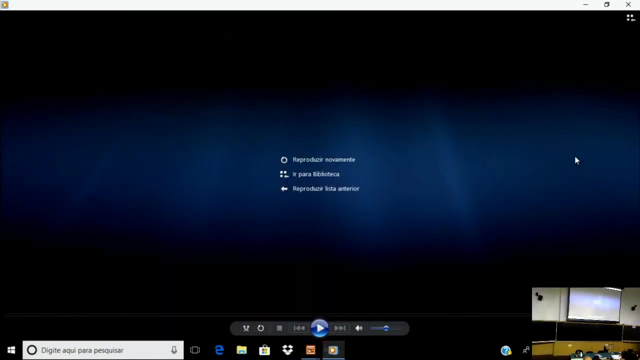 This will not play. I'll take again, I'll show how it develops from a Gaussian state. The Gaussian state, and time is increasing. These are the vortices: The Gaussian state, and time are increasing. 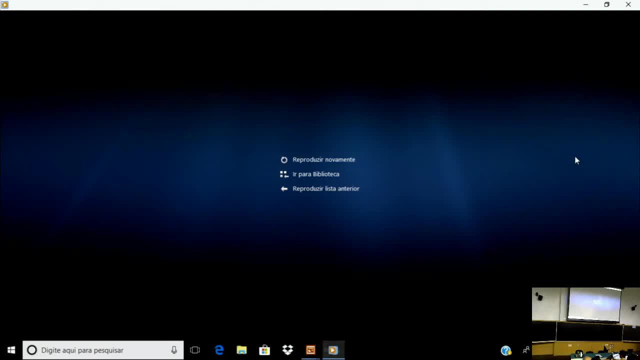 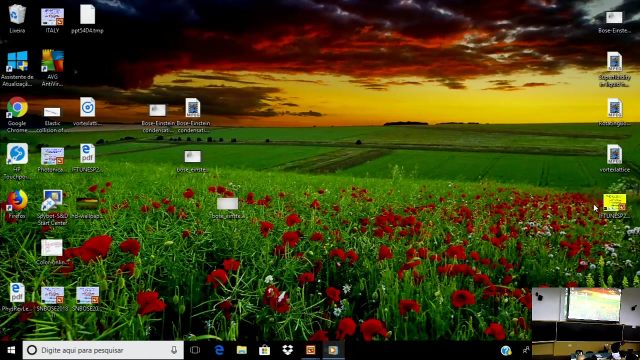 only that This is two-dimensional, but it could be three-dimensional, because then it is rotating. When I talk about angular momentum, it is rotating always about an axis. It is. 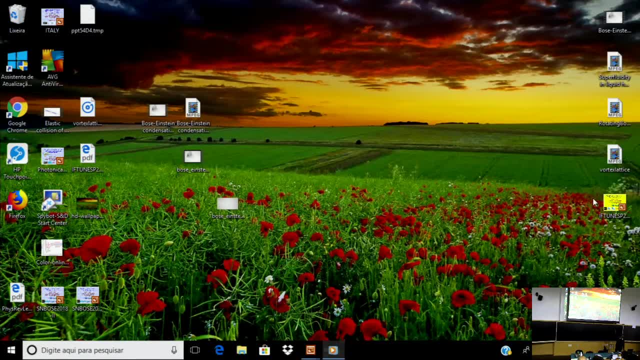 not the angular momentum quantum number of hydrogen atom, which is in spherically symmetric coordinate, It is axially symmetric coordinate and quantized version of L square is L square, not L times L minus, L plus 1.. Say it again. 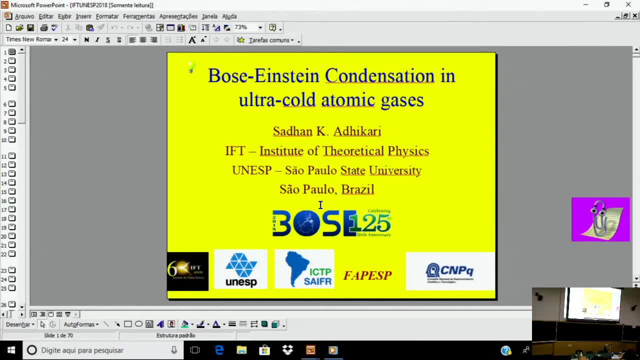 Yes, you take a size sufficiently bigger to accommodate the whole system. Suppose imaginary time. this is: the BC is 50 micron. You take a size of 100 micron, then it is okay, And then you force the wave function to go to zero at the boundary. 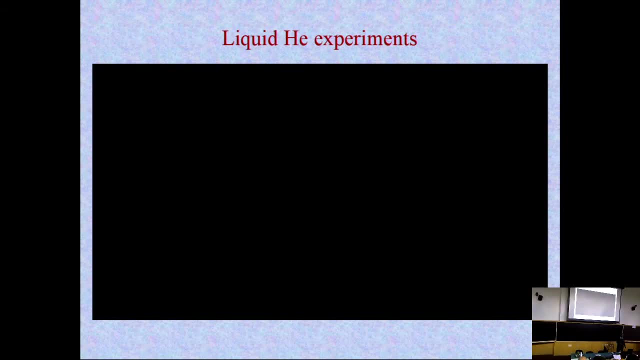 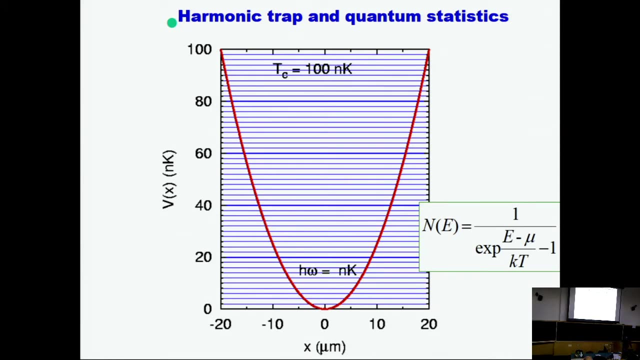 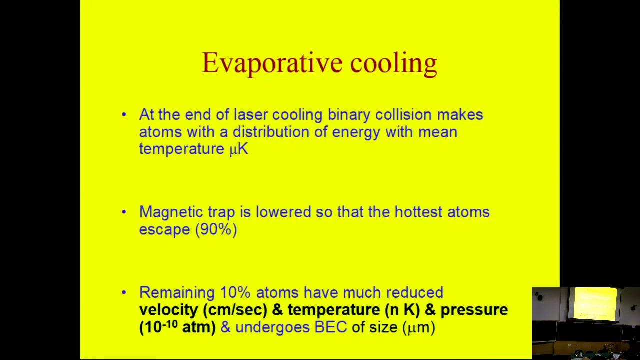 Sir, why is? there is some reason why it is triangular. shaped of this, like That minimizes the energy In case of very weakly interacting system, dilute system. Some basic intuition to see why this is termited? I don't know the intuition, I don't have the intuition. It was predicted by Avri Koshav. 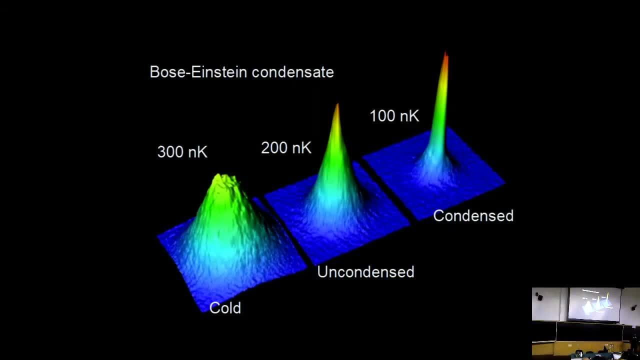 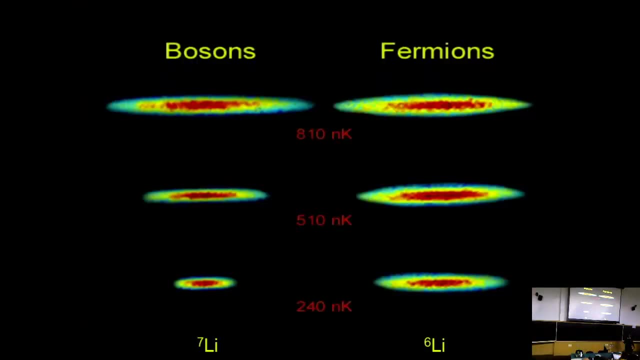 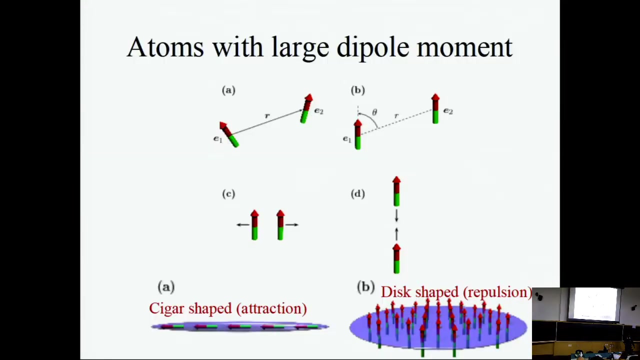 in 1957, completely theoretically. There is no experiment, nothing. He said the triangular lattice will minimize the energy And this was detected much, much, much later. He got Nobel Prize recently. So the angular momentum is fixed at the initial position, right. 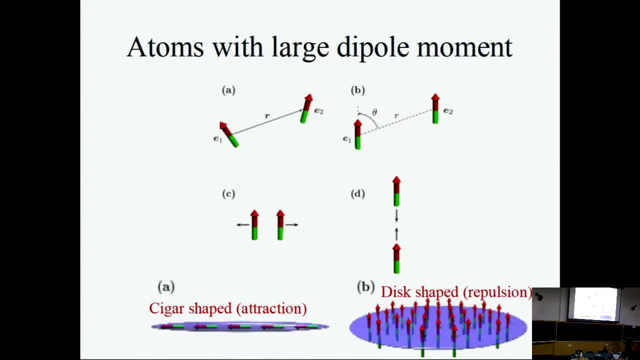 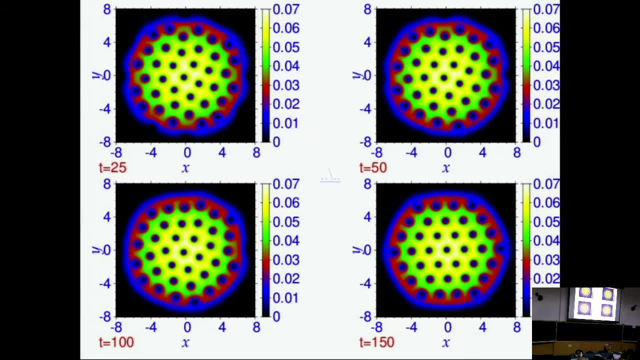 Right, Of course, angular moment: No, the angular velocity will fix the angular momentum. Right, so it sticks by the ratio. The omega Right, so it sticks by. so if you put it by hand, what omega is right? 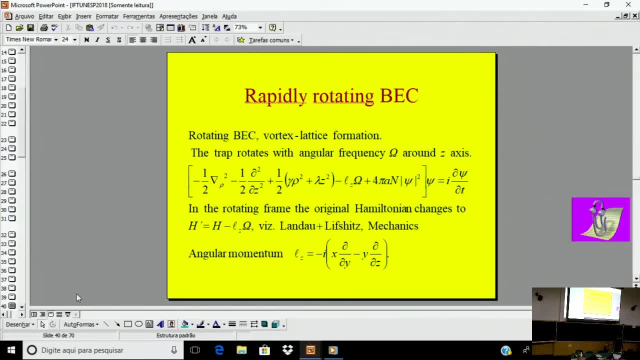 We put it by hand. what omega is The number of vertices that will form must be the, n should be each vertex should have 1 unit of angular momentum. Yes, per atom, 1 unit of angular momentum per atom. If you have 1 million atom, then 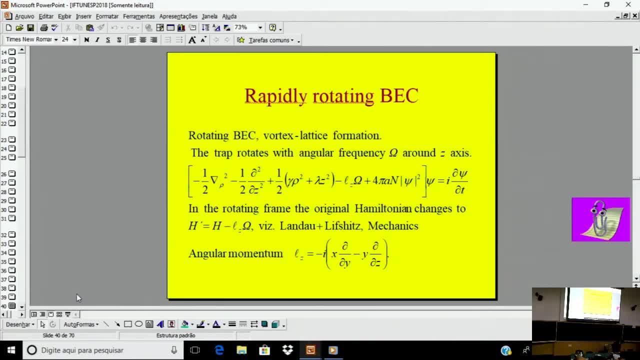 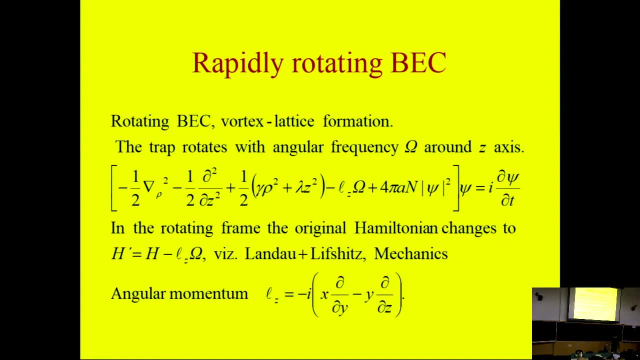 total angular momentum is 1 million h bar. Yes, say go. Is the wave function for a single, what you call atom, right, So that the solution is shown: Single atom or it is identical: The wave function for the single atom. 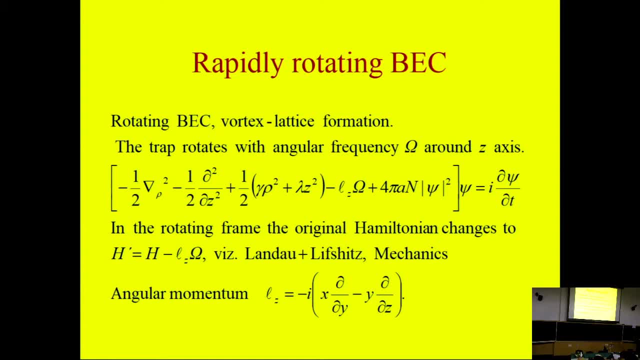 The wave function for the single atom is identical to the wave function of the BEC Bose-Einstein condensate, Only the intensity will be higher. Okay, It is the same wave function, And what I showed is the single wave function. 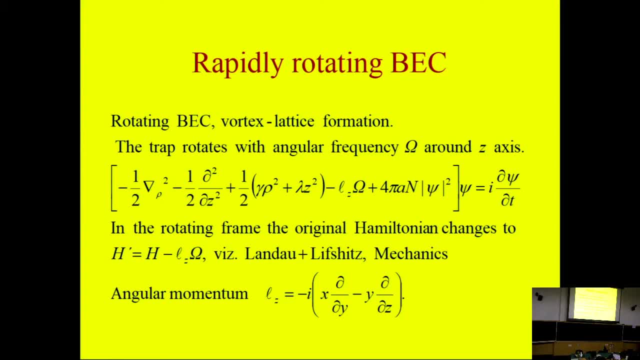 In the solution you showed us, there is no trapping potential anymore. it is just No. no, this is rotating with the trapping potential. Yes, the trap is rotating And I am calling for the diagonal classes, perhaps 1,, 2,, 3,, 4,, 5,, 6,, 7,, 8,, 9,, 10, 11,. 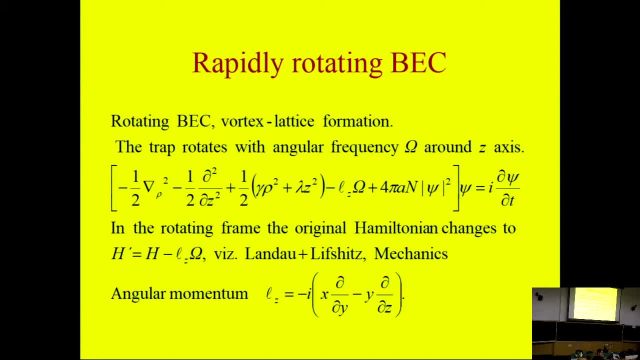 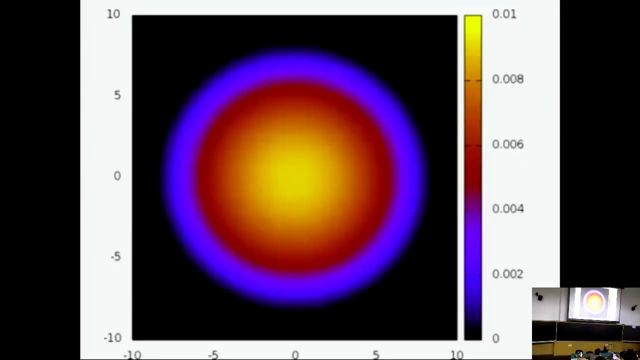 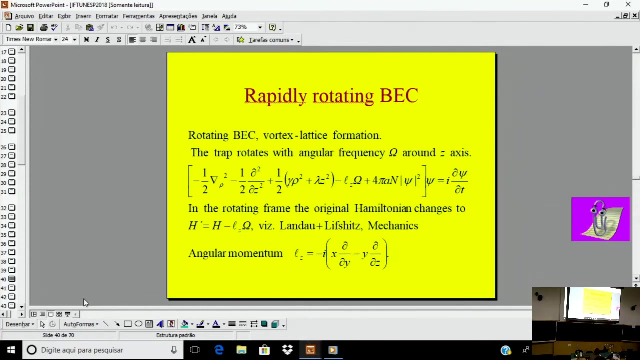 12,, 13,, 14, 15.. No, once you, yes, once you increase this angular momentum, the number of vortices will increase because it will be turning rapidly. Once you increase this angular velocity, it increases. 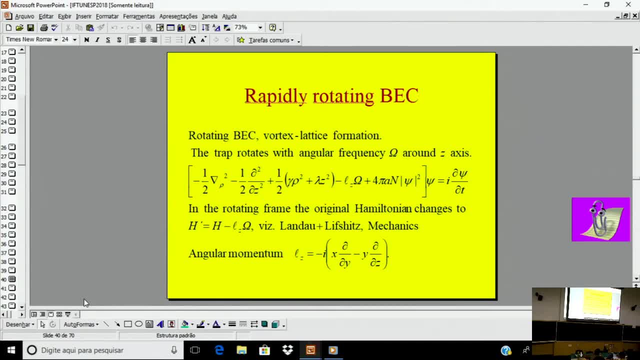 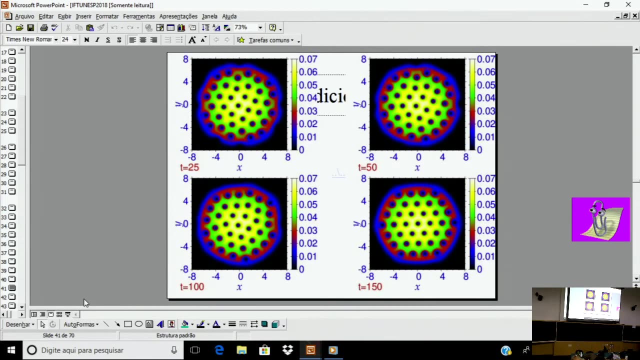 And once you increase the non-linearity, it also increases. A linear system does not generate these vortices. So if you make this 0, there is no interaction. no vortices will be generated, Dependent of how fast you rotate the quantum system. 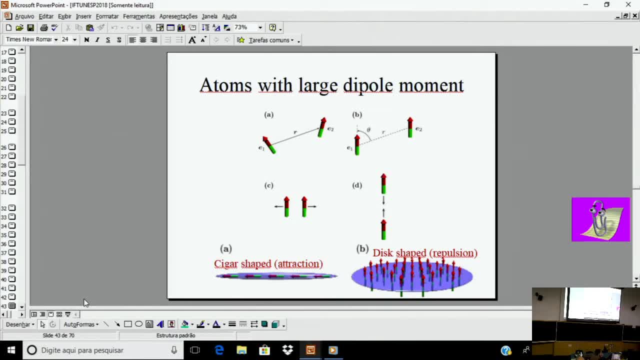 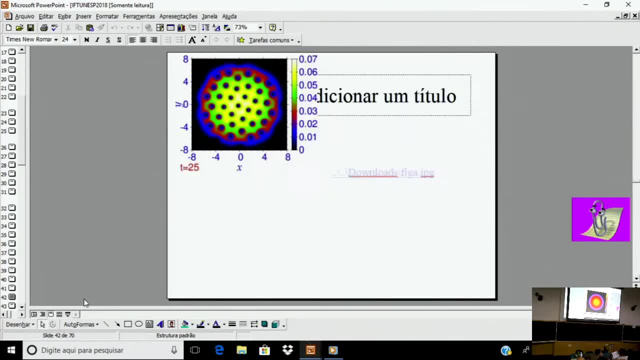 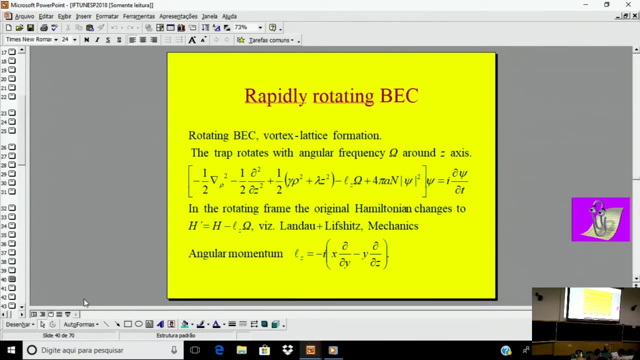 Sir, Sir. one last question: Where is the assumption that you have a weak interaction system In the A? you showed No, the number of N and A. A is small. N is small If A goes to infinity, the scattering. 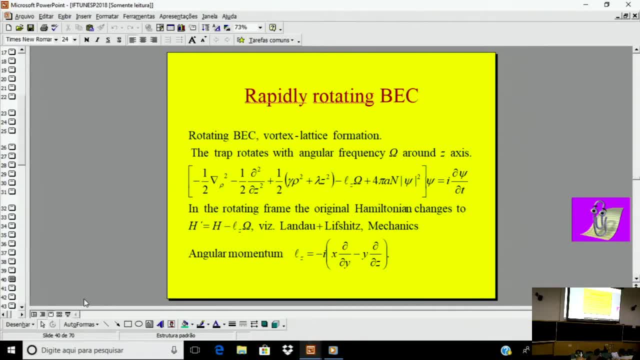 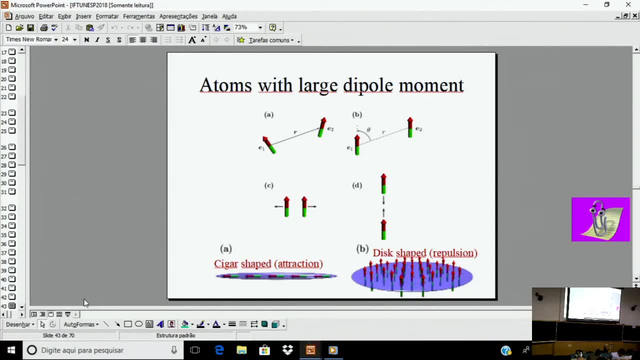 layers goes to infinity. you have a strongly interacting system. So you can have dipole moment. So you can have Bose-Einstein condensate with atoms with dipole moment. The atoms we consider, they have dipole moment. hydrogen atom, rubirium atom has dipole moment. 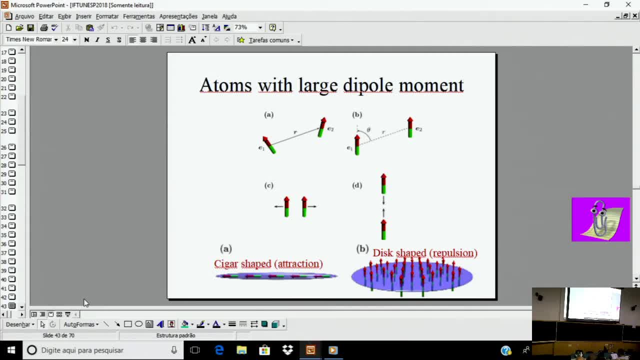 but it is one unit. But there are atoms which, for some strange reason, the electrons start occupying one electron in different shells, So it can this way accumulate 5 units of angular momentum or 10 units of angular momentum. Usually normal atoms- they are always coupled, spin up and down, So angular momentum will. 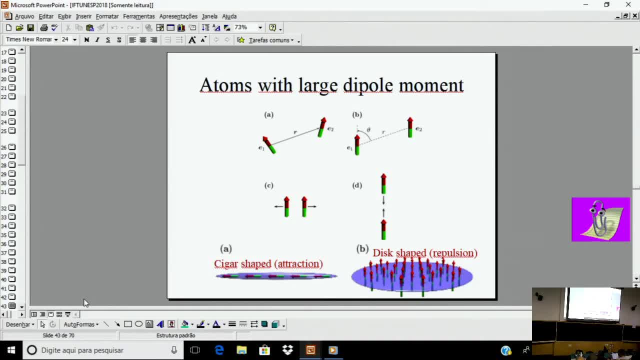 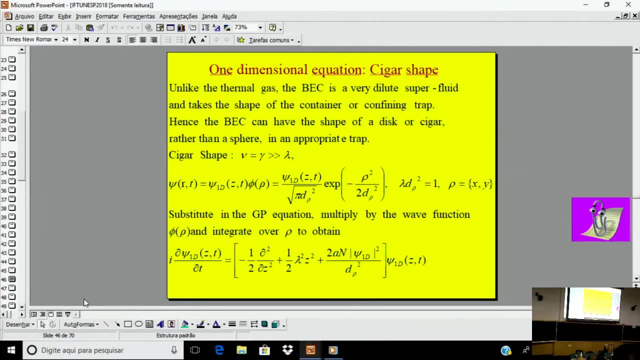 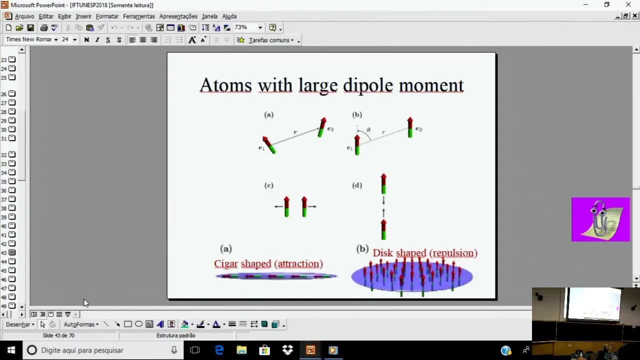 be 1 or 0, something like that. So there are atoms with very large angular momentum And you can form a condensate with these atoms, And then the atoms are like this, tiny magnets. You can have this interaction between them. So they prefer this figure-shaped attraction. 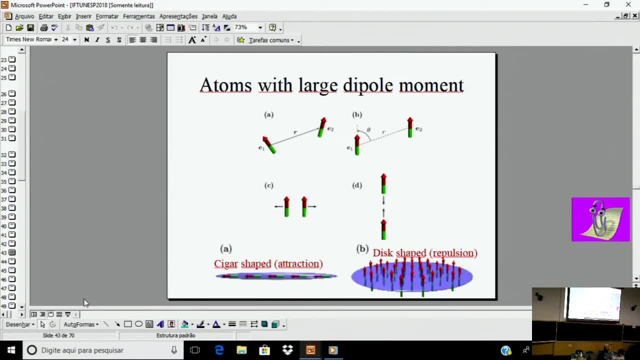 So it has an extra attraction. So if there are 10 atoms like this, highly magnetized, they will just form a chain and will not will be bound by themselves. They can be bound by themselves, Provided you can put in a line, but if you force them to put here in this, 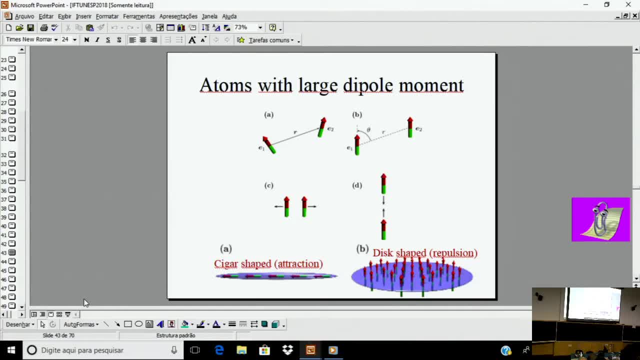 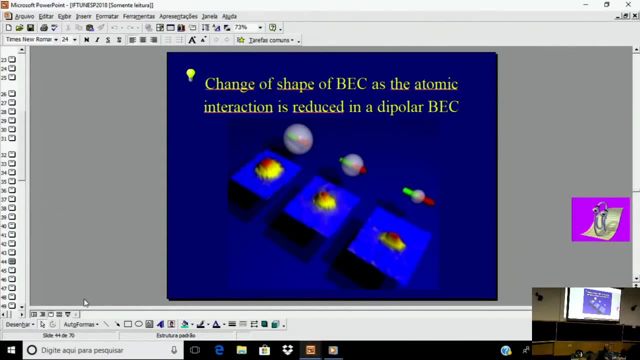 fashion they will be repulsed. So external trap, it puts it like this: It will be easily attract and form a condensate. So what happens? if you have the magnetic moment, then the shape changes. you see It. 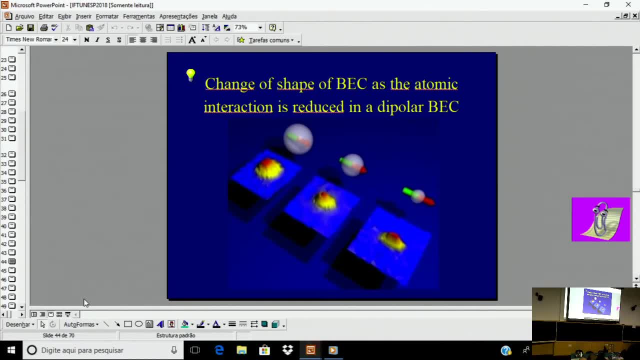 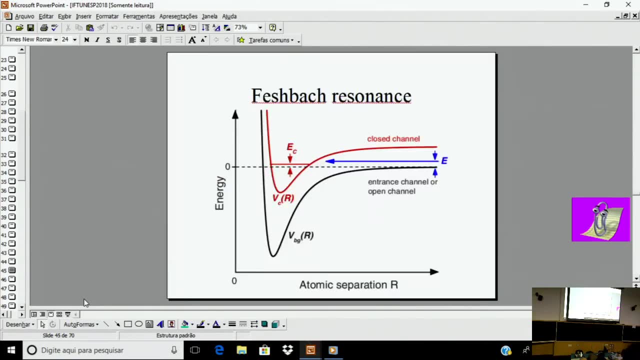 will be elongated in the direction of magnetic moment. We assume that the magnetic moments are polarized. Now the last thing I will mention is the phase back resonance. phase Phase back resonance is taken from nuclear physics. So phase back told the following: 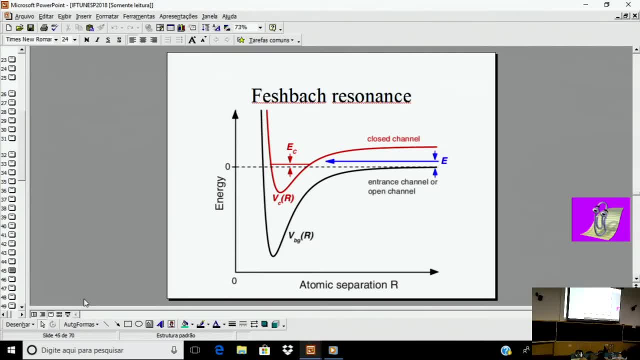 Suppose you are doing experiment in a system and this is the potential it sees: nuclear reaction between two nucleus. So this is the potential it sees and in this case, this is the potential between two atoms: the black thing, and this is the close channel, the red: 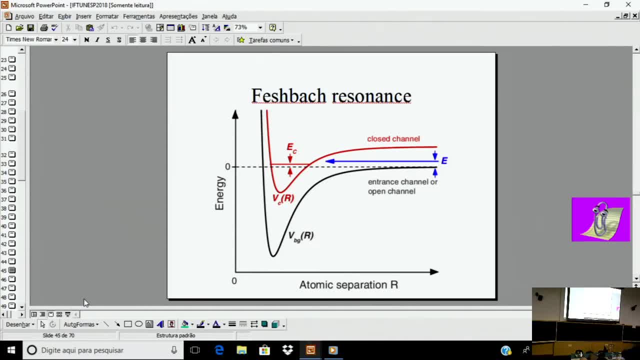 line. and if it is, so it and suppose there is a resonance in the red channel, the close channel. So what will happen? that if this resonance is close to the incident energy, then there will be resonance in the open channel. So this is what phase back told, but usually this is far away. suppose it is here. So this: 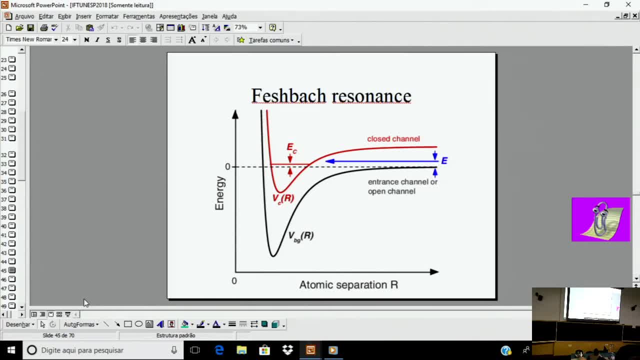 will not this. if the incident energy is this blue line, it will not feel this. but there is an ingenious way in atomic physics to change the effective interaction between the atoms. The way is the following: You take, make a Bose Einstein condensate of atoms which have 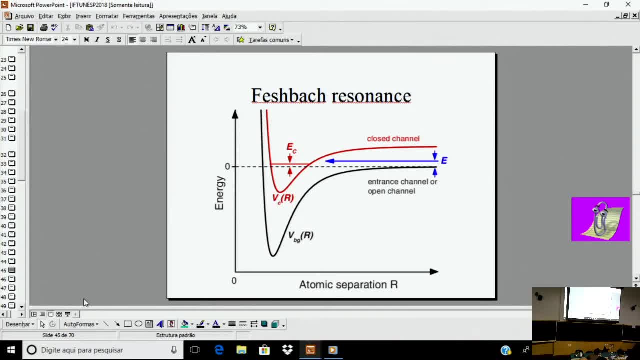 electronic spins Polarized. that means the all electronic spins are in one direction. but you can also make a system where the electronic spins of the of the two atoms are up and down. theoretically This system does not exist, but theoretically this system will be coupled to the other system. 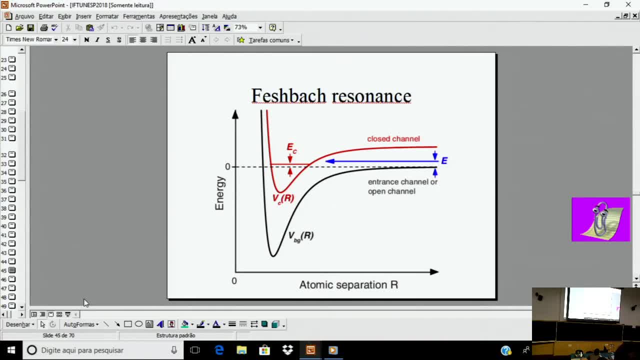 if you want to solve the dynamically the problem- and those are close channel, though this is not in laboratory, nowhere, but see what happens. you can suppose there is a resonance in the other channel. So if you can go change your energy then you can sit on the top of the. 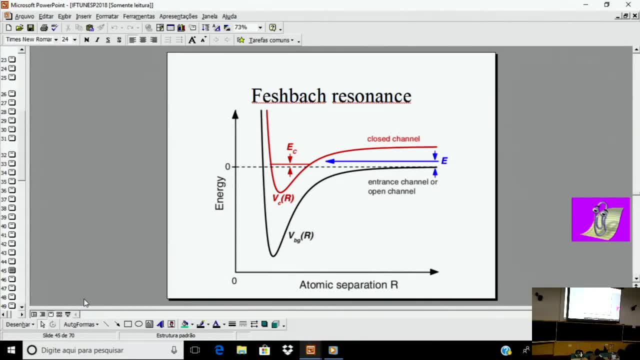 resonance in the other channel. So suppose the bound state or resonance in spin up, spin down system. because spin up, spin down always attract but spin parallel, they repel mostly. No a bound state, but these spin parallel system will feel this thing. how can you make them? 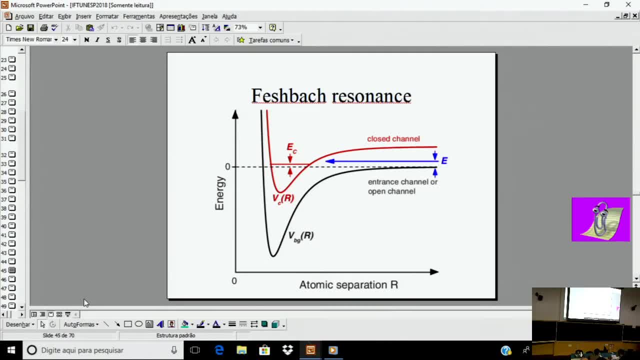 and make the spin parallel system feel8, you put an external magnetic field and increase it. If you put the external magnetic field, the open system which is spin parallel, it will accumulate magnetic energy. So each the energy will change, will go up and down. You can make it up, up, down and back. 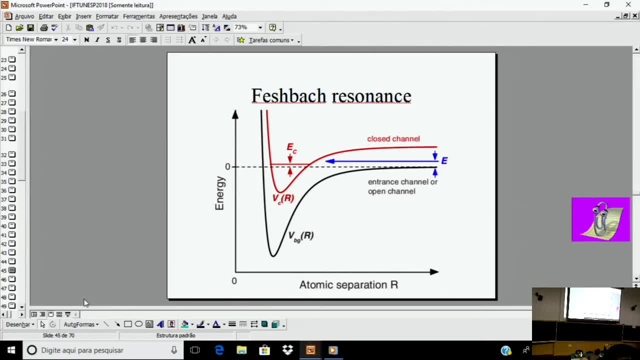 or down, So it can go on either side of the resonance. So if it is on top of the resonance the scattering length will become infinity. So you can make the system strongly interacting from weakly interacting by putting it in a external magnetic field. So this is phase. 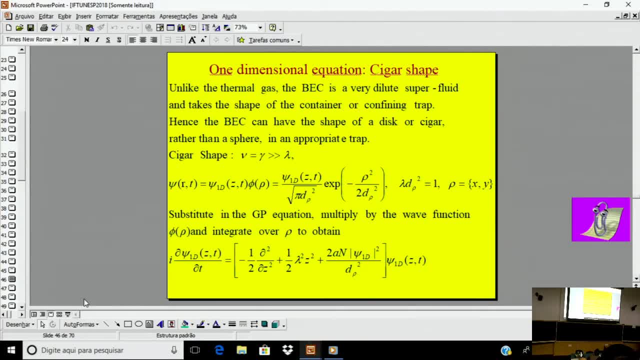 back resonance So you can make change the interaction between the atoms. So this is the crucial. When Feshback talked about this, he never had this idea. He died without knowing that it could be even possible to change the atomic or nuclear interaction. So now it. 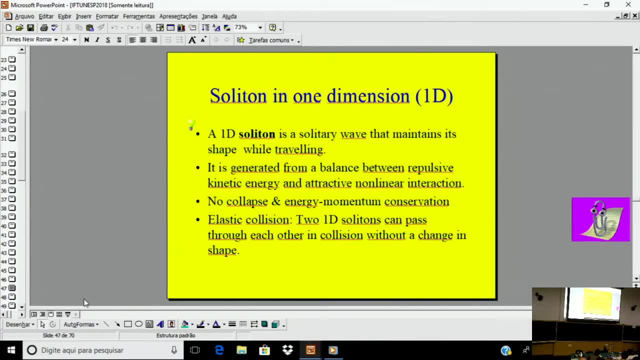 can be changed easily in the laboratory. Now we talk about soliton in one dimension. What is a soliton in one dimension? So one dimension of soliton is a solitary wave that maintains its shape while travelling. So this is a soliton in one dimension. It is generated from a balance between repulsive. 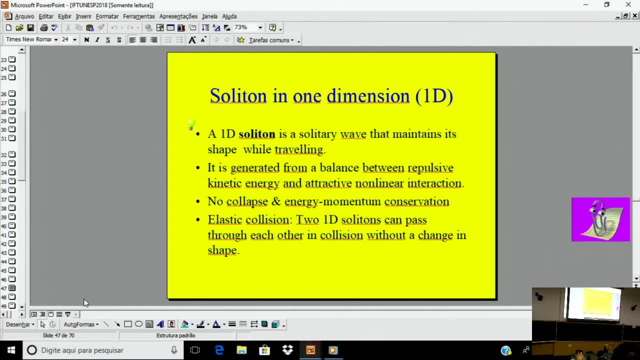 kinetic energy and attractive non-linear interaction. There is always a non-linear internal interaction, So there is no collapse and there is energy momentum conservation. I will talk about what is collapse, because if you have an attractive system, it can collapse, But in one dimension. 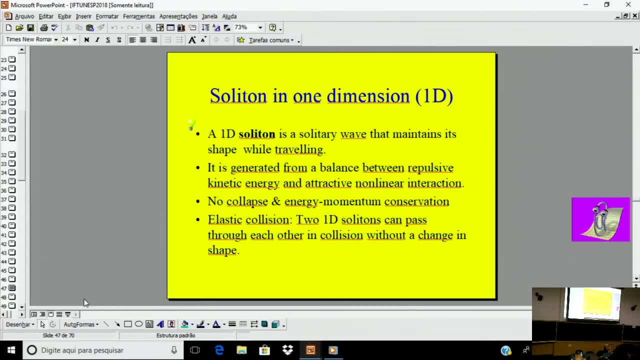 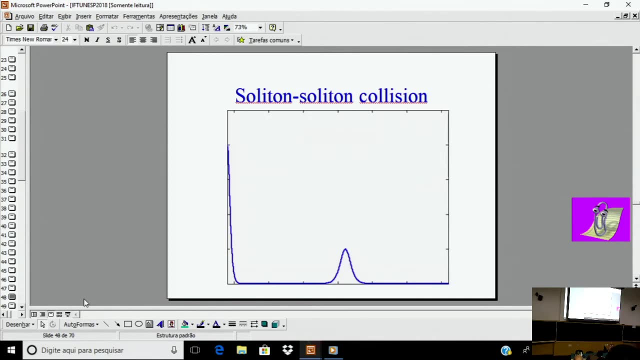 there is no collapse, So you can have elastic collision and because of energy- momentum is- and conservation, two 1D solitons can pass through each other in collision without a change in shape, like this. This is the wave: the two solitons crosses the other one without shape. 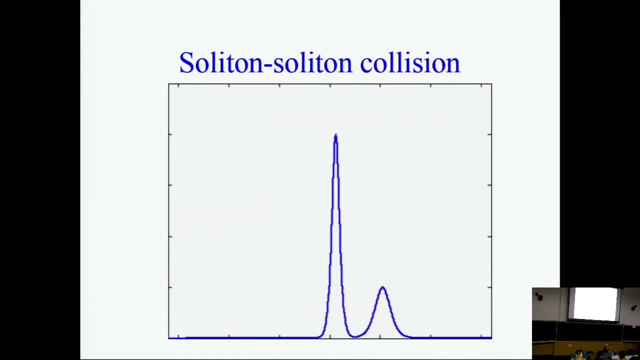 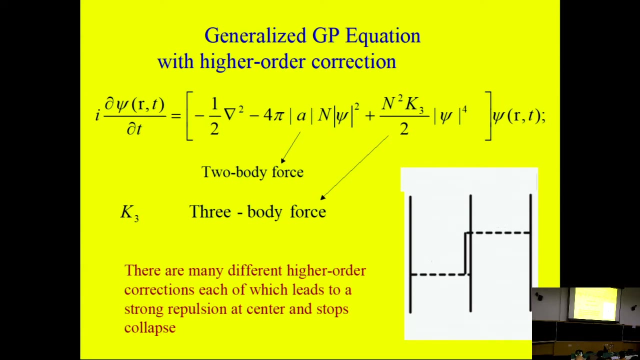 Now the question is: is it possible to have such a soliton in 2D and 3D? It is not possible, but you can have something very similar. So you write the generalized G-P equation. So so long the equation had these two terms, you will have obviously higher order terms. 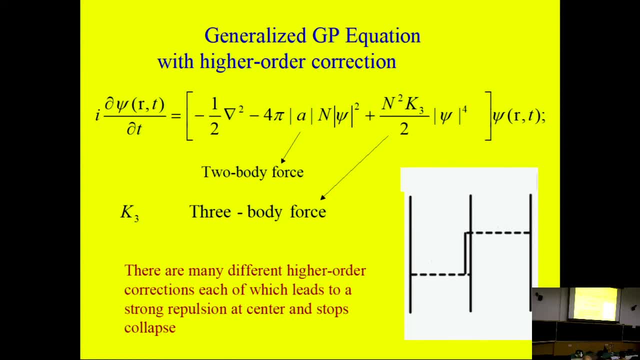 The easiest term that we can imagine is comes from the three body interaction. So three body interaction will couple the wave function of three particles, three atoms, Like two body wave function coupled the wave function of two atoms. that is why it was psi square. it was psi square. Now this will couple three and this will it will be psi. 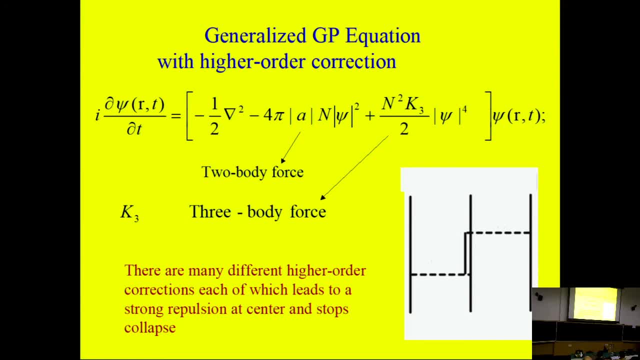 4 and k 3 is the three body force, So this is not a repetition of the two body force, because here this double line means that this atom is in an excited state. This is Feynman type diagram, So there are many different higher order corrections, like if you make a perturbation. 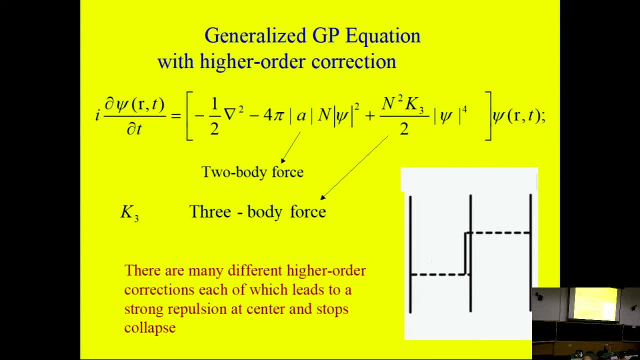 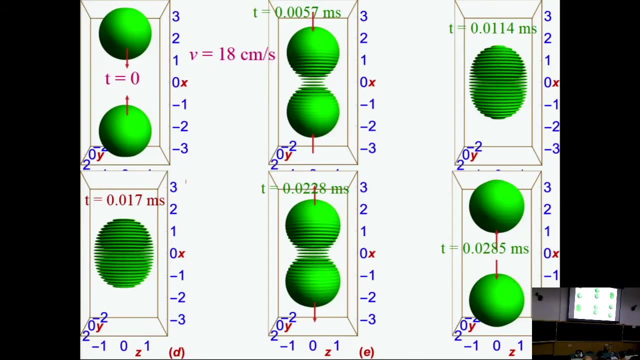 theory, there are many higher order terms and which, each of which leads to strong repulsion and center and stops collapse. So higher order term, and if it is positive, it will mean repulsion at the center. So the higher order term and if it is positive, it will. 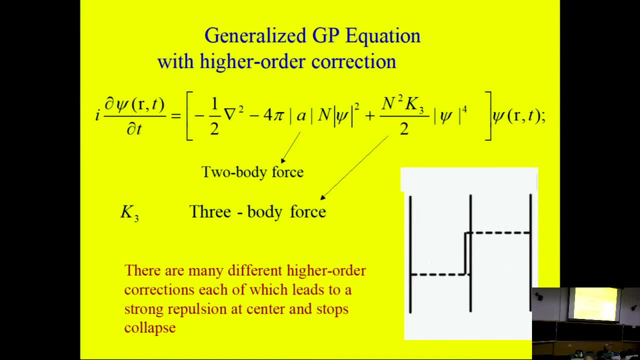 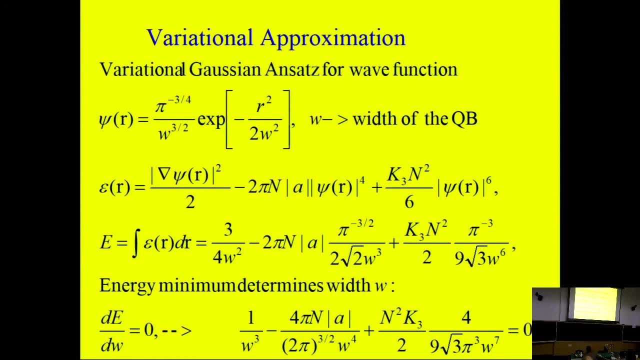 store, it will produz and volume С. So what about? H is typical, and how does H function, look like at high temperature? Let us say say at low temperature of 5 digamos in image here, where this will decides the valores here. So ø is equal to minus a fullhta. 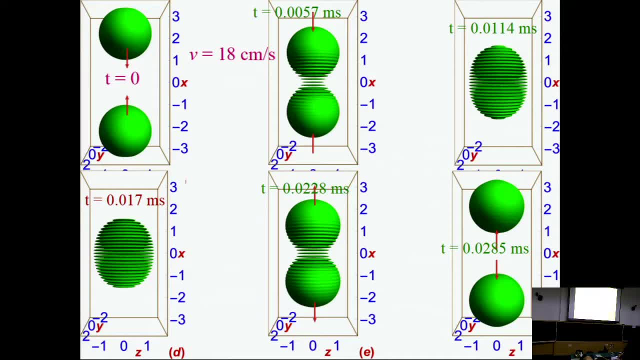 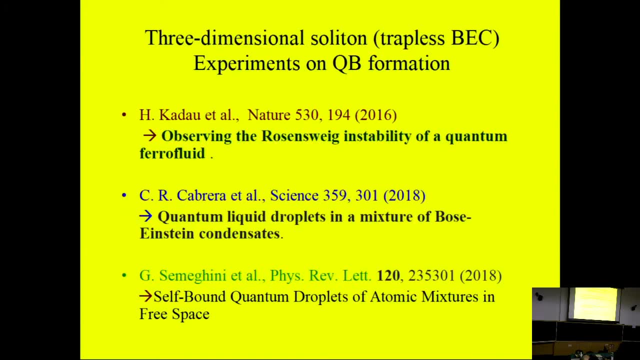 or V is equal to minus 2.. The domain around finish value: same way by name. you know what is V solution to extract the number from that V function. So now I am, I am present. here is the V function to extract. 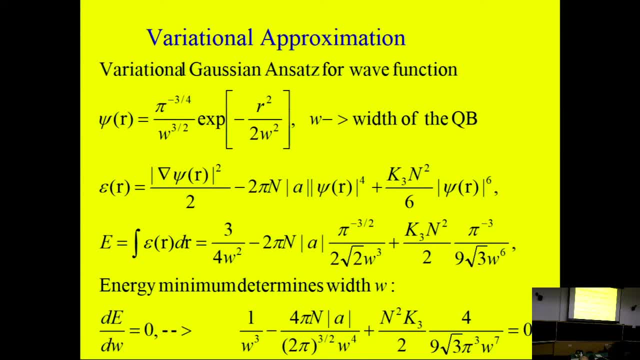 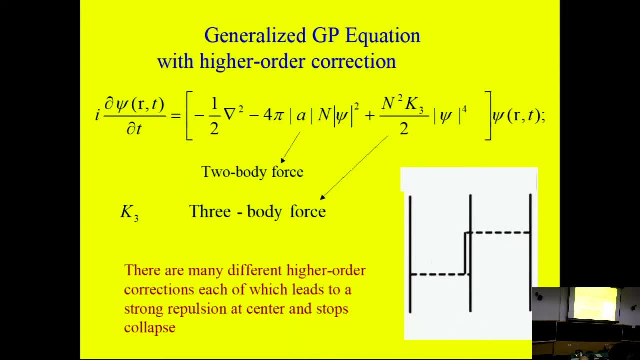 so I am like an equation. I am such a using, Leo. This is the kinetic energy term. This is half of the last term this term, because this is twice this chemical potential. So this will be half and this will be one-third something. 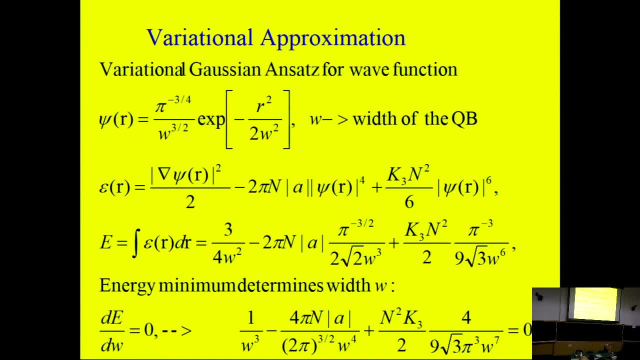 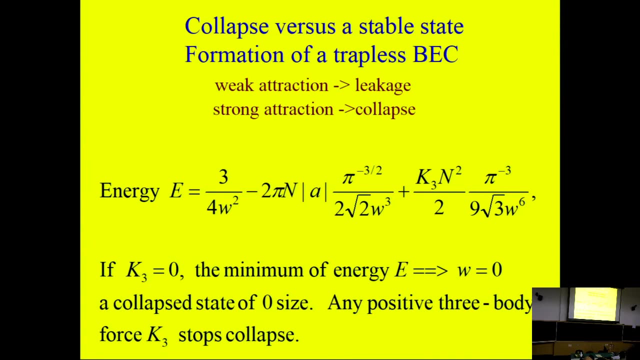 like this And you can calculate the energy, known the wave function. you can calculate the energy and you can minimize the energy and that gives the width. So you can easily calculate the width And how can you see that it stops collapse. This is the total energy. 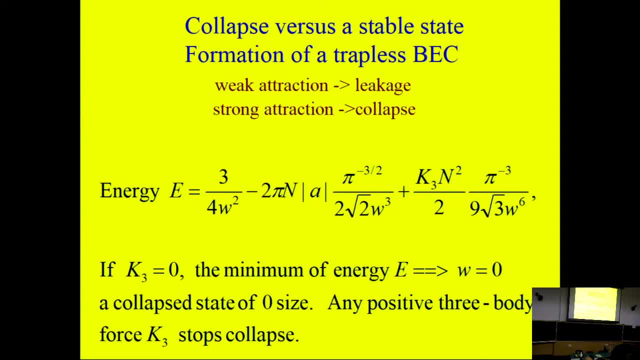 You see, this is total energy. W is the width of the Gaussian if there is a bound state. So if K 3 were 0, the volume of energy E is always at omega equal to 0.. So 0 means. 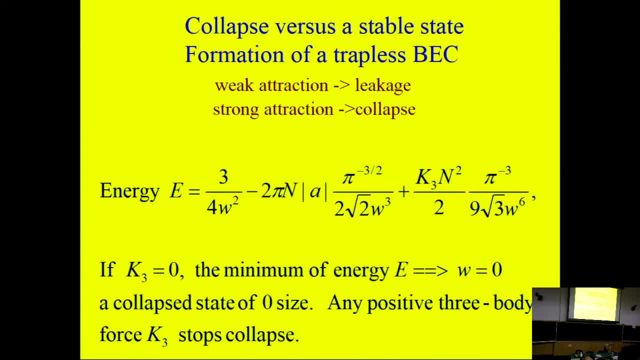 a state of 0 size. that means collapse state. But any positive K 3, you see in this case will make the energy infinity at for omega equal to 0. So collapse is avoided. But now you go to one dimension. This term will remain the same, but this term will be 1 by W. So 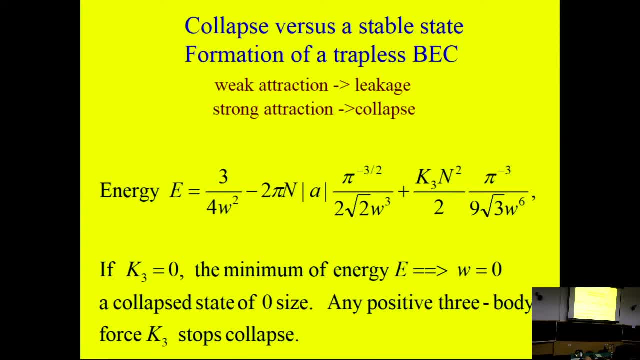 there is no collapse. And two dimension: the collapse starts. This is three dimension. This will be W square, So collapse will start, But in one dimension the energy at zero is really plus infinity, So there is no collapse. So now you see, you can have if the attraction is very strong. 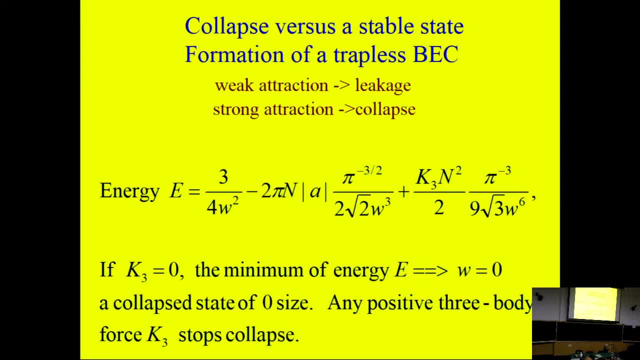 you can have a bound state If the attraction is weak- suppose this term is not there. so then the stable state is double equal to infinity. That minimizes the energy. So the weak attraction, the leakage, it goes to infinity. and strong attraction, it can have collapse. 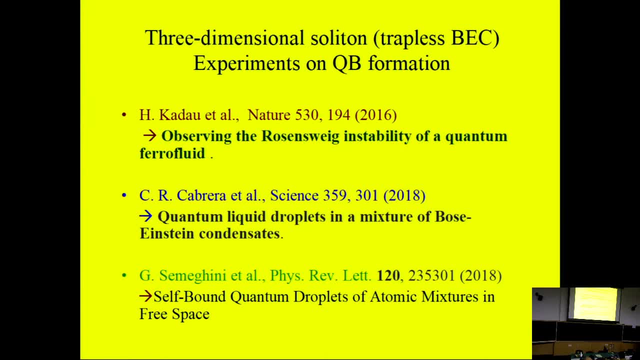 Now there are three. In search of this, I'll pass to 10 minutes, 5-10 minutes, Some quantum bound state formation without trap. So there is a paper in Nature in 2016.. They observed bound states in dipolar condensates. 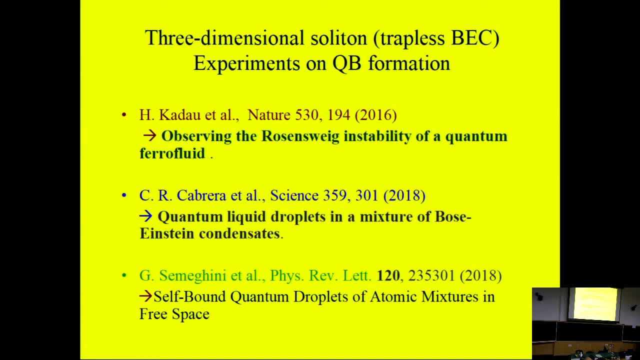 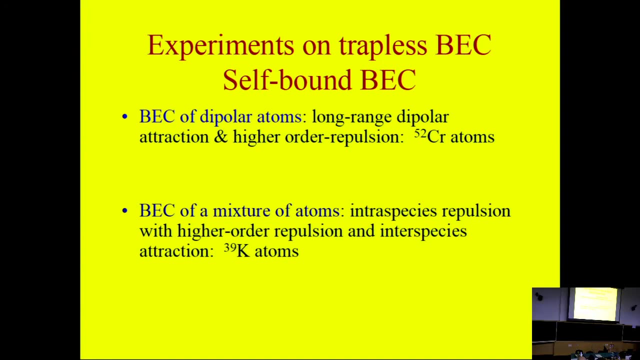 And these two observed bound states in this is in science in 2018.. Bound states of mixture of Bose-Einstein condensates- all without trap. The first experiment is on chromium: atom of dipolar things- A long-range dipolar attraction, and then you put a higher-order replacement. 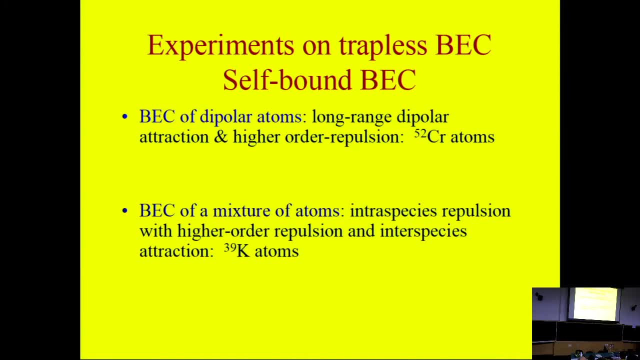 You put a higher-order repulsion to stop the collapse And then you make a mixture of Bose-Einstein. You take inter-species repulsion with higher-order repulsion. So this stops the collapse and there is the attraction between two species, two types of atoms. 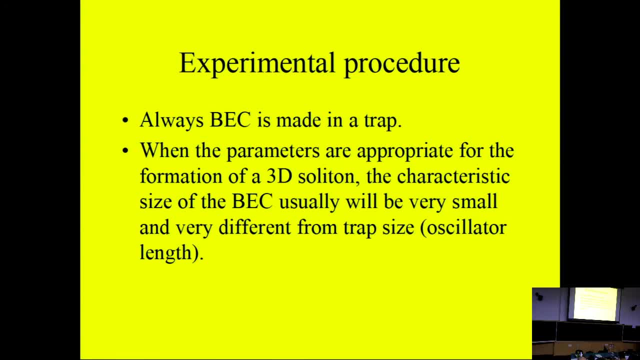 So experimental procedures always. Bose-Einstein is made in a trap When the parameters are appropriate for the formation of its 3D soliton. the characteristic size of Bose-Einstein usually will be very small And very different from the trap size, the oscillator length. 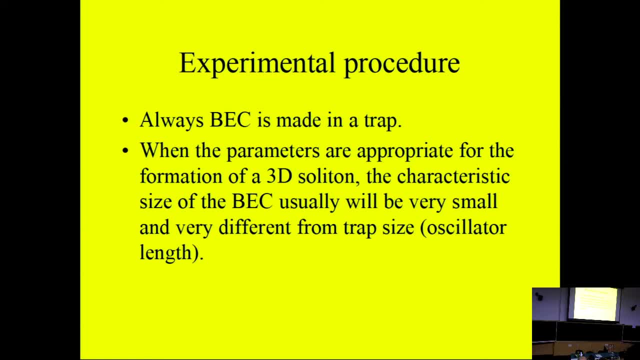 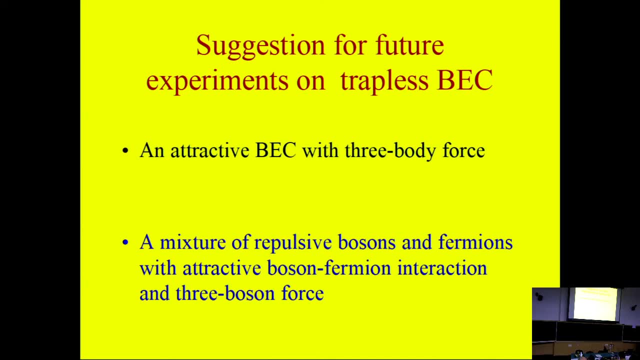 So it collapses but cannot collapse. So this is the self-bound state three-dimensional soliton. So suggestion for we have made some suggestion for future experiments on trap-less BEC. First is one attractive BEC with three-body force. 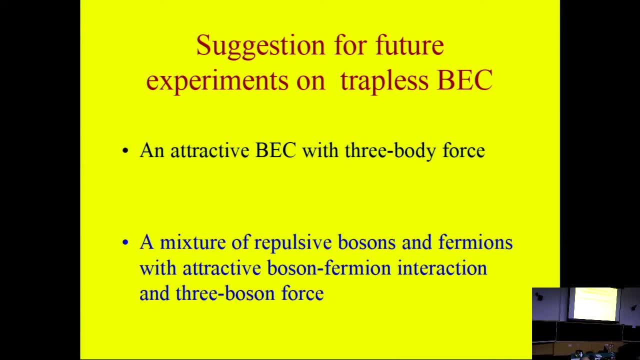 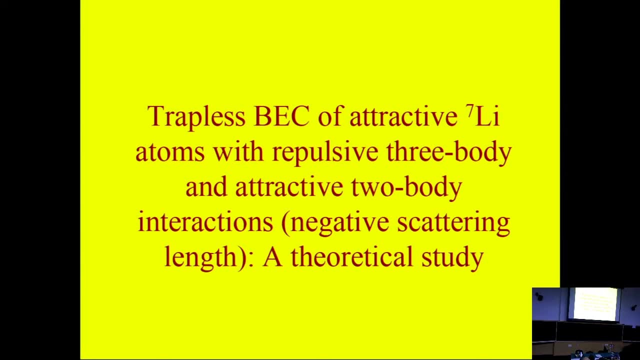 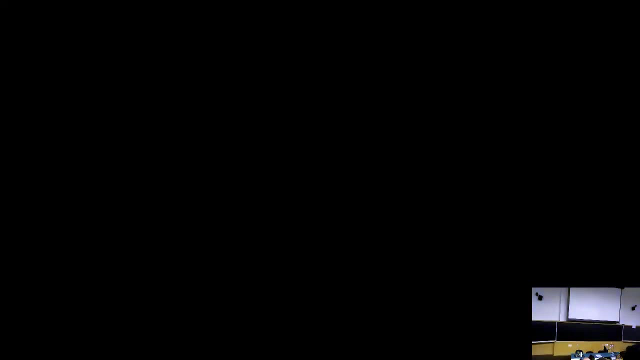 And second is the mixture of bosons and fermions which can also form bound state, So trap-less BEC of attractive lithium atoms, repulsive three-body and attractive two-body interactions, negative scattering length. This is theoretical study. So this is the equation: we had: the two-body force and three-body force. 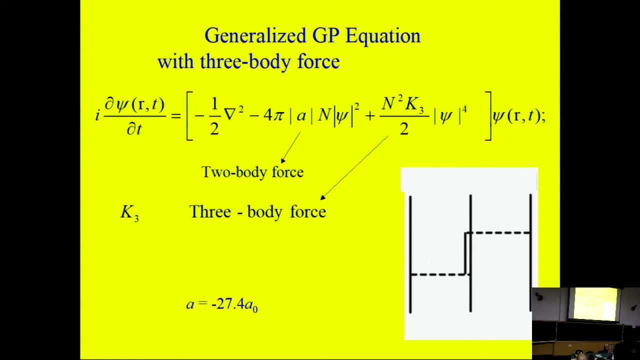 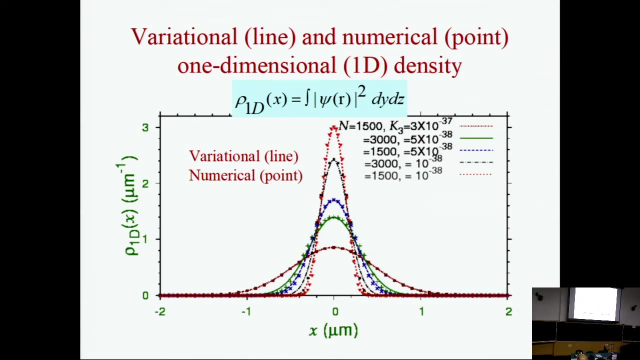 We take the scattering length of 27.4 angstroms. This is the experimental value of scattering length. So these atoms are attractive. lithium: 7 atoms, And this is the three-body force. We put a three-body force. So then we solve that equation for certain number of atoms and certain value of three-body force by numerical and variational procedure. 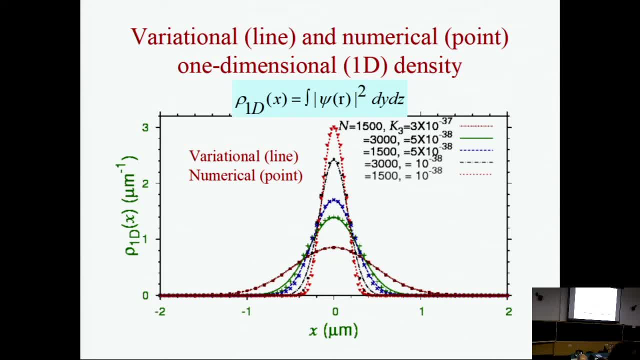 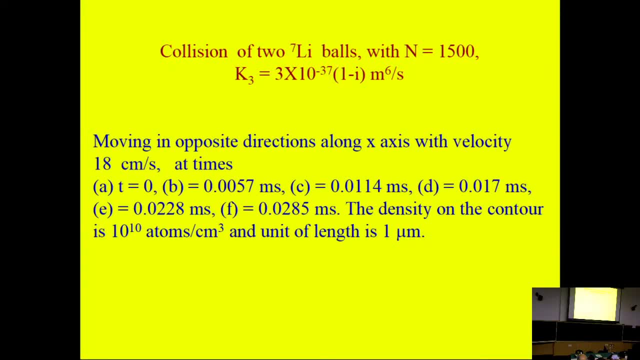 And they agree, And so we are more or less sure a bound state can be formed, a soliton can be formed. Then collision of two lithium balls, So whether they really act like solitons. So we take two balls which are formed with 1500 atoms. 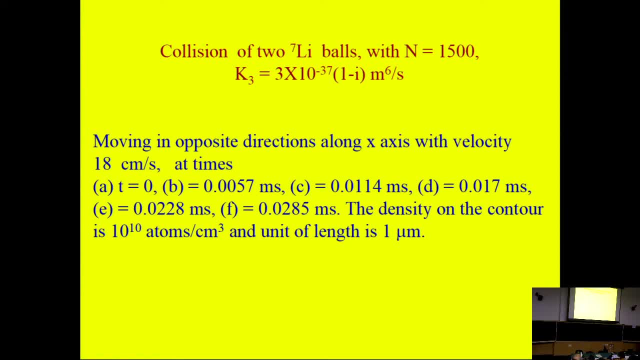 And K3 is this: I put this imaginary part there. This is the value of the three-body force, Because three-body force it is a three-body T matrix And it has real and imaginary part. So I also included the imaginary part. 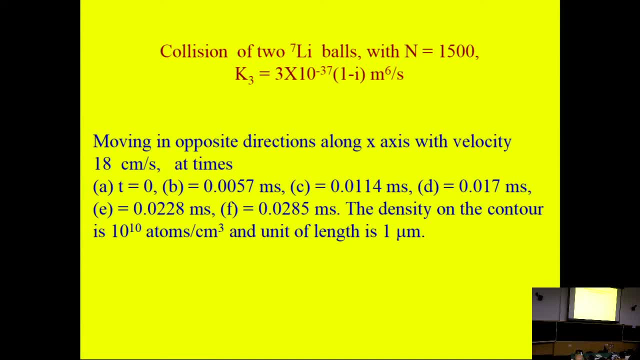 The two-body T matrix are zero energy. It becomes a real quantity which is scattering length, But three-body, continuous, complex. So we make them move, the two We consider, make two balls and make them move at a velocity of 18 centimeters per second. 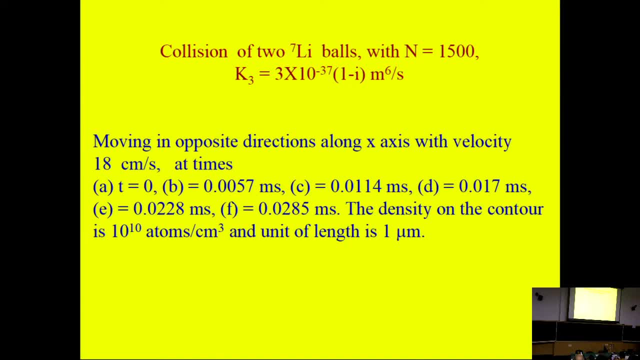 And we watch them at times 0. This many millisecond, millisecond, millisecond, millisecond, And density of the contour will show in the figure is 1 micrometer. So these are the balls, Two balls made without trap. 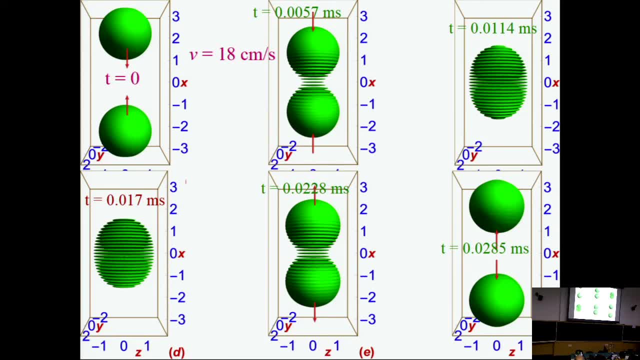 In that potential And they are moving with velocity 18 centimeters per second down and up. This is the first part And then it becomes here. So you see that in this way, in the middle case, there is interference pattern. 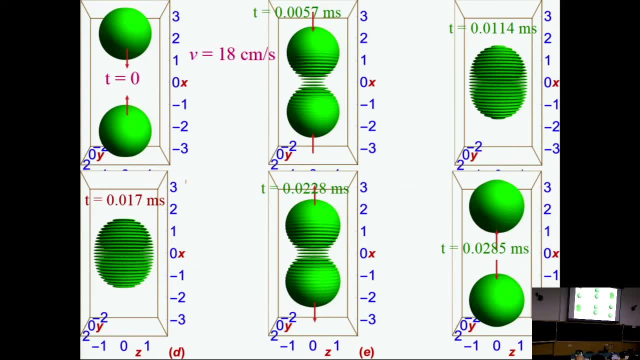 Because we put two balls identical balls there, So they are coherent states, So they form interference And then they separate. So they separate here. Last, And they are almost like soliton, There is not much distortion in these balls. 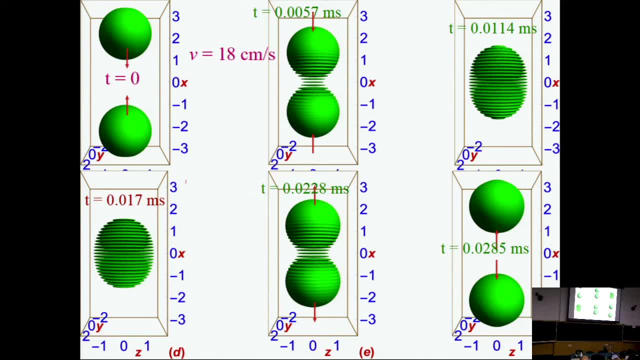 The velocity. I tell you. it's much larger than the velocity of sound. Sound is the velocity with which a disturbance will propagate inside the Bose-Einstein condensate. So 18 centimeters per second is larger than velocity of sound. 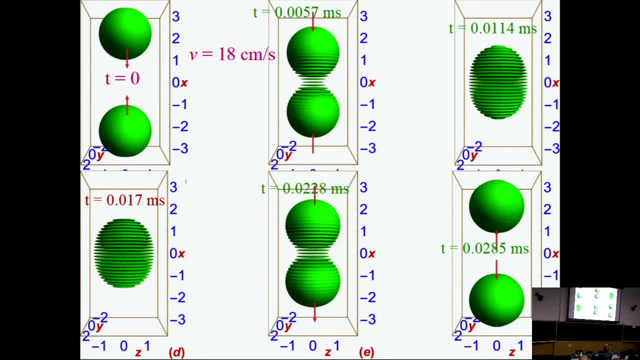 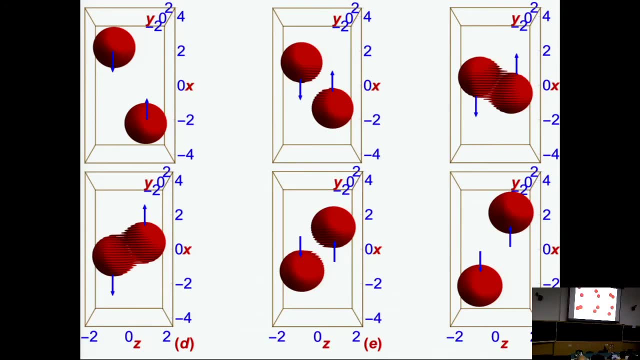 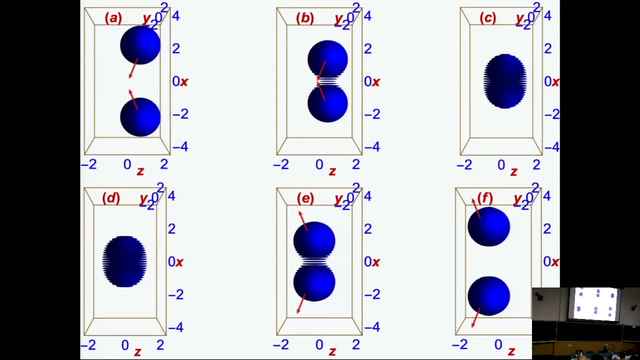 But it is smaller. There will be deformation, But in one-dimensional case there is no deformation. So now you have an impact parameter. They are separated. Even then, the same thing happens. They behave like soliton Or angular collision. 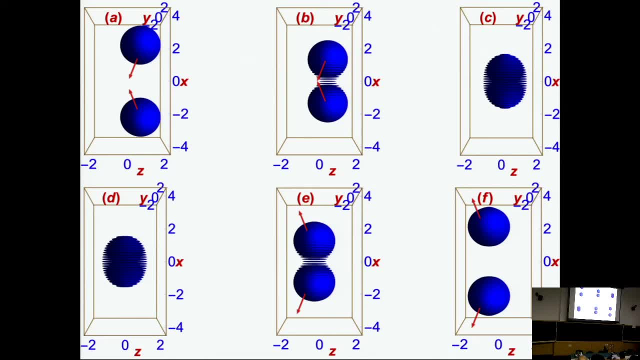 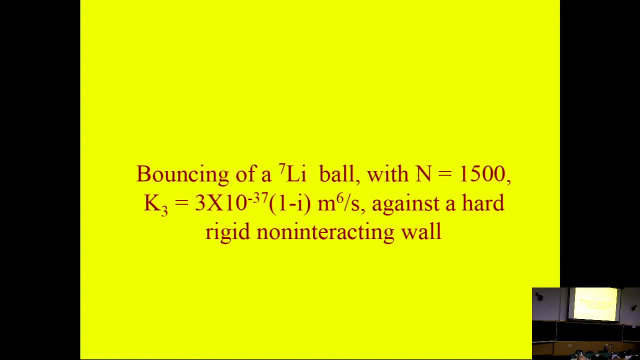 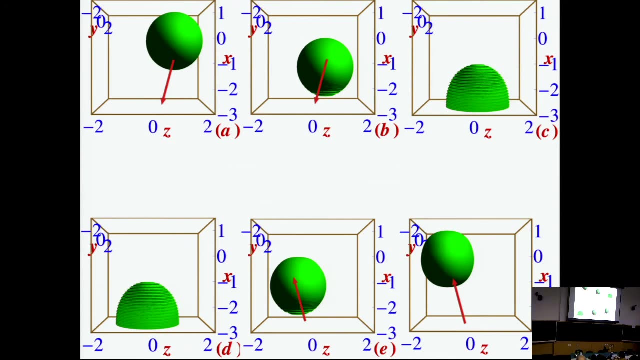 They come in angles And they separate out without distortion. So you can bounce a ball like this against a hard, rigid, non-interacting wall. So they come here, Hits here, And this is like this. And after some time it is like this: 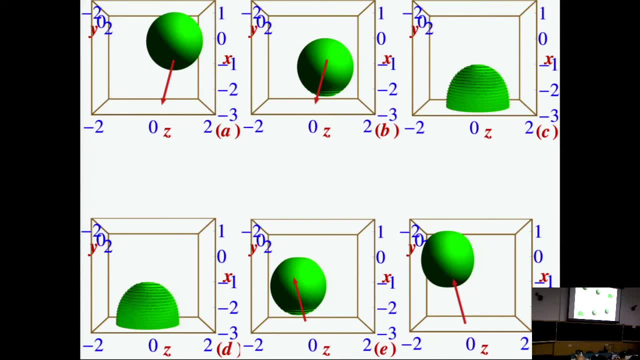 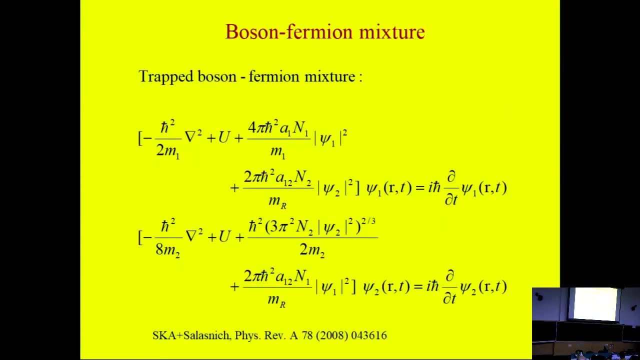 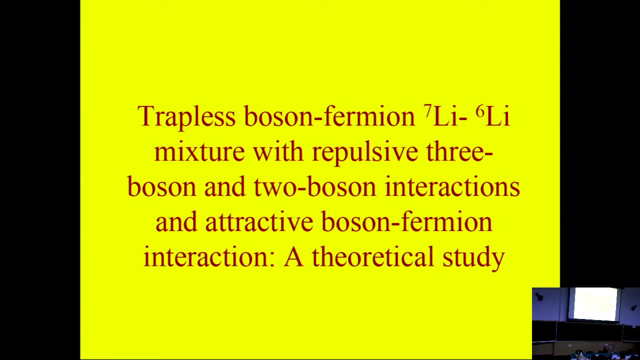 And then it comes out practically unchanged. So in the intermediate stage it was distorted here. So now we talk about another possibility: Deformation of bound state of lithium-6 and lithium-7 atoms. So we have the. So we have repulsive 3-boson and 2-boson interactions. 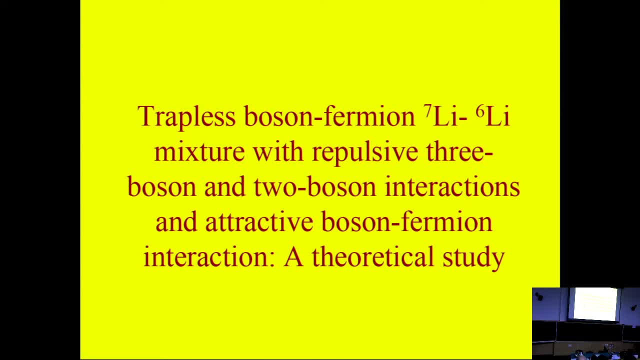 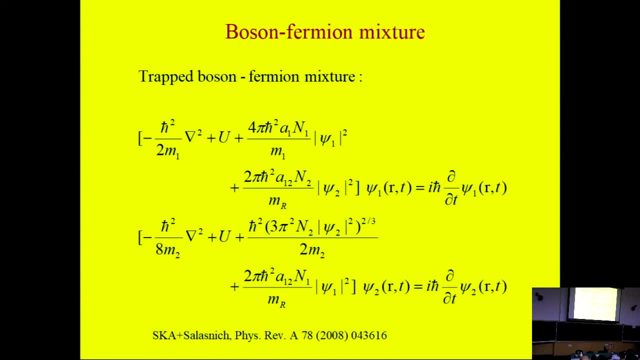 And attractive boson-fermion interaction. The fermions are by such non-interacting or repulsive. So the equation we have to modify. I will not go into details of the equation, But equation is modified. This was the previous equation. 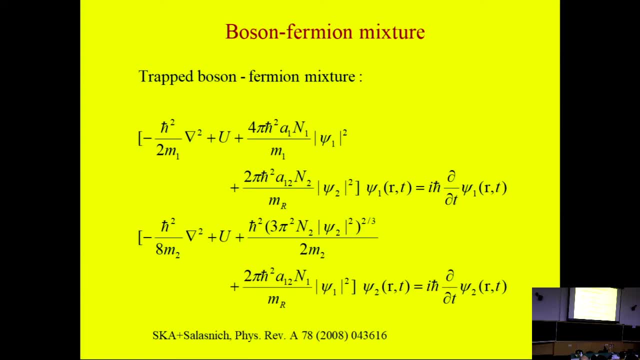 This term is the interaction between bosons and fermions. 1 is boson and 2 is fermion, And this is the fermionic equation And this is the interaction between fermion and boson. You have this equation And this is the fermionic energy of the atoms. 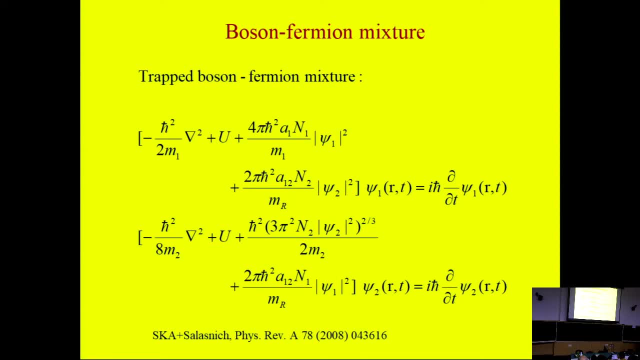 The kinetic energy of atoms. The fermions are arranged in different levels. So at 0 temperature they have this 0-point energy. It is less than Fermi energy. So if it is full up to Fermi energy So it will be n times some average energy. 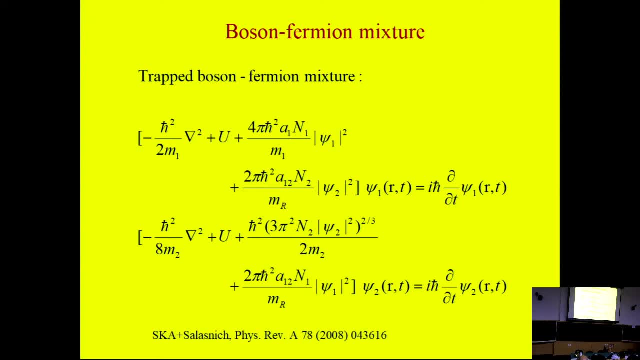 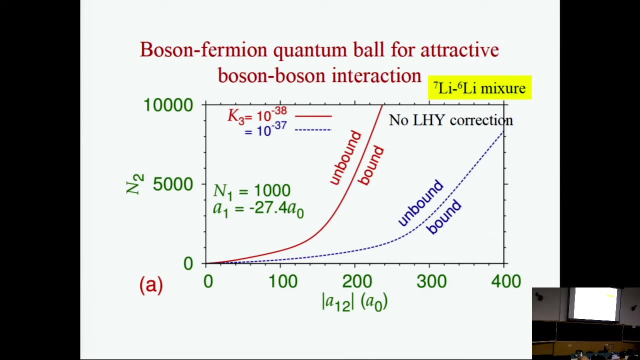 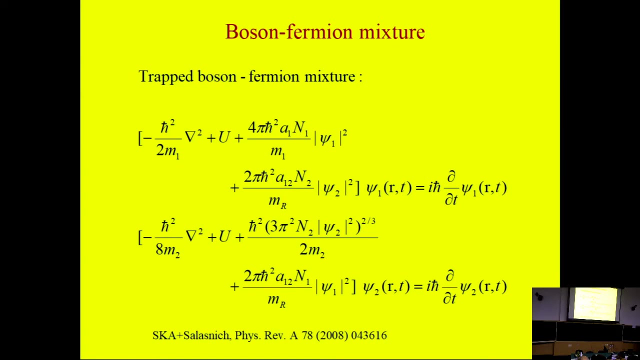 3-fifths, Fermi energy. So then you can show that they form bound states And there is some plots In this. I included the 3-body repulsion here To stop collapse. For fermion you don't need to include anything. 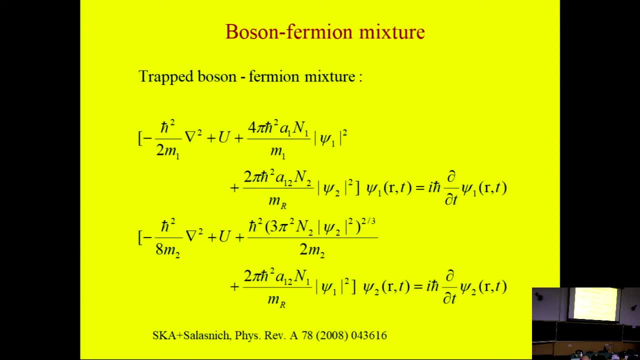 Because the whole thing is repulsive. So, bosons and fermions, they have attraction And this attraction is sufficient, Of course, if the whole system is at infinity. This attraction is not sufficient to bring them from infinity to 0.. 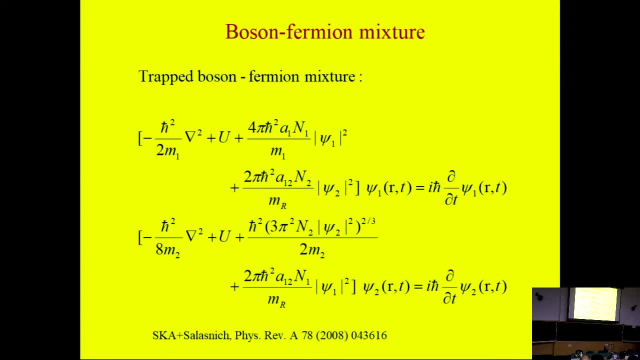 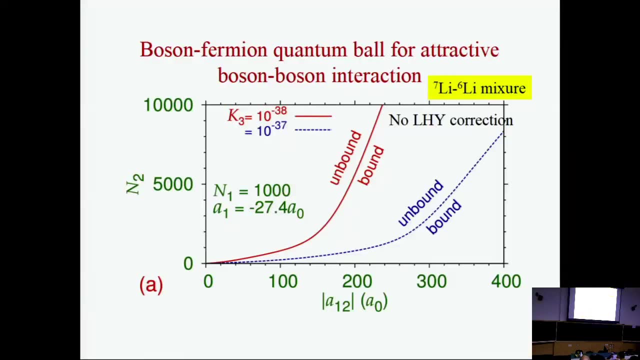 But if they are near origin, localized, Then this attraction is sufficient to form the bound states And they will not escape to infinity. There are some phase diagrams. This is the scattering length of the bosons. I took this. This is attractive. 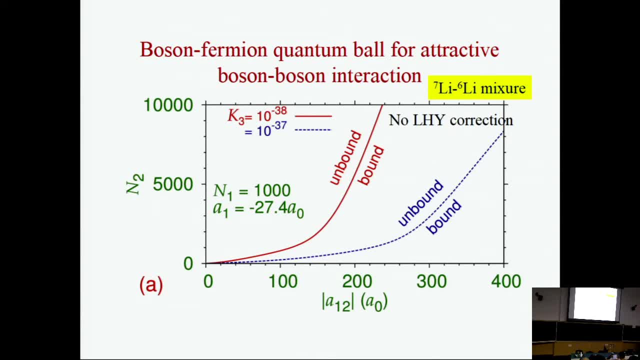 You can make it attractive the bosons, And still there is a region which is bound and unbound And we are changing this 3-body force. This is the number of atoms, Fermi atoms, The number of Bose atoms, And this is the bosonic scattering length. 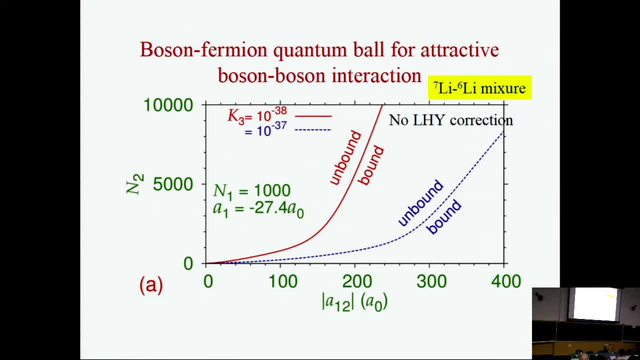 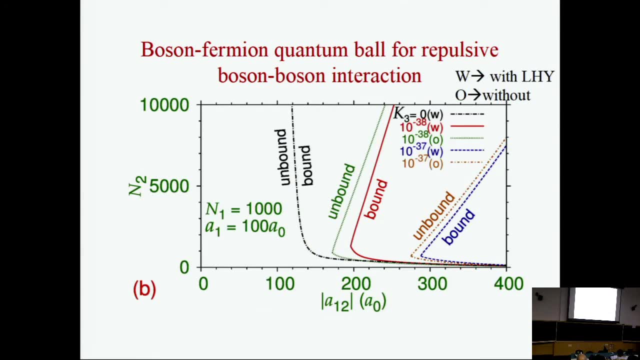 And this is the boson-fermion scattering length. So this is some region of bound and unbound, And now the repulsive boson-boson interaction And same number of atoms, And this is the boson-fermion scattering length. 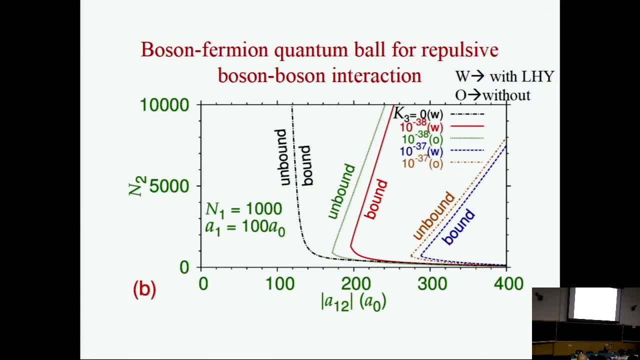 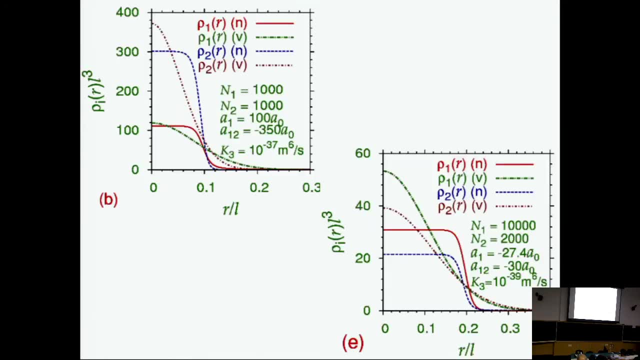 And this is number of fermions. So you have bound and unbound regions Once you change The 3-body force And you can put the wave function. You can calculate the wave function in a specific case By variational and solving the integral equations. 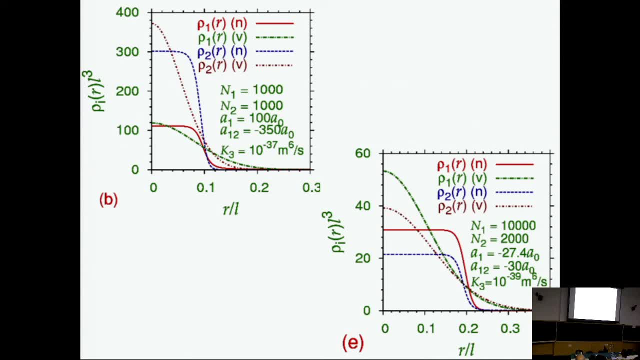 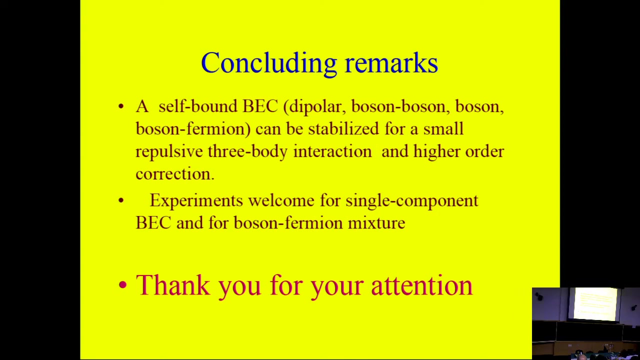 And they agree, Although the shapes are different. But there is agreement between variational and numerical calculation, Like this, This green one With this red one, So this gives some average. So the concluding remarks, So these things can be formed. 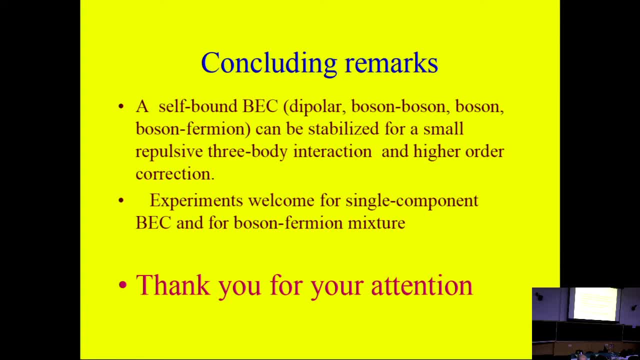 So experiments will come from single component, BEC, Which I talked about briefly, And for boson-fermion mixture, Whether they can form this 3-dimensional solid. Two others are already detected: Dipolar and boson-boson. 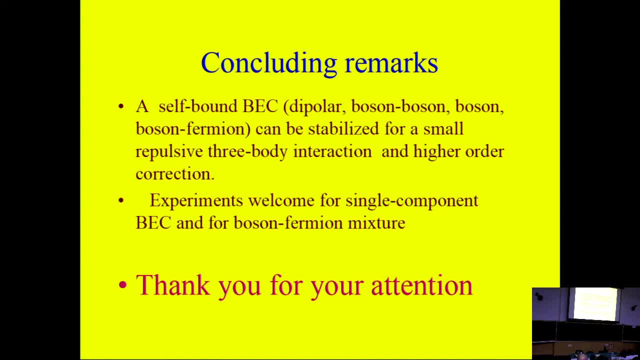 These are detected. So this Probably could be future experiments. So that's all, Thank you, Thank you. Thank you, Adhikari, So we have time for couple of questions. Yes, just a second. I did not understand about laser pooling. 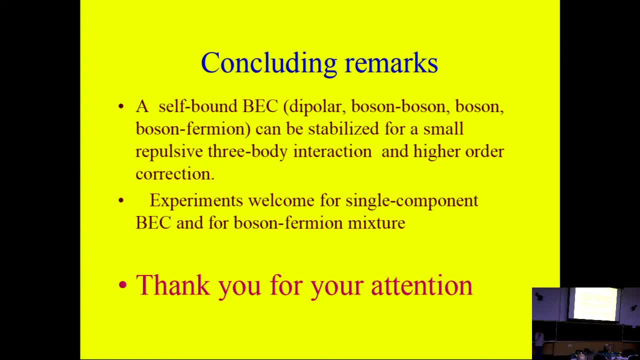 Can you explain again? Laser cooling? I'll tell: Take go Laser cooling, Laser cooling, That's just laser. Yeah, Yeah, Yeah, Yeah, Yeah. Well, I did not understand about laser cooling. Can you explain again? 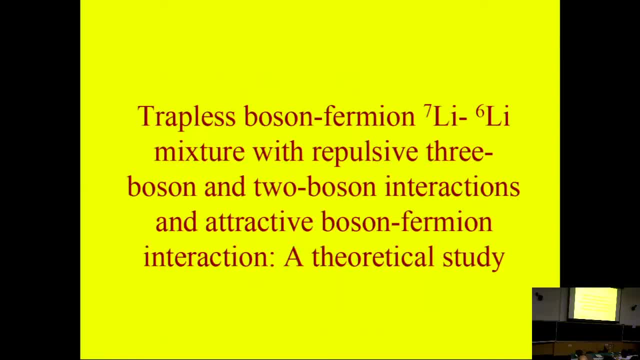 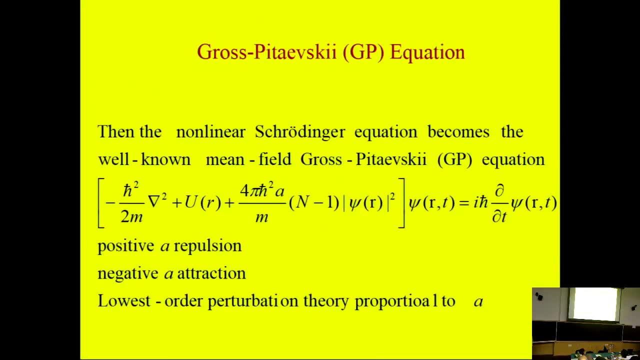 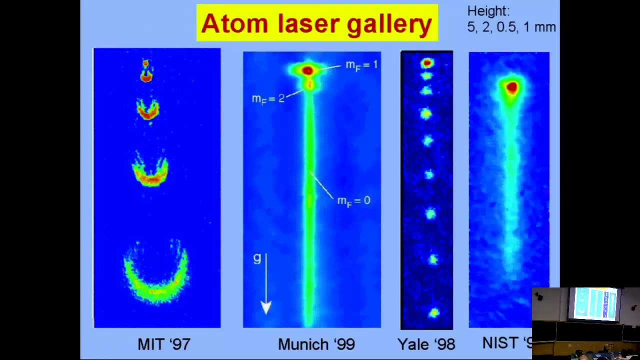 Laser cooling. I'll tell: Take, go. Okay, Let us go back. Any other question? No, I will go back. It is easy. The idea is very easy. It was done in 19.. So here is an oven and the atoms come in this direction. 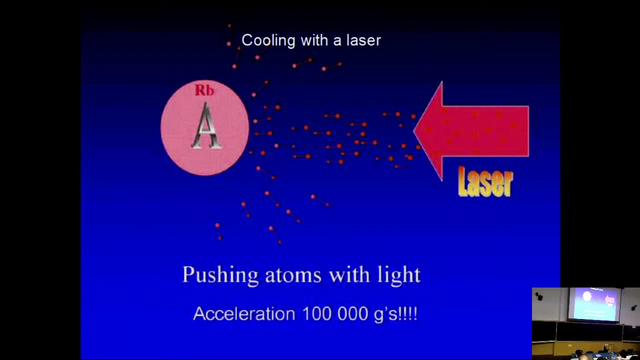 They come in ground state, Hydrogen atom in the ground state, And the most probable excitation in case of hydrogen atom is 1s2p, And this laser has energy equal to the 1s2p difference. So then the hydrogen atom will be excited to the 2p state, But with a lower moment. 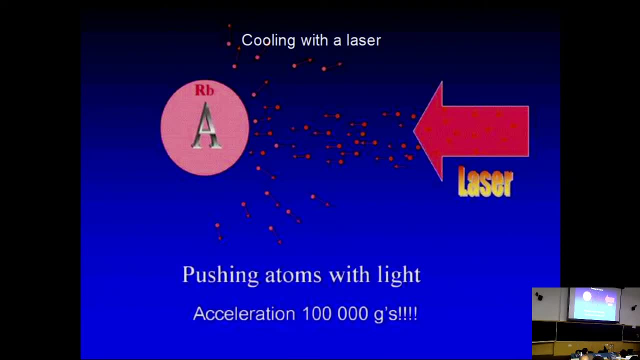 it will have less momentum. Why? Because it receives the momentum of the laser by momentum conservation. The laser is absorbed, So it absorbs some momentum. The velocity will be reduced. Why? Because it absorbs the momentum of the photon, But the question is: it emits. 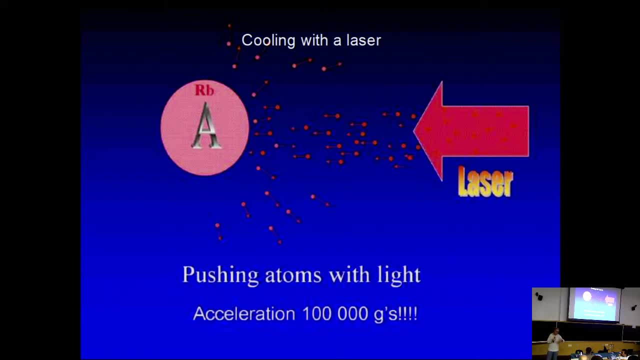 again the photon, It will emit again the photon, Then it has a kick again, But it can go in a In any direction. So some atoms will be lost, But some atoms will go in the forward direction. So you have to start with many, many atoms. Some atoms will be lost because 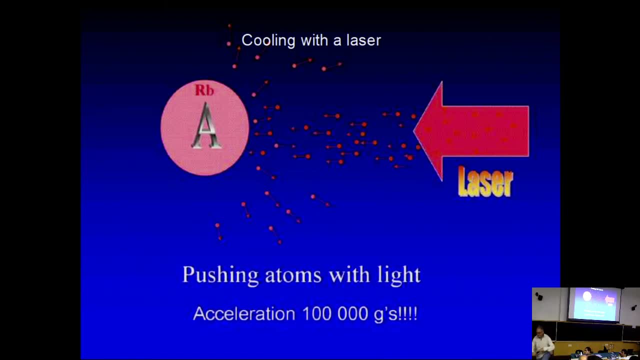 that will go in the wrong direction. But why it decreases velocity when it absorbs the photon? I do not understand. Photon has momentum. Photon is gone, So You have Doppler effect when you are approached to the photon. It sees the photon with another. 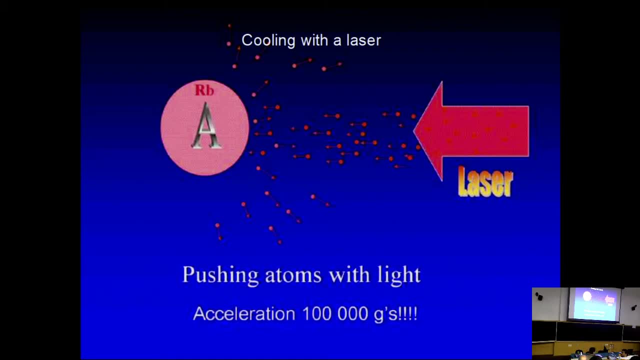 frequency Of the momentum of the photon, So it decreases when it goes toward to the photon And so, But how do I know that it moves? They are always pushed back Statistically. I think that the laser is likely between this frequency, such that the atoms 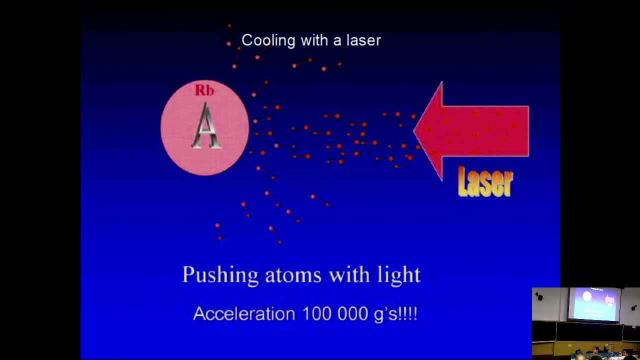 that come in the opposite direction receive the momentum. No, If you go into many details, because once the velocity is reduced the laser energy has to be adjusted. That is done by optical pumping. I did not go through it. So once the energy of the 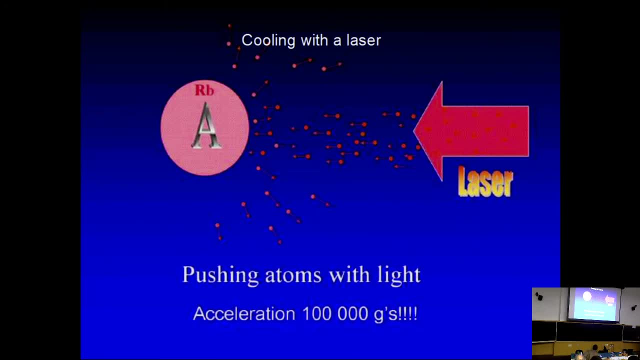 atom is reduced because of Doppler effect. you have to change the laser energy also. It is about Doppler effect. No, no, no, no. The momentum is reduced because it receives the momentum of the photon. I do not understand Why atoms moving towards the laser absorb photon and the atoms moving 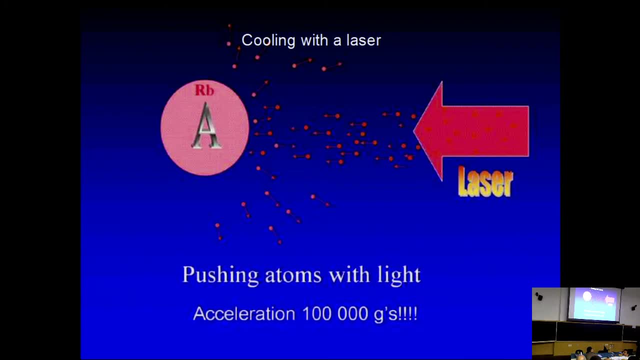 in the opposite direction? do not, Because if the atom moving in the opposite direction, then it also, I see, Because it receives the impact of the photon, And photon had a momentum and energy. It absorbed the energy, so it went to the excited state. It absorbed the momentum, so its velocity. 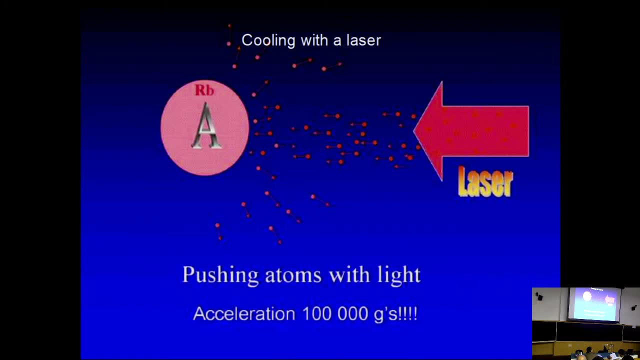 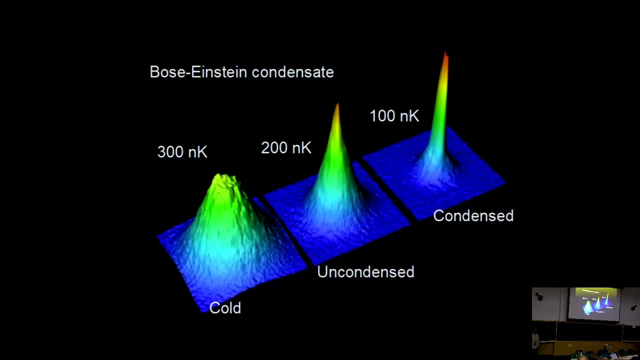 will be reduced. My question is: why do you need repulsive three-body potential? to stabilize, to avoid the collapse of your, Oh, repulsive three-body potential? You have to have repulsive three-body potential. You have to have repulsive Because otherwise the equation is two. 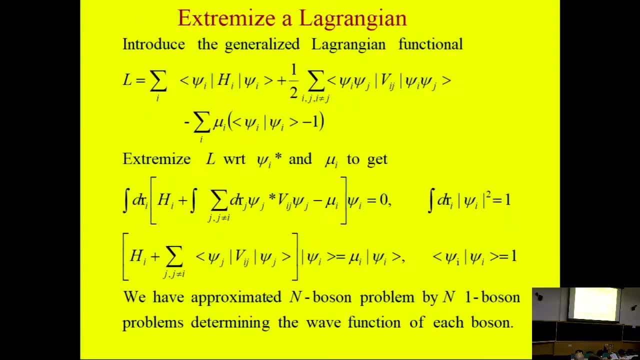 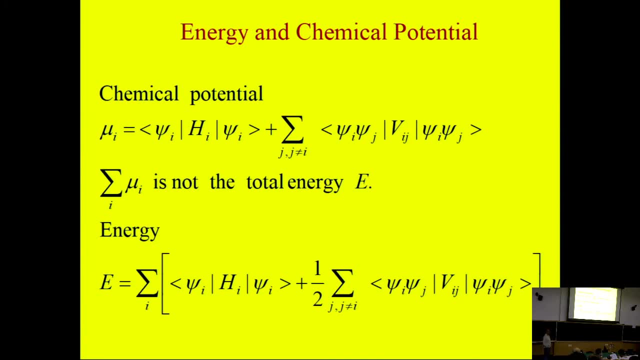 But in Let us go there, Because in principle, your two-body potential is already very repulsive at short distance. atomic potential, No, no. And in two We don't have the two-body potential. We don't have the two-body potential in this model. 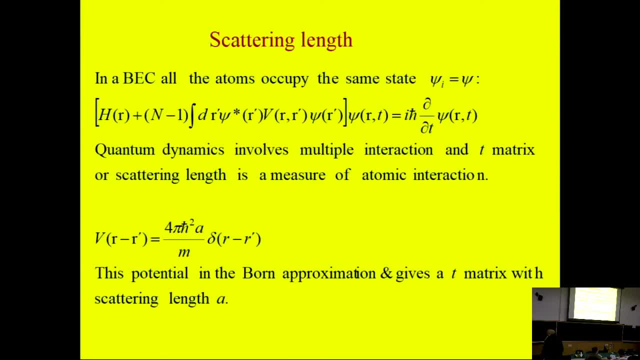 In this very weakly interacting limit Because two-body potential? I changed here Because two-body potential is very repulsive at the center. That is true, But it does not see the two-body potential. It sees the effective potential, which is 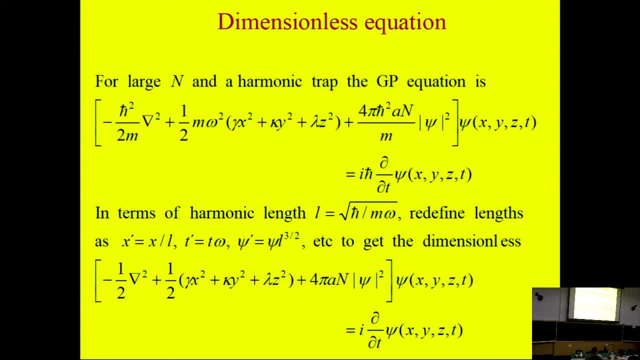 a sum of this series. This is two-body potential, So quantum mechanically it can interact as many times as you like. If two balls- classical ball comes, it will hit once and go away, But quantum mechanically it will. You have to sum the whole series And this will become a T matrix. And as it is very 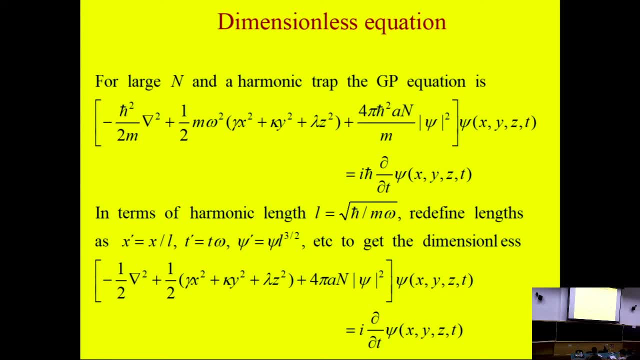 dilute and as they are separated it will see the T matrix. So the two-body potential could be Is always attractive at large distance and repulsive at short distance. But this scattering can be anything. It can be either plus or minus. If it is plus, the system is attractive. 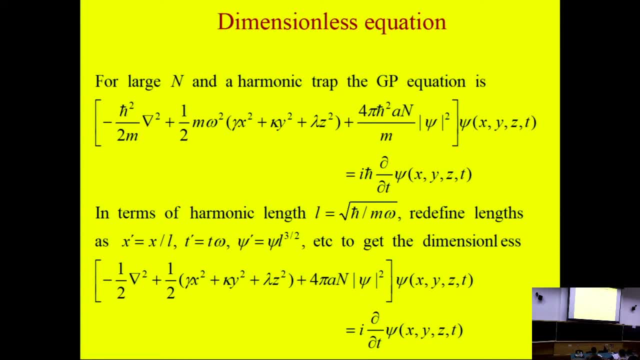 The Bose-Einstein will: No. no, If it is plus it is repulsive And if it is minus it is attractive. Sign, change, Sign of the potential change. Okay, But this is three-dimensional, This is three-dimensional equation. 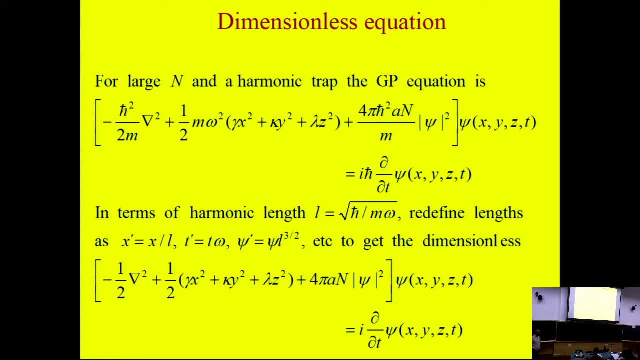 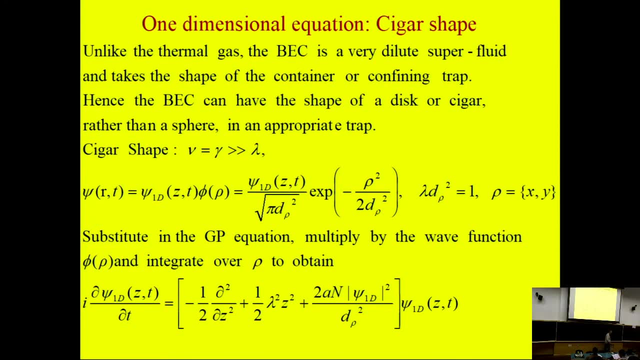 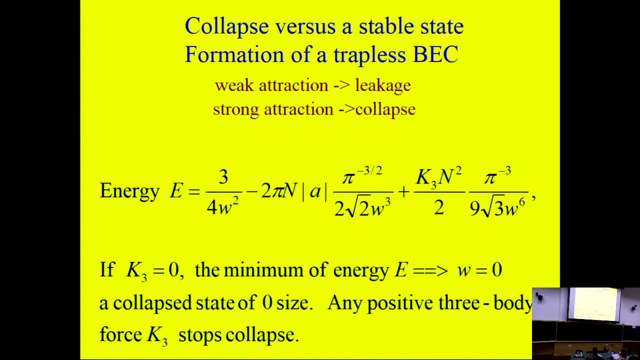 But in two-dimensional you don't have such collapse, right? Two-dimension is limiting case It starts collapsing. I'll show you: I talked about This is the energy Suppose. you take out the three-body term. This is three-body term. 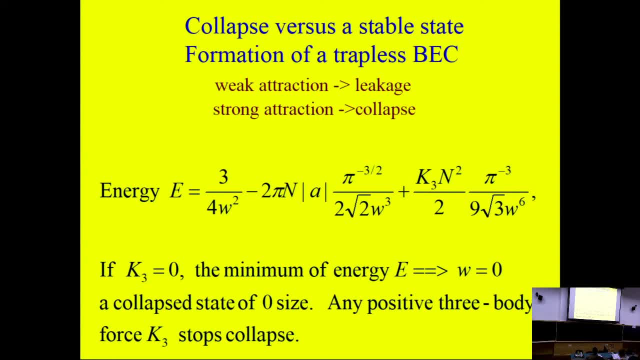 You have this And omega is the size of the bound state. You see that at 0,, if this is attractive, you have to have attraction because you have to have negative scattering length for binding. So at 0,, the energy is in. 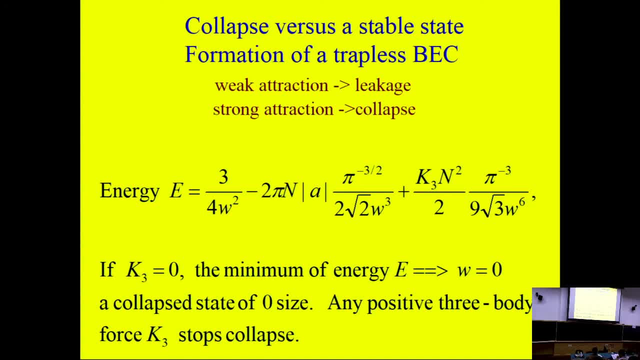 It is infinite, So the system will collapse. This is in two-dimension. Two-dimension it will be omega square, So it's the limiting case. It can be anything. This is 1 by W square, It is the kinetic energy And this will be also 1 by W square, So come. 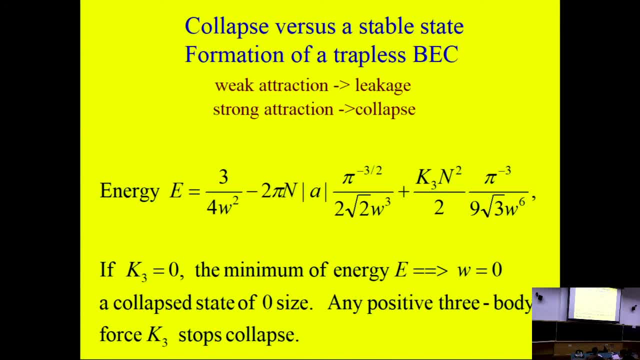 to one-dimension it will be 1 by W, So the attraction will not be strong enough to overpass the kinetic energy repulsion. So it cannot collapse. Just a short, Because, as you know, in two-dimension you don't have such collapsing, if you consider. 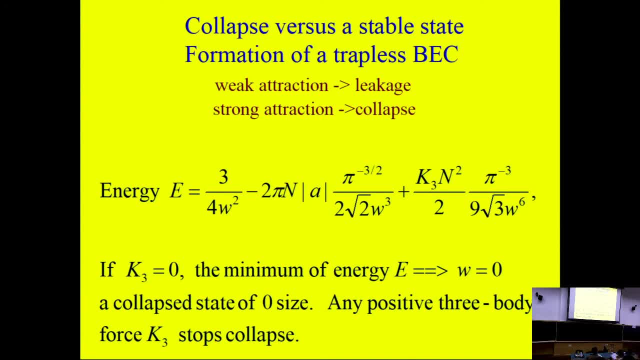 just three bosons. I know There is no collapse. OK, In two Limiting case. It's the limiting case And 2 plus epsilon dimension will start collapse. Eduardo has a question Why? So maybe you have kind of addressed my question already, but let me just make sure I understand. 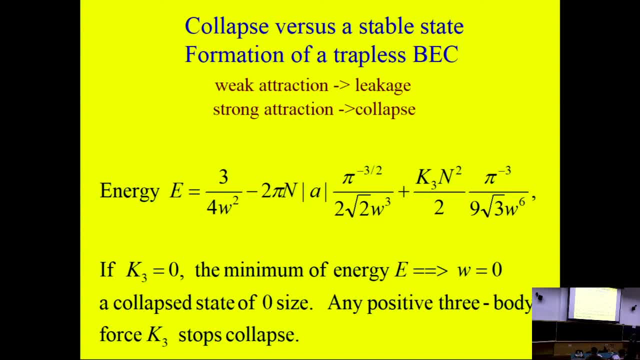 So it's connected to these 2 to 2 versus 3 body scattering terms. So for the first term. so you assume a very dilute system. So you replace by the function and so on. So naively one could imagine that the 3 to 3 scattering should be less important. 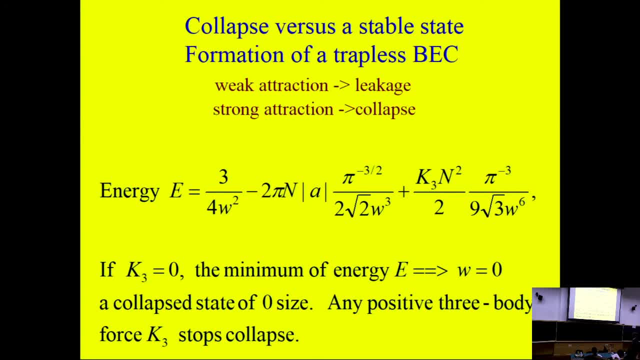 So I guess the fish diagram, the second diagram, it's a series, Yeah, but this is a series, Sorry, This is a series, Right. But so initially I was wondering about the consistency of the dilute approximation when this other term is playing an important role, clearly. 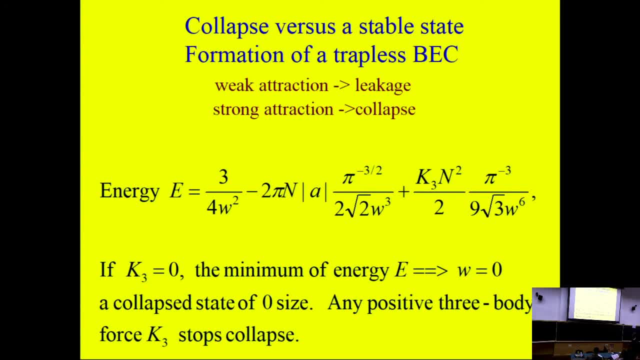 And the density increases. But OK, So the fish diagram- I thought for bosons at least- gave rise to a- Let's say it was a fit to the fourth theory- gave rise to an attractive force. Is that Here? 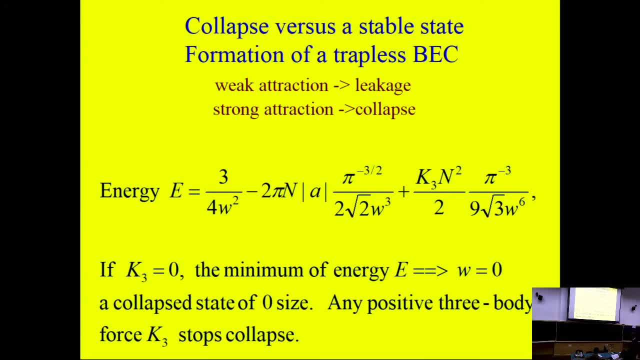 Here, I don't know Noted This gives the attractive force at large distance. The potential is attractive at large distance and repulsive at small distance. So it depends on the coupling, of course. But Yeah, Yeah, Yeah. 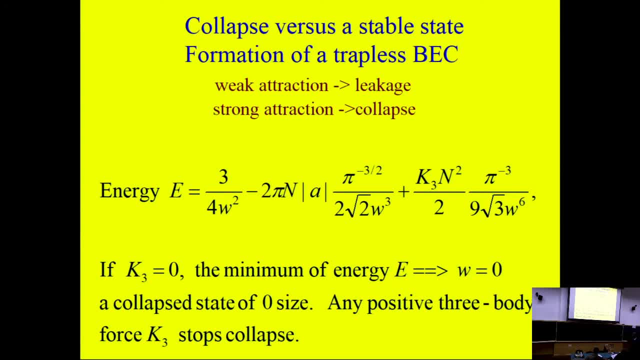 It depends on the coupling. Atomic potential is usually attractive at large distance and repulsive at short distance. For fit to the fourth, Huh, Nuclear potential also, OK. So for the fish diagram, For the fish diagram, what is the range of that? 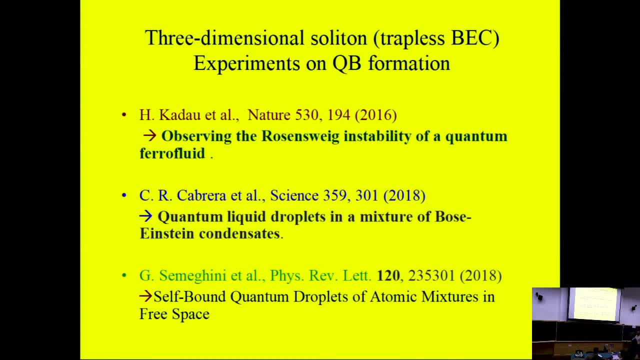 So is there an effective mass that enters into that? Not that one. This is the potential. The second- I'm talking about the second diagram- No, the second. The second. Yeah, Yes, So what is the? Is there some mass in those propagators that enters and controls the range of these? 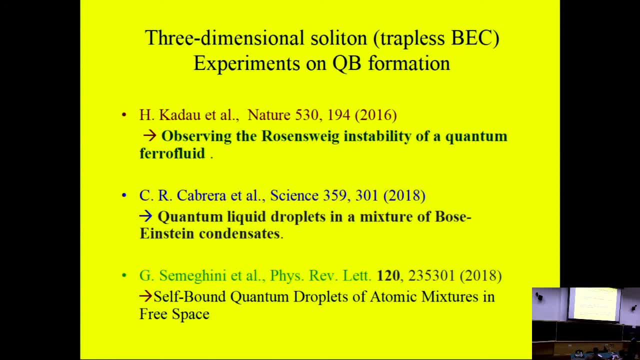 This is the same mass of these incident atoms. This is the scattering series. So how large is that range compared to the diluteness of the? I do not know, I did not compare What I know that if you increase the number of atoms, the density increases. and then this: 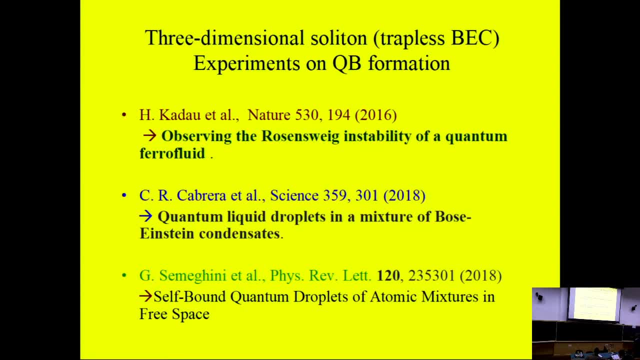 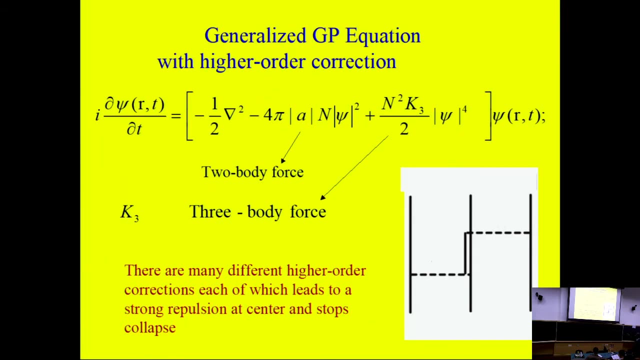 is not sufficient this term. The lowest order, approximation is sufficient, and this will come into picture. Little bit, little bit it will come into picture And this will break down. when A goes to infinity, Scattering goes to infinity, Then it's unitary. 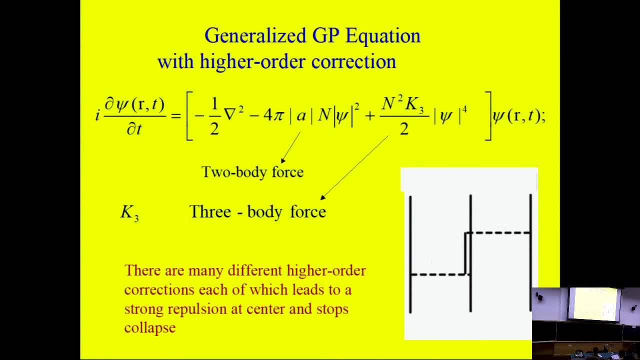 It is strongly interacting system, But it does not mean the energy is infinite. Many people think that if A goes to infinity, that means the energy of the system is infinite. That is not true. It's strongly interacting system. Okay, Now we continue. 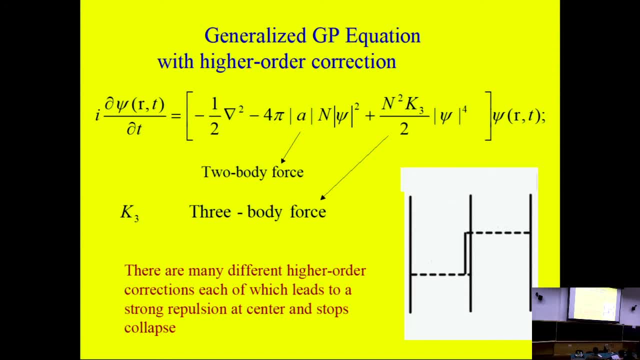 I'm just wondering. So you think that this truncation at this term is Gives a Gives a sufficiently accurate picture that if you go and look for these things experimentally, you will be able to see this solid? Yeah, I think when A is small and N is small, like N is few thousand and N is hundred million, 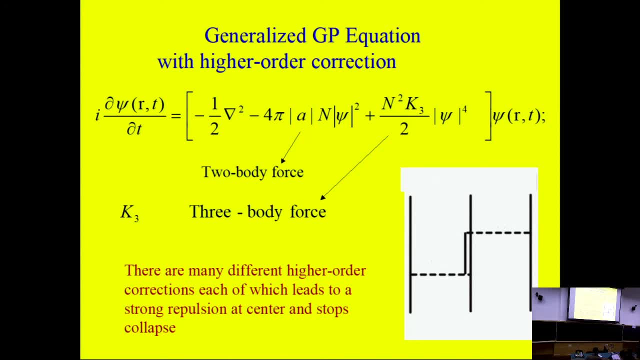 there has been a condensate, then there will be deviation. This equation will not be good because this term will be too big. It's not anymore in the weakly interacting region, Like liquid helium four, which I showed. everything will break down because of very 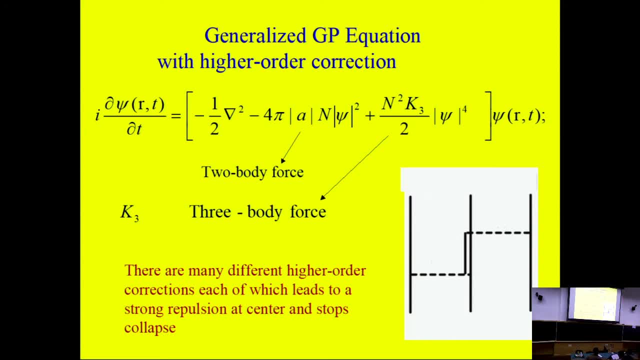 very strong interaction, very dense system. You cannot make a theory. There is no theory for liquid helium. There is another question: Yes, Are there any applications of Bose-Einstein condensation? I don't know. People ask when Caterly, who got no prize? 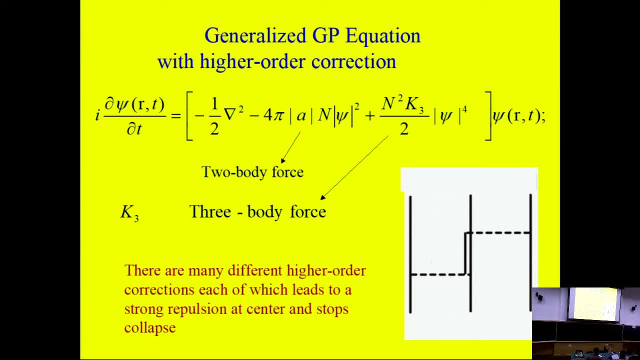 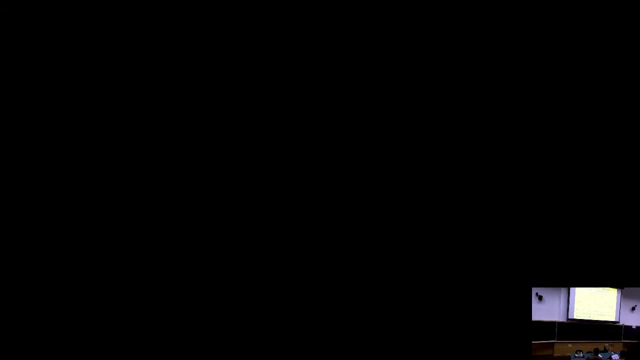 Yes, There is application in quantum computer entangled state. This is a laboratory testing ground of quantum mechanics. But real, real application like this laser is showing this thing Still not known. That's what Caterly replied. But it is very strong, good application in quantum computing, quantum information science. 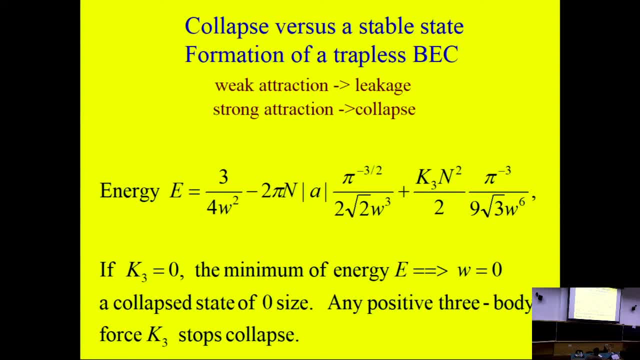 Because these are coherent states And you can study or test your theory Or things like that. Okay, So let's thank Caterly again. There should be some refreshments, I hope. Okay, Thanks. I think Eduardo's question is that you considered the interaction of three bodies. 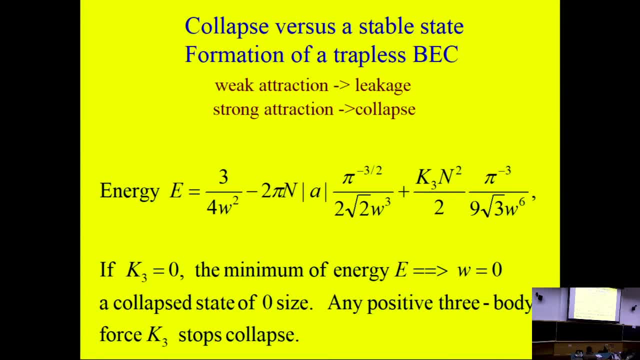 Yes, And his question is: why not of four bodies? No, no, no. Four bodies will be important, They will be very important. They will be very important. Yes, Yes, Yes, Yes, Yes, Yes, Yes. 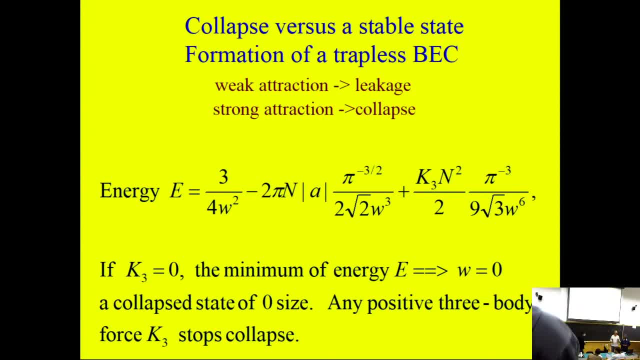 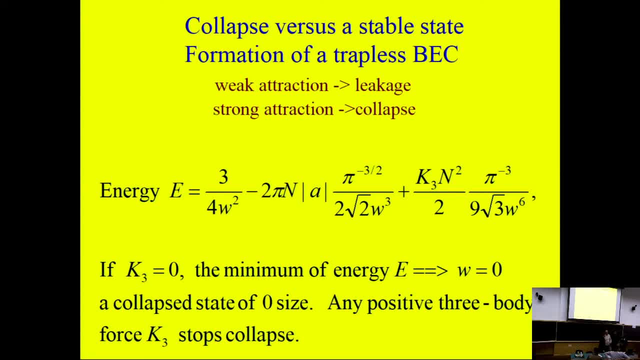 Obviously, Then you need to increase the density even further. What is the expansion parameter here? Series, What's the expansion parameter? and that's the question. And the first question is: are there any application of quantum southwest? What is the expansion parameter?